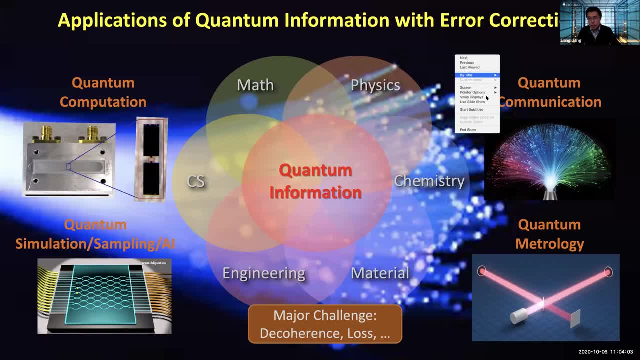 ranging from like a quantum computing communication- sorry, I just need to remove another screen and the error correction for communication. quantum metrology simulation And one of the major challenge for the quantum information processing, if you want to go to a larger scale, is the decoherence. 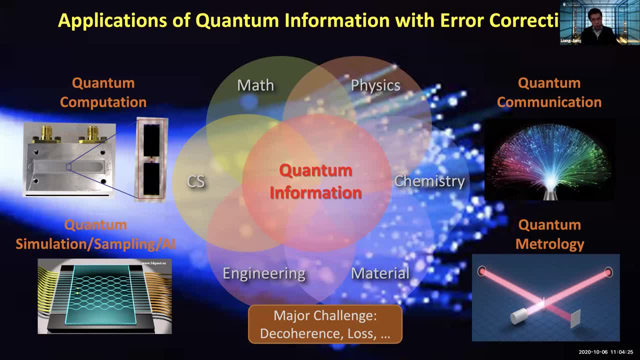 And, for example, your qubit will be depolarized And if you have excitations, it may be lost to the environment and the system may be heated up by the thermal noise. So one question is that okay, well, will error correction be useful for these applications? 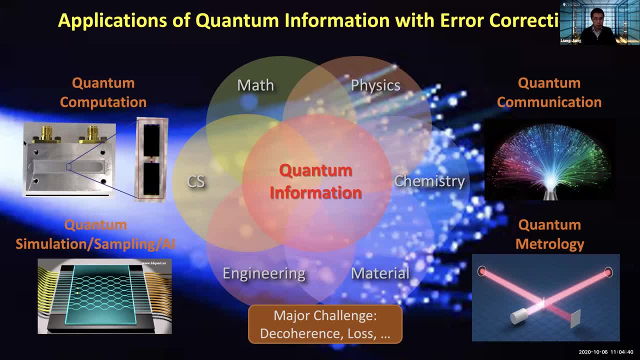 And then we- I guess we probably heard many talks about okay error correction could be useful for computing, or you sound like, for tolerant quantum computing ideas, And also error correction could also be useful for communication if we do some encoding or do some active error detection. 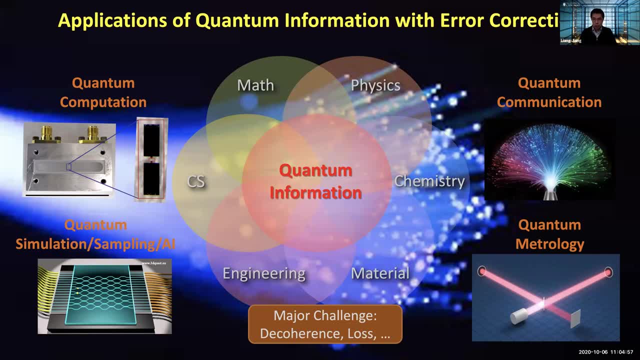 And so today's talk I'm going to be mostly focusing on the other two applications, namely the quantum metrology, if error correction could be useful for that, And also, like a quantum simulation, if we could also use error correction to simulate some system while suppressing noise. 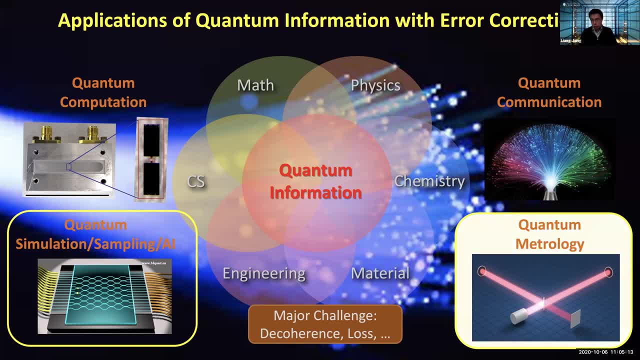 So let me maybe start with the first part on this quantum metrology, And so one of the- actually the idea kind of like- emerges around the well, first the people. I've studied how to use error correction for quantum metrology for more than two decades. 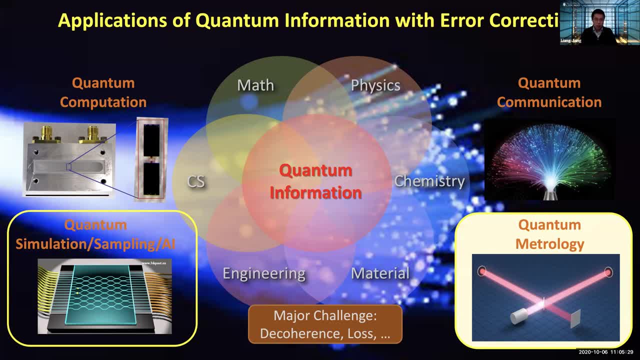 But it was kind of like a bit still vague that it's still well. maybe one of the key questions is: is it easy, Is it easier or harder to use error correction for metrology as compared to use error correction for computing? And on one hand we may say, okay, it's probably easier. 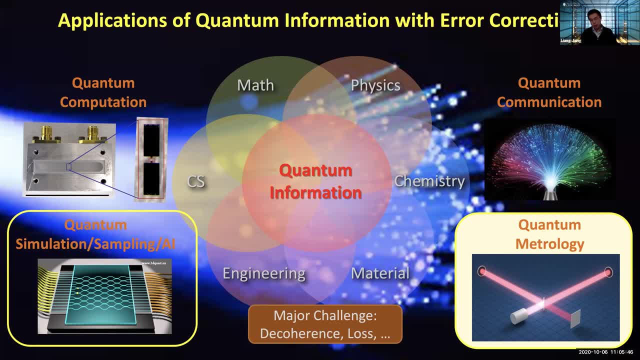 because, okay, we don't need like a extreme, like a precision, and we don't need, we can average many times if we want to do the metrology, While on the other hand, if we say we do computing, we probably maybe need like a large scale. 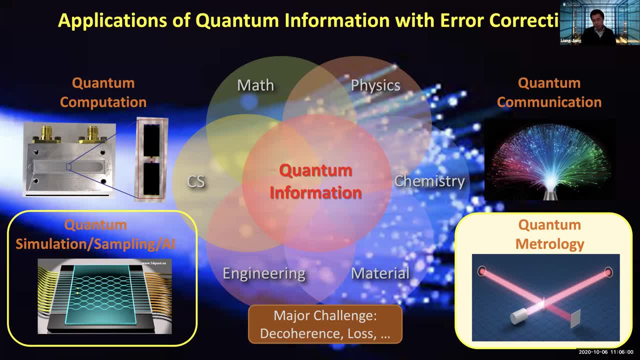 and fault tolerance for computing. But it turns out that actually maybe there's some bit more interesting things. We that distinguishes error correction for computing and the metrology, And I will talk a little bit about it. And so kind of the what motivates me to think. 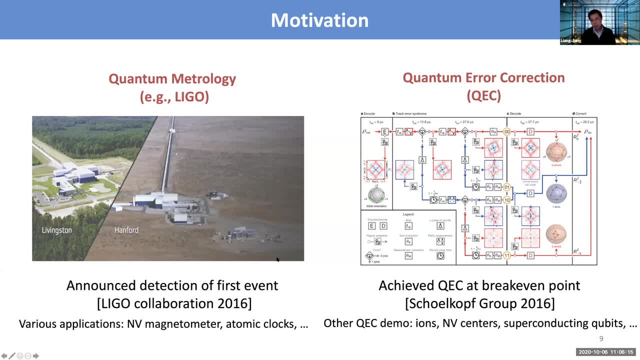 about quantum metrology with error correction was a kind of a two events happened in 2016. And one of the events is the detection of a first gravitational wave events by LIGO in 2016. And the kind of that. it's kind of like a significant 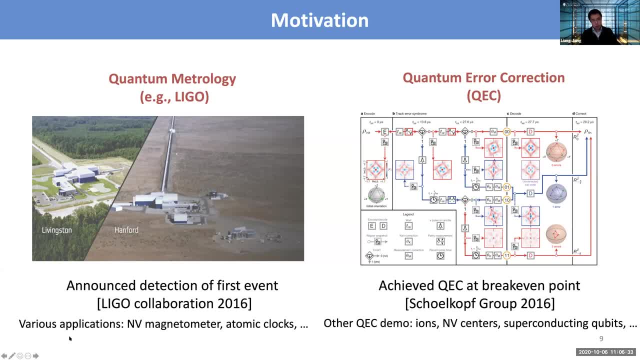 achievement of LIGO metrology, And there are also like various applications, like from larger scale to smaller scale, like MV, magnetometer, atomic clocks, And, on the other hand, in 2016,, there's also like a, like a breakthrough in quantum error correction. 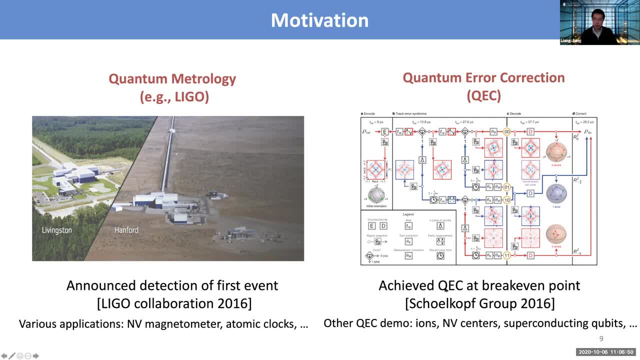 which is like in Rav Shoukhov's group, that they achieved the quantum error correction at the breakeven using CAD codes And also at the same time there are also demonstration of error correction using trapped ions or MB centers or supernatant qubits. 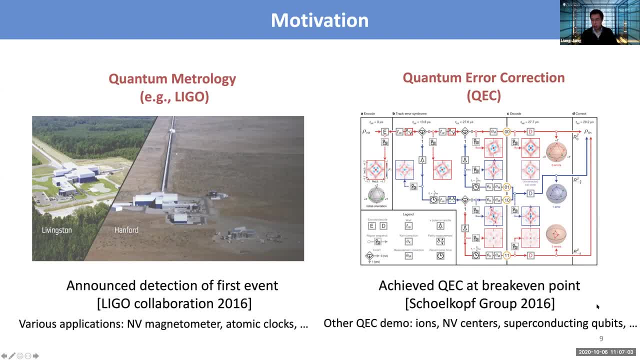 which probably mostly focusing on the error detection. So that's one of the things that we're trying to do, And then the other thing that we're trying to do is to try to find out what is the most common error correction that we can find around that time. 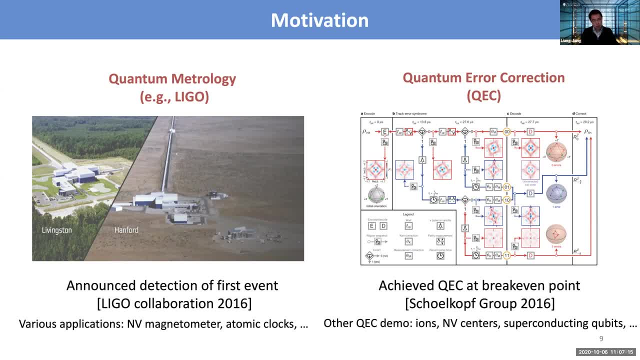 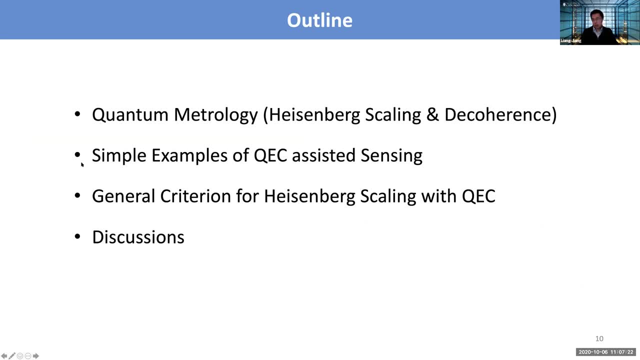 So one question that naturally emerges is that can we actually use error correction to help quantum metrology And to understand, to maybe like to? first we will try to like formulate the kind of the general formulation of quantum metrology And probably go through some simple examples. 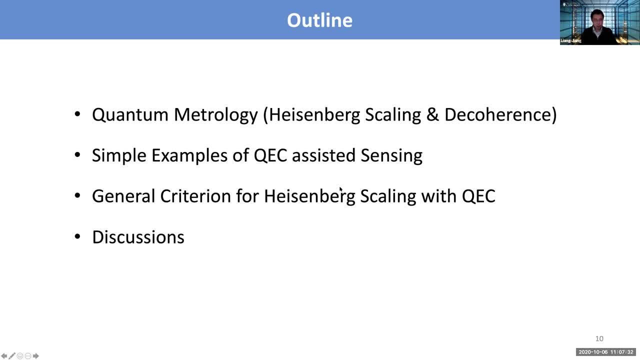 to see that error correction sometimes can be useful to get to the most from the quantum advantage, And then I'll try to develop a general criterion that under what situation that it's possible to use error correction to achieve Heisenberg scaling even in the presence of decoherence. 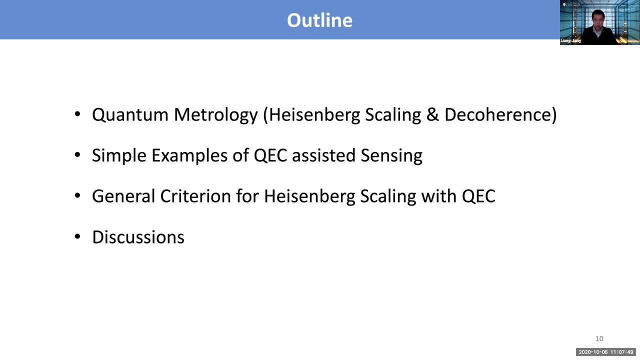 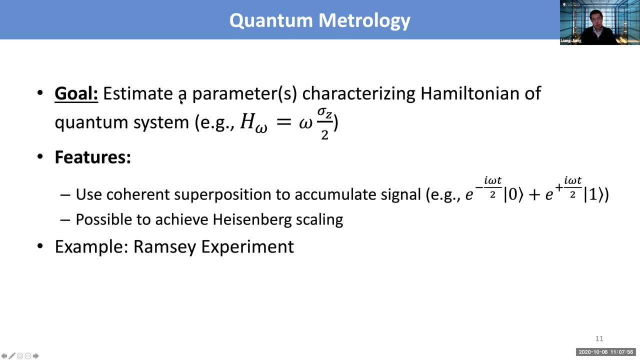 Okay, and then can explore like a different further extension. So maybe one of the goal for quantum metrology is actually to estimate a parameter, or multiple parameters, that is characterized by the Hamiltonian of a quantum system, And here I'm focusing on a particular and bit. 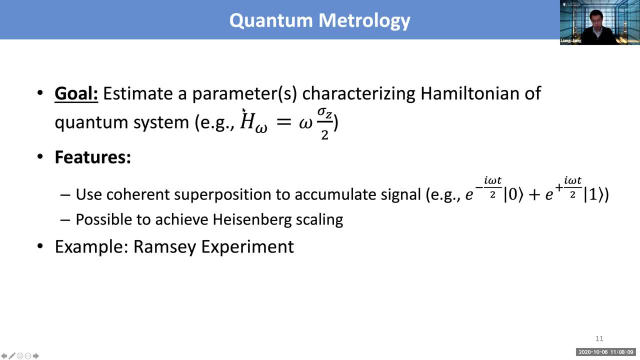 maybe for a specific case is the Hamiltonian. doesn't depend on time, Because that's the case. we can kind of have well defined, like Heisenberg scaling And but there'll also be other interesting cases. But here we're just focusing on parameter estimation. 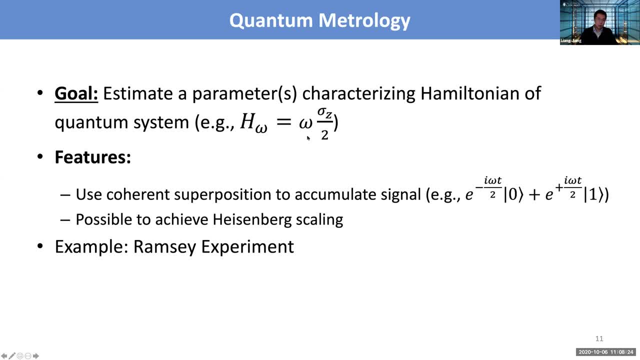 of a time, independent Hamiltonian, For example, the energy difference between two levels, And the feature for this, like quantum metrology, is that the key idea is to use a coherent, coherent superposition of. if it's two level, you can do a zero, one superposition. 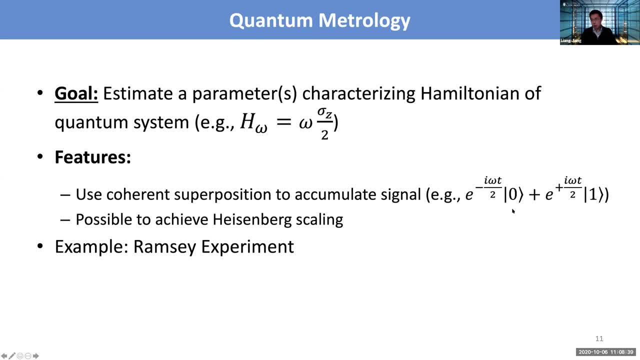 and then let it evolve under the Hamiltonian And then to accuse, accumulate a relative phase between the zero and one state, And then one can use actually some something called the Ramsey experiment to achieve the Heisenberg scaling. So I think that probably most people know about the Ramsey. 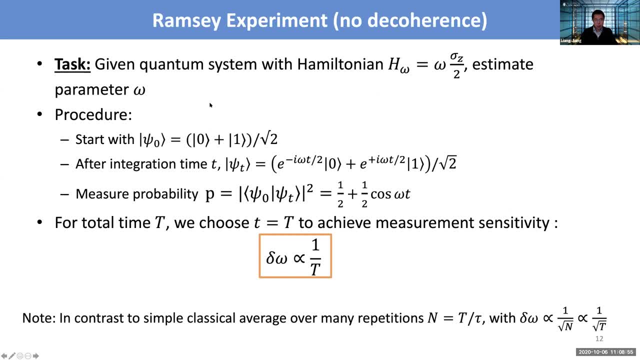 but just to make sure, like we're on same page, just the one slide for Ramsey, which is we have a two level system, starting a symmetric superposition of zero and one state. Let it evolve under the Hamiltonian, which accumulate relative phase between zero and one. 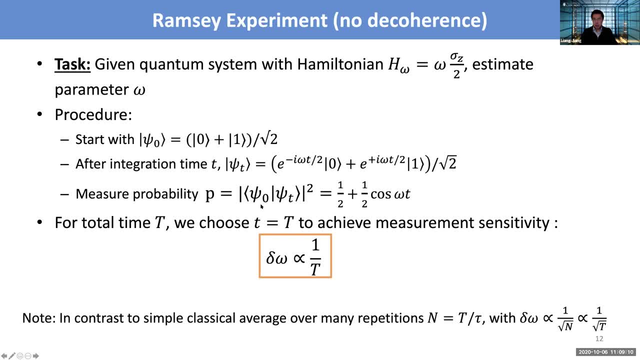 And then you measure what's the probability that the system still stays in the original state And you'll find that actually there's a oscillation that depends on the waiting time and also the energy difference between the two levels And if you have a total time T. 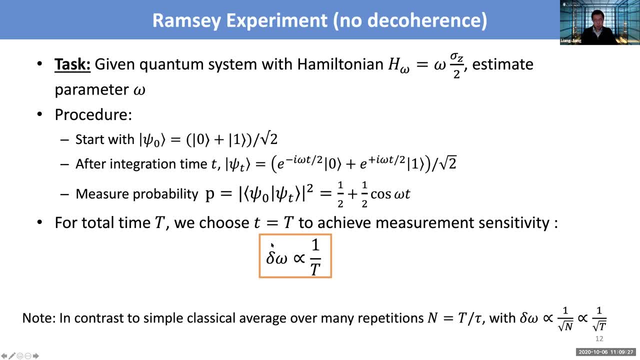 then basically you can choose the measure or you can measure around the time and you will get a time sensitivity, a frequency sensitivity which scales inversely with one over the measurement time T. So that's kind of the measurement sensitivity And notice that it scales inversely. 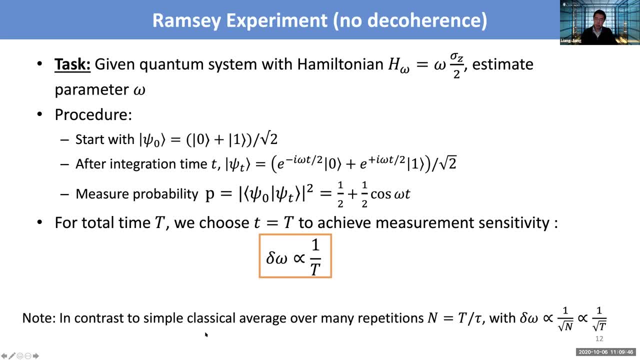 with a total measurement time. And this is in contrast to the classical average, because classically, if we repeat the experiment many times, the number of repetitions scales linearly with n And the uncertainty we get scales as one over square root of the number of repetitions for the classical averaging. 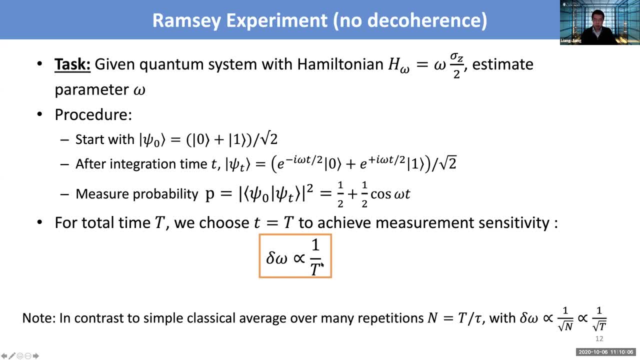 So which scales as one over square root of time T, while in the quantum case actually you get one over T. So this is actually indicating that if you have a pure quantum evolution, we can actually achieve Heisenberg scaling. And here the Heisenberg scaling. 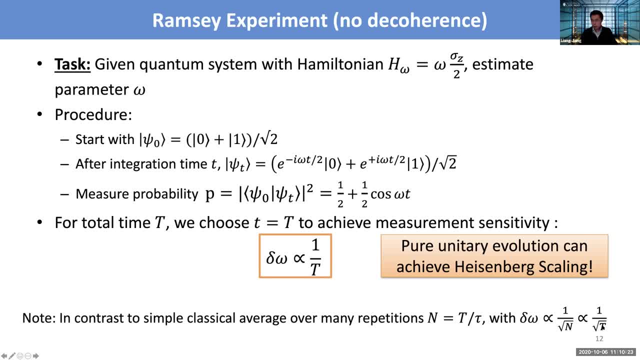 I'm writing in the form of one over T versus one over square root of T for classical scaling And there is a corresponding version. You can say it's one over kind of n, if you consider like multiple sensors doing it at the same time, versus one over square root of n. 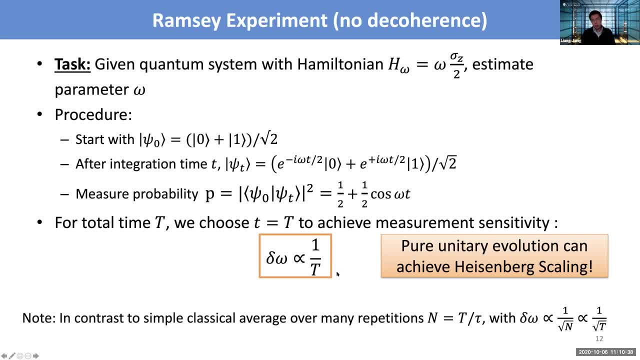 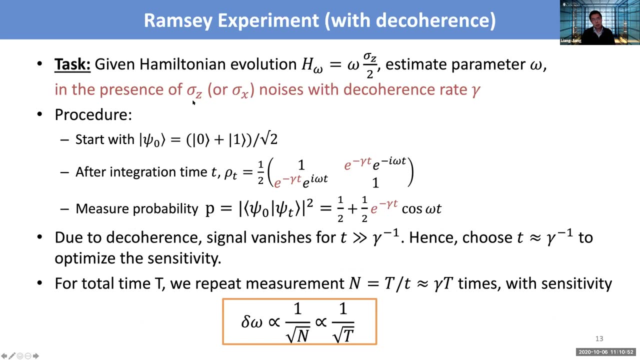 if you consider repeating the experiment n times. So there's sort of like a one-to-one correspondence which works for this time independent Hamiltonian case. So now, ideally we don't have decoherence. That works really nice. In practice, however, the defacing or the spin flips. 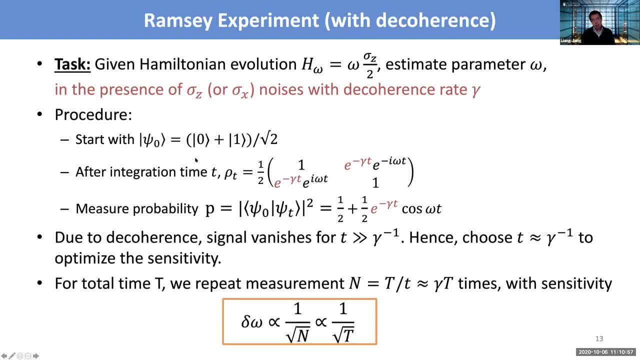 during these evolutions. Now suppose you have defacing, then the state evolution will not be a pure state anymore. So basically, after some like a measurement, interrogation time for T and then the evolution will evolve into a mixed state. So if you have defacing, 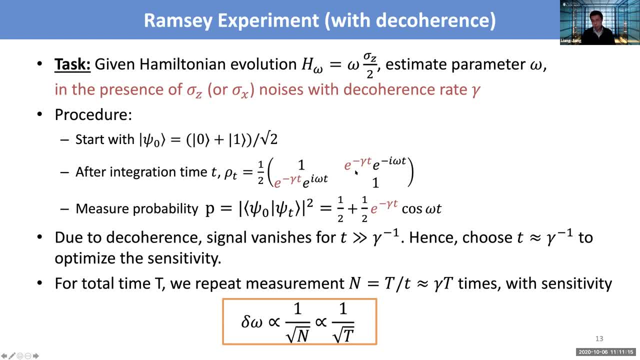 then off-diagonal entries will decay exponentially with this defacing rate And in the end, once you project to measure what's the probability over the initial state, then you will find that actually there is still oscillatory pattern, but the pre-factor for this oscillation 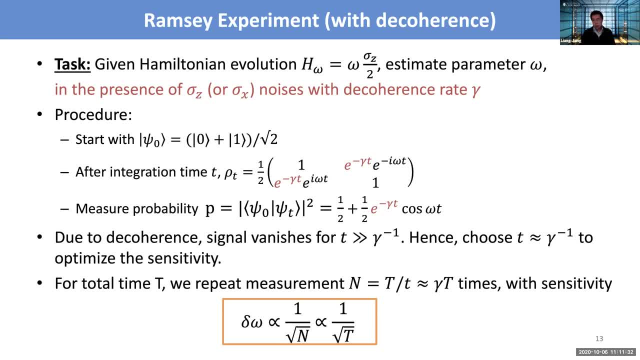 will decrease exponentially with time, Which means that it's probably not a good idea to wait for a time much longer than one over gamma, And so actually one of the optimum point is to choose the time to be of order- one over gamma- so that you optimize the sensitivity. 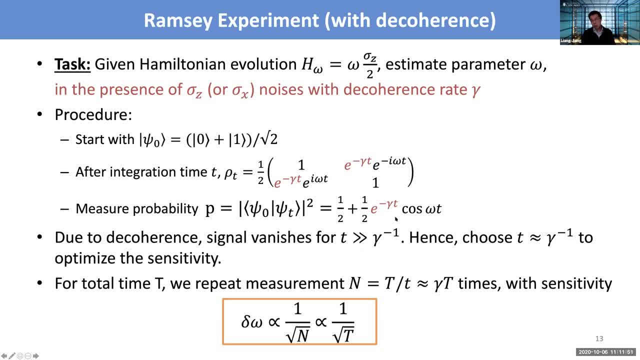 So basically, before the amplitude decays away, probably you should start doing the measurement And then basically you have to restart the measurement and repeat the measurement like n times which n scales as the capital T over T, And then it goes back to the classical averaging. 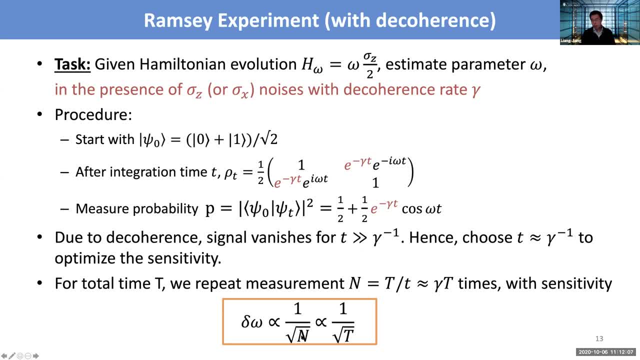 So the sensitivity you get gets back to the one over square root of n, which scale as one over square root of T for the total time. So this again, that's usually that decoherence prevents us from achieving Heisenberg scaling. Yes. 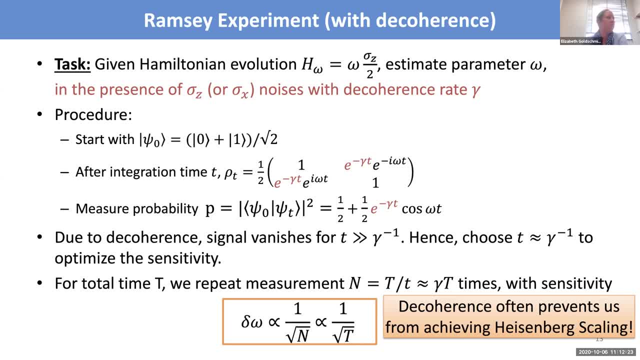 Paul had a quick question that I think is relevant here. So he asked: on your last slide, doesn't the quantum case still scale as one over square root of n, and that you only get one over n if you have entangled quantum systems? 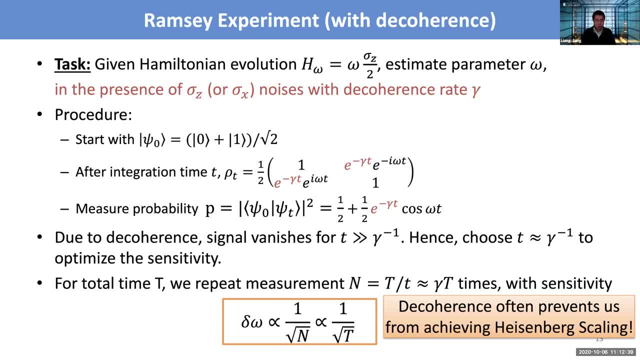 Yes, that's a great question. Yeah, thanks for asking. And first, in the quantum case, if there's no decoherence, I will probably prepare a GHD state. Then that will enable to achieve one over n scaling, And so actually later I will talk about that. 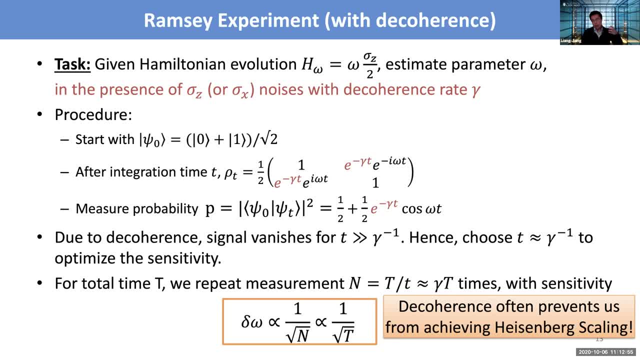 If you have multiple sensors one can actually simulate such evolution with just a single probe, with the price at that. But if you have multiple sensors you will have n times longer for the interrogation time. So that's sort of the you can trade off. 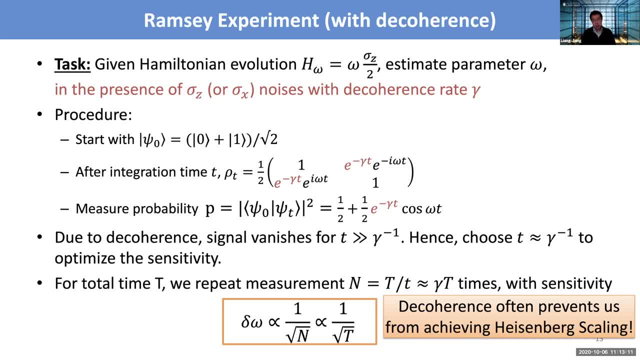 And basically what matters is n times T. That scaling it will be either one over n times T or one over square root of n times T, And I hope that clarifies the question. But here just for simplicity, that's. 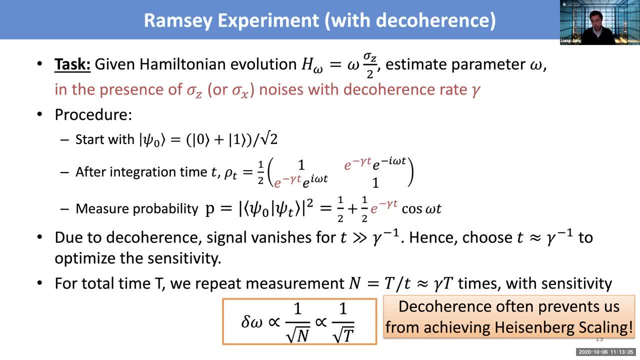 just focusing on the time, which here we show the difference that if there's decoherence, actually we might not be able to achieve the Heisenberg scale. So one question is actually: is it still possible to restore Heisenberg scaling? 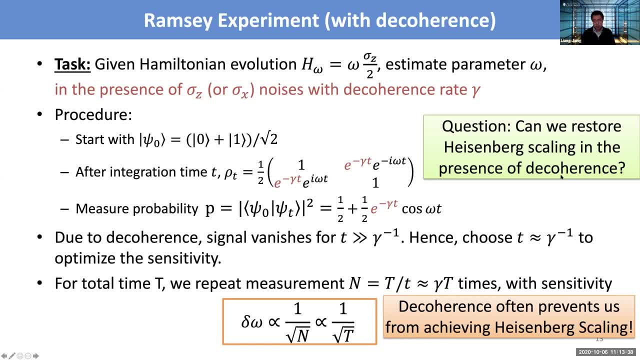 in the presence of decoherence. And well, I ask the question because there are some cases that actually it's possible to restore. But before we get to those cases, maybe let's first give a more clear definition about: well, what do I mean by decoherence? 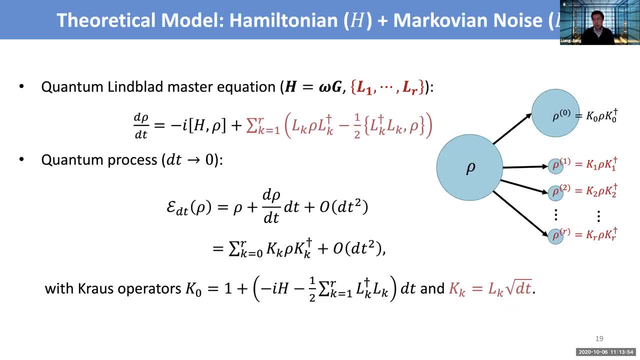 And so here actually I'm considering the most kind of the most detrimental decoherence, which is the Markovian noise And which here the model, theoretical model is considered, that quantum Lindblad mass equation with a Hamiltonian evolution and some quantum decoherence. 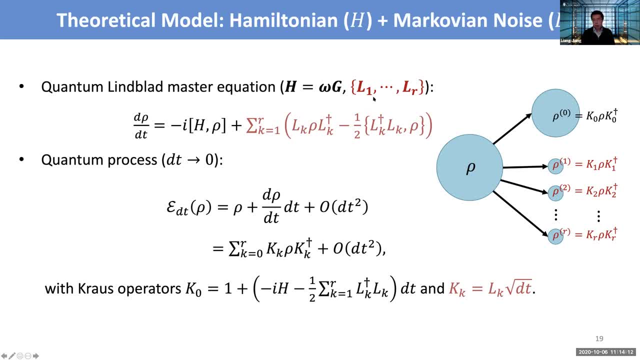 processes characterized by these jump operators, L1 to Lr. And so if it's a short evolution dt, then I can expand this dynamic equation and with the time or extend to the order dt, And you'll find that actually the evolution will mostly be. 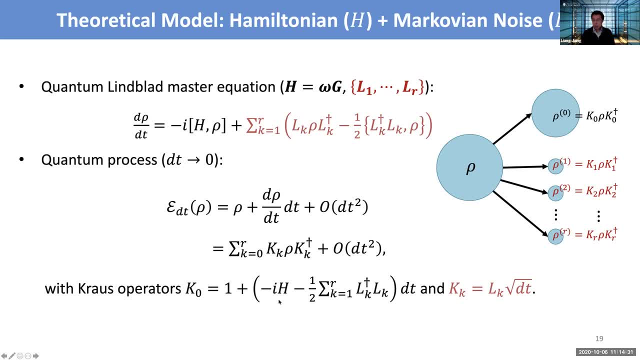 like just a: The identity, combined with some Hamiltonian evolution, combined with some like back action due to the decoherence, that kind of will be the dominant term. So when you take the dt goes to 0, it's just the identity, right? 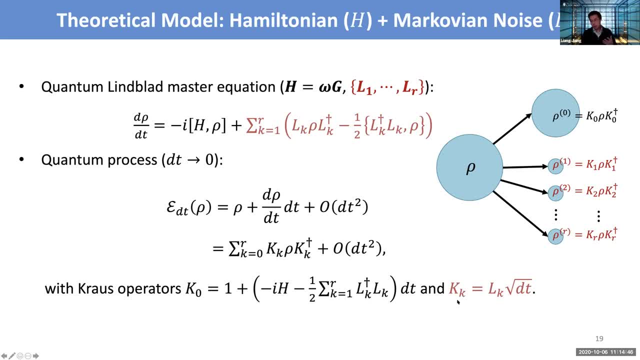 And then the decoherence actually induces some like the quantum jump processes characterized by these cross operators, which is proportional to the Lindbladian and square root of dt, to make sure the dimension is square, OK, So you can think that there is kind of a branching out. 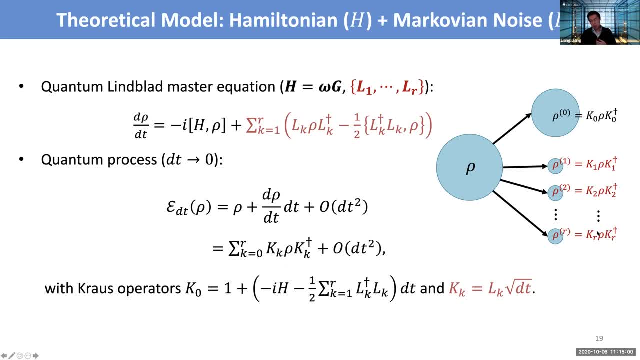 that there is some desired evolution and there is some like undesired quantum jump due to these decoherence processes. So this is kind of the noise model I'm considering And I want to point out this is the Markovian noise, which 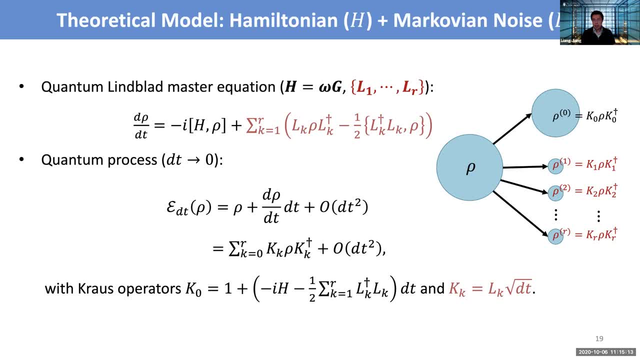 is different from the kind of. like the other noise models, It's time independent. Maybe we can use spin echo to remove the noise, But here we cannot use those tricks to overcome that, So we sort of have to use quantum error correction. 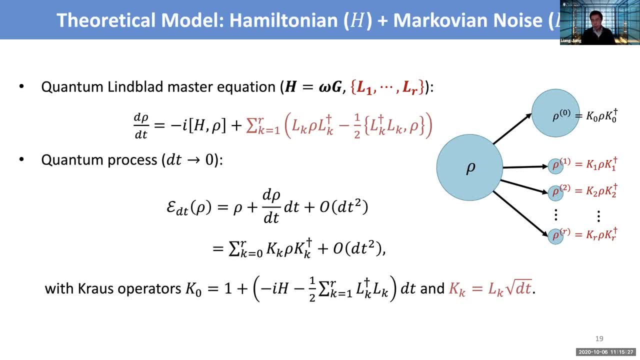 if it's applicable to suppress those noise. And now let's actually, Let's actually consider: OK, what do I mean by? how do we consider the metrology? And here we should, in order to understand how error correction could help, we actually 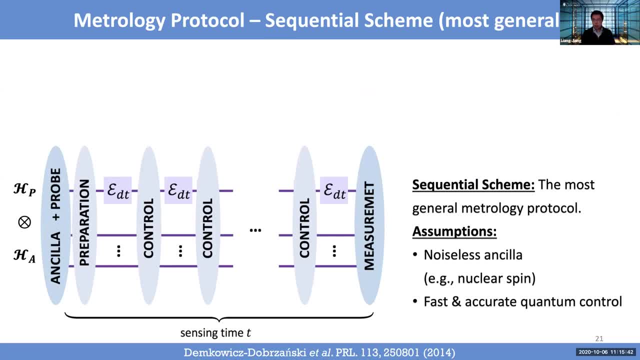 want to consider the most general metrological protocol, And here most general means that here I'm presenting a protocol which it actually can simulate, or possible, or other protocol. So here let me just first describe the protocol and then I will draw the connection to other protocol. 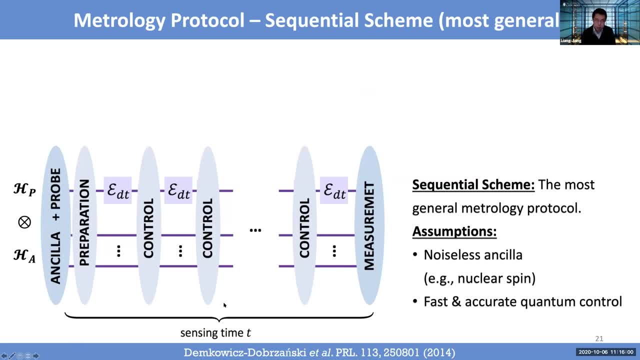 So the protocol is called a sequential. So the model is the following: It consists of the probe, which will couple to the Hamiltonian, which will evolve under the Hamiltonian, And there is also an ancilla, which is some additional ideal system. 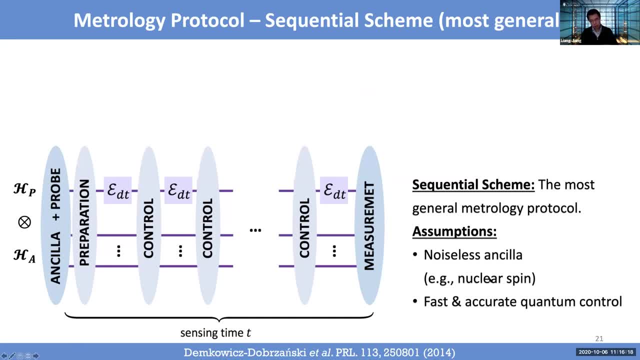 Here I assume noiseless ancilla for example, if you have really long which can play the role of ancilla, And I have a combined probe-ancilla system, I first prepare some entangled superposition state between the probe and the ancilla and some encoding. 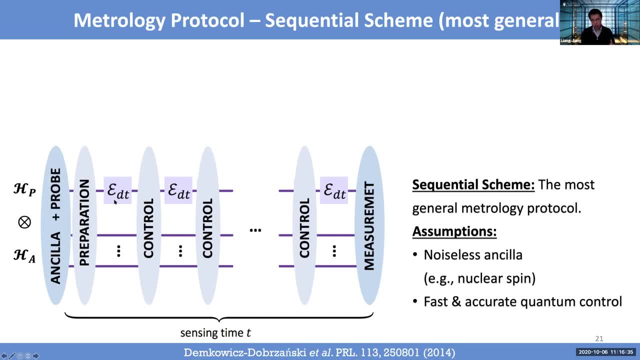 Then I can use my probe to interact with the environment to acquire this parameter that I want to sense. Then I can couple the probe with the ancilla and then alternating this coupling to the environment, a coupling to get the signal and also this control. 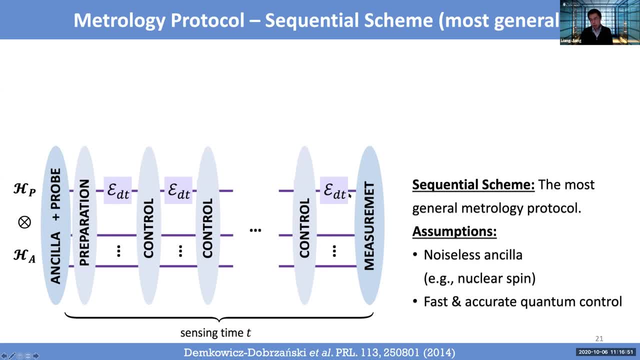 between probe and ancilla, And this is what I mean by the sequential scheme. Notice, there is just a single probe coupled to the kind of try to do the encoding And then I can just do the interrogation And I assume noiseless ancilla. 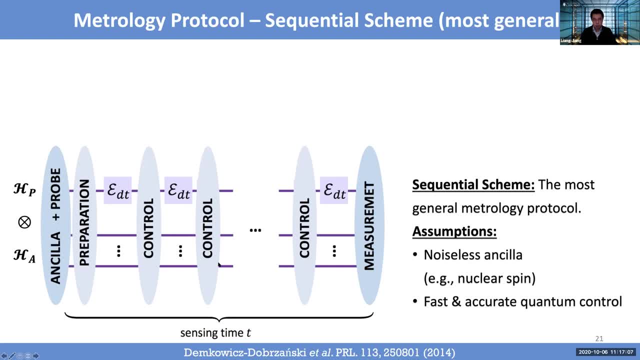 And ideally I also assume there's a fast and accurate quantum control over the ancilla, between the probe and the ancilla And the reason I notice that. I agree that this is a very, very ideal assumption because I assume sort of like a perfect probe-ancilla coupling. 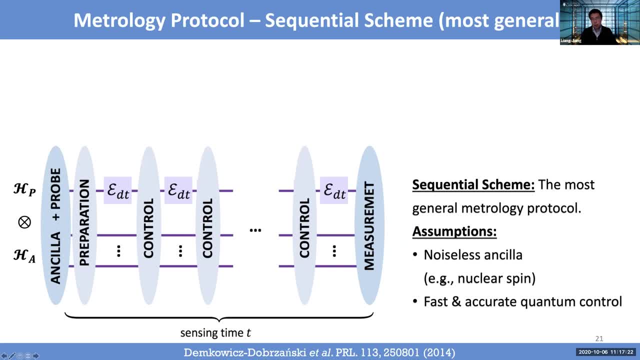 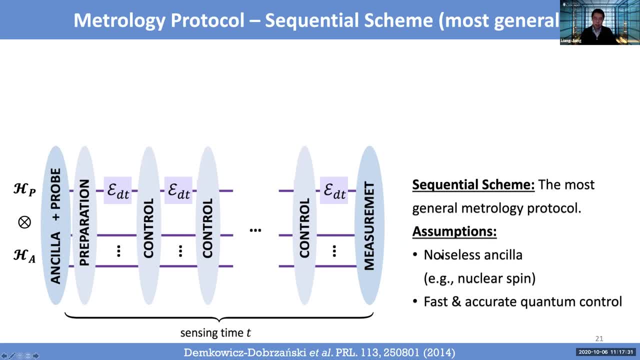 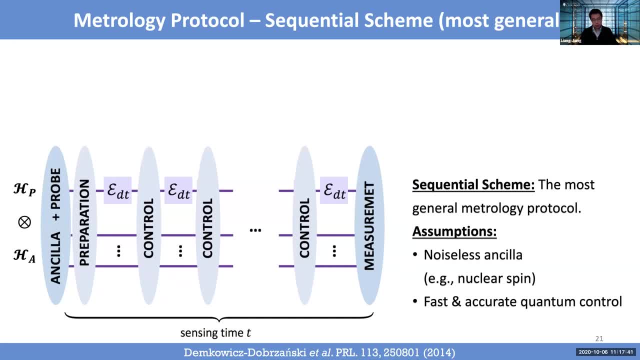 and ultra-fast control, just to see what's a fundamental thing one can do with error correction. And the one question kind of related to one scheme. people might think: oh what if I have n probes? And actually that scheme can be effectively simulated. 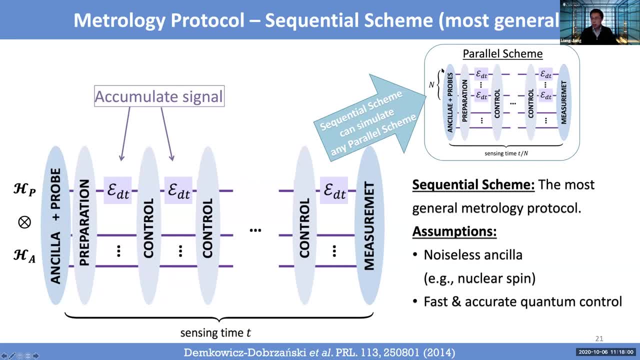 by using our. So suppose you have n probes, you can use n probes to simultaneously to interrogate and to get the signal. OK. However, the simultaneous interrogation can be reduced to our single probe acquisition if we can extend our sensing time by a factor of n. 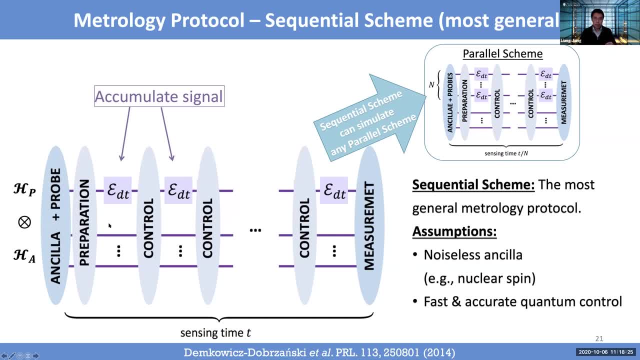 And therefore we can essentially swap between our probe and ancilla to effectively simulate that there is n probes which are simultaneously doing the sensing. So that scheme is called a parallel scheme, which can be actually reduced to our sequential scheme, because a sequential scheme just adds: 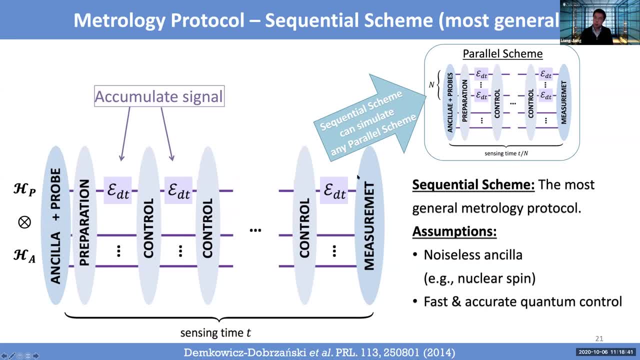 the price of extending the time by a factor of n. It can perfectly simulate this parallel scheme. So that's why we call this sequential scheme is actually the most general one, which actually sort of captures all possible schemes that you may have. OK. 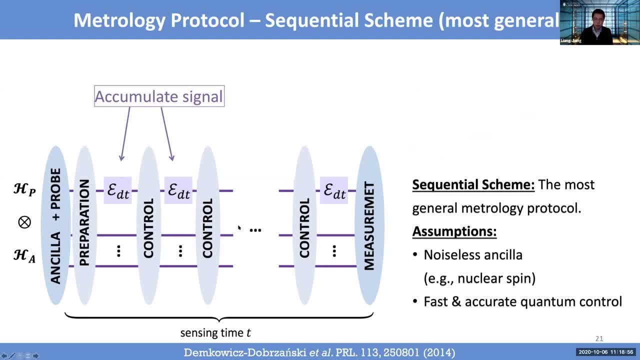 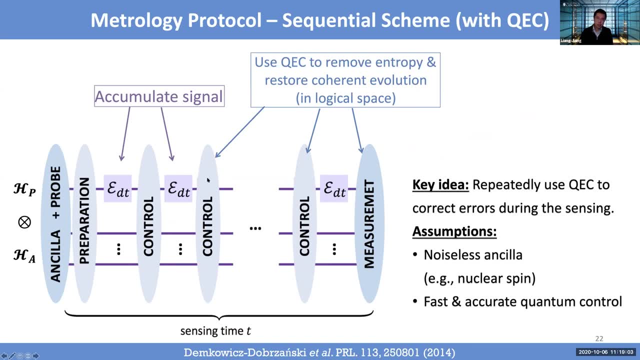 And here we actually want to be a bit more focused on kind of how to do these controls And we'll consider just using quantum error correction to perform quantum error correction, doing these controls, And the goal is to remove the entropy from the noise and try to restore the coherence. 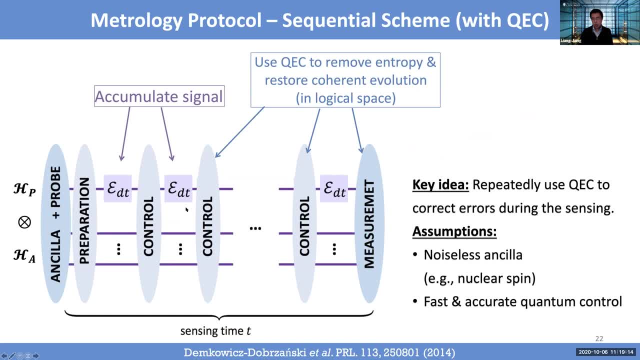 So that's a probe that is combined with some ancilla. There will be some logical space and there will be a coherent unitary evolution in that subspace. And if we could have some effective, coherent unitary evolution in the logical space, then we 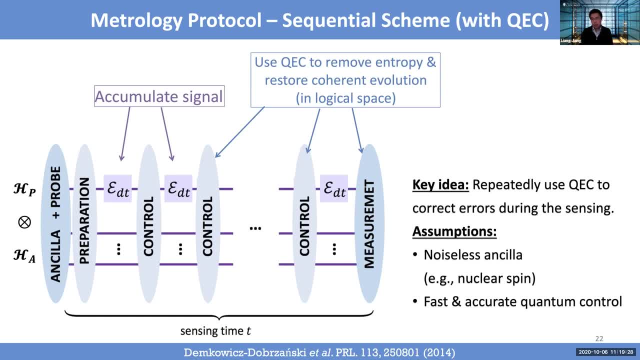 might have some chance to restore Heisenberg scaling, Because in that logical space the system still behaves as a quantum system. So this is a bit abstract. so maybe let's look at some examples. So the first example is actually a qubit probe. 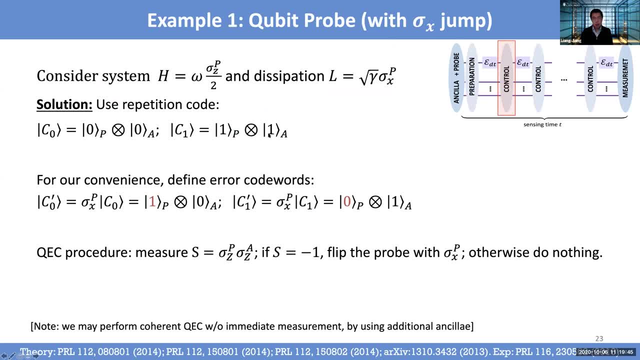 with a spin flip along the x-direction jumps. So basically, Hamiltonian is the poly-z, Hamiltonian with frequency omega and the dissipation is poly-x. OK, It's only poly-x, It's not like a random rotation around different axes. 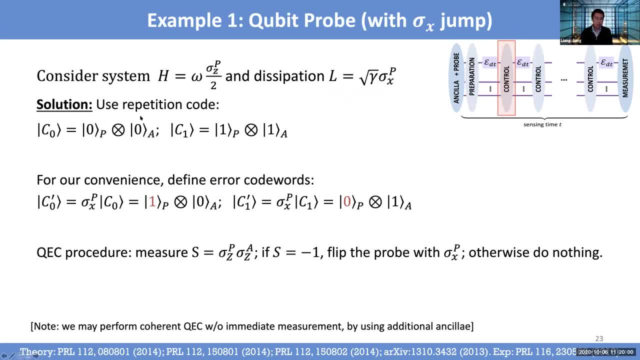 It's only a random rotation around the x-axis. And here's the scheme. You can use a repetition code. Basically, the probe is 0. You also attach ancilla being 0. And if the probe is 1, you attach the ancilla to be 1.. 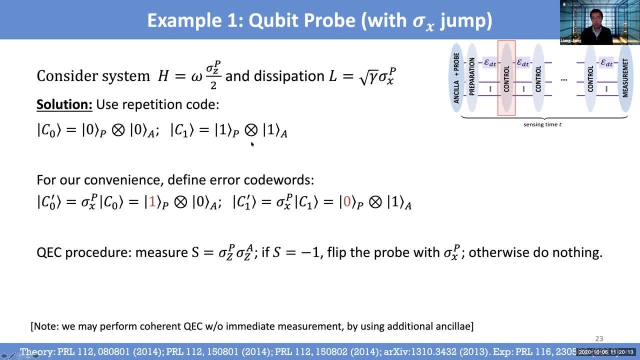 So it's like a simple repetition code which span a two-dimensional subspace over a four-dimensional space associated with a qubit and answer. And if there is a bit flip in our probe, then what happened is that 0, 1 will. 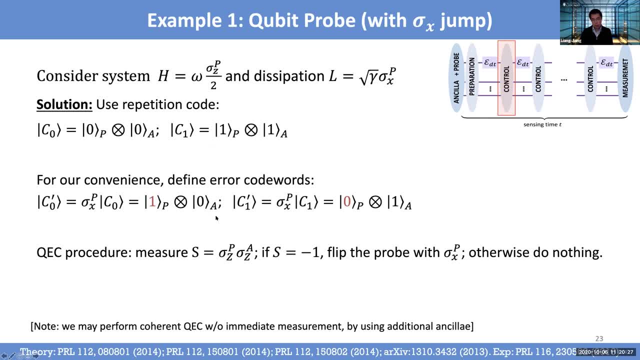 be flipped to 1, 0 for the probe and answer And the 1, 1 will become 0, 1 for probe and answer. So therefore you notice that if there's a bit flip, it goes to orthogonal subspace, with respect. 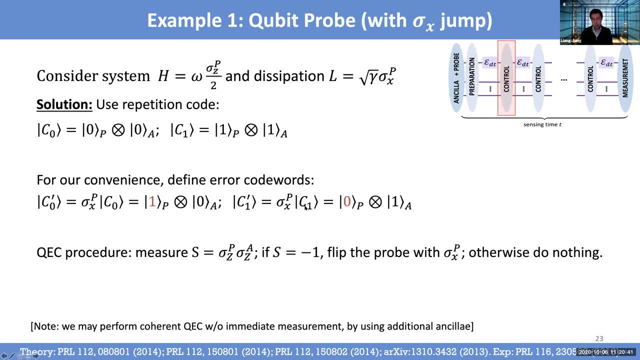 to our logical space So we can ambiguously detect. there is a bit flip because there is a simple procedure: You just measure the product of the polys of the probe and ancilla And you will know whether it's plus 1 or minus 1.. 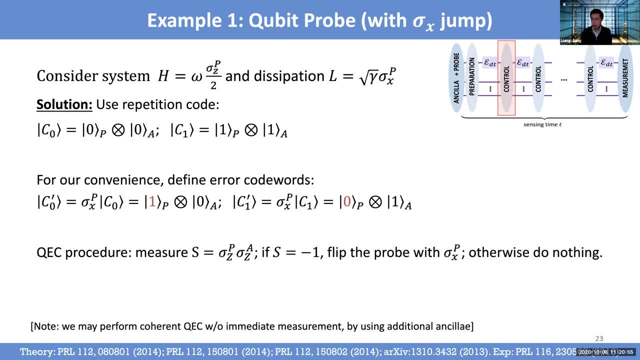 That tells you whether or not there's a bit flip happen while you're doing the interrogation. OK, So if the bit flip happened, then you can undo the bit flip by applying X rotation on the probe, And if there is no bit flip error. 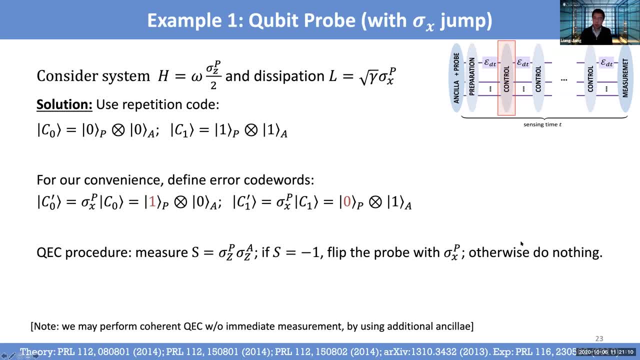 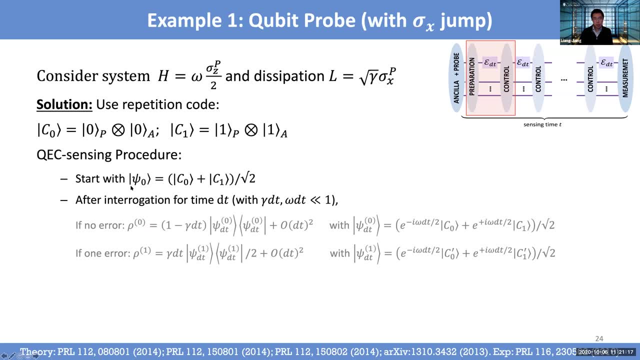 then you don't do anything, You just let it keep continuing during the acquisition. OK, So now let's look at the procedure. So, basically, we start with a state that's encoded in the logical space associated with the C0 and C1.. 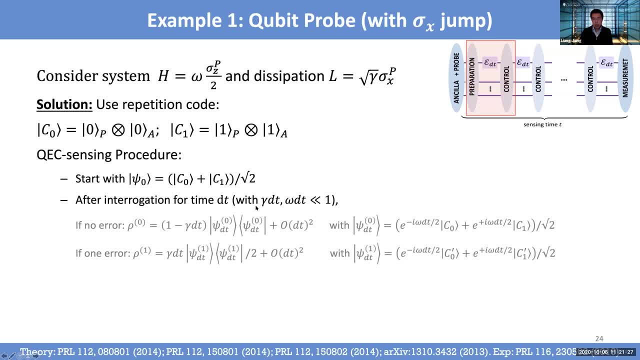 So after some interrogation, for a small time dt let's assume OK, the decoherence during that time, gamma dt is actually much less than 1.. OK, So in that case basically there are two possibilities, If there's no bit flip error. basically the system. 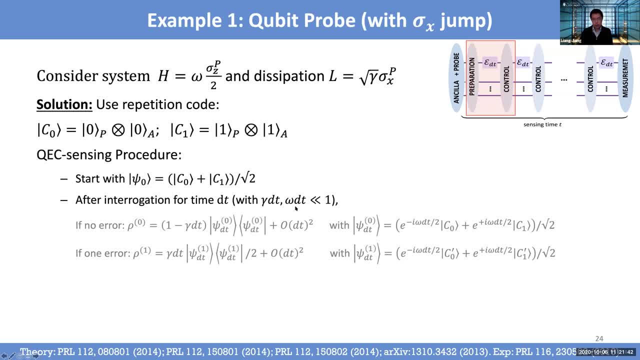 evolved as it should be with this desired Hamiltonian And there's a little bit of reduction of probability, because there's a finite probability, there is no error And if there's error happened, then the system evolved actually in this error space with C0, prime and C1. 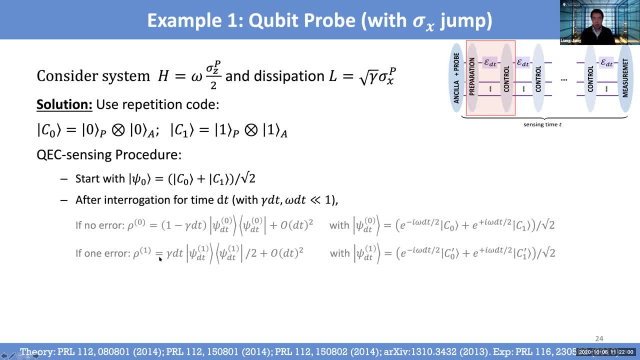 prime. So this is a bit flip error which is a bit flip error, which is a bit flip error, but it has a probability, which is gamma dt And, as we said earlier, there is a way you can measure the product of the polys. 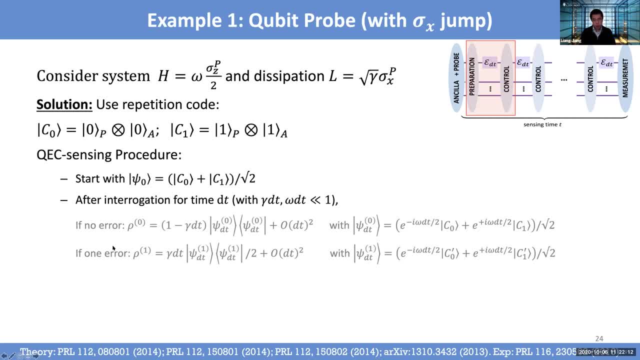 and to distinguish whether or not there's a bit flip. And if there is a bit flip then basically you can flip back the first probe qubit so that it restore back to the logical state. And after you're doing that then basically 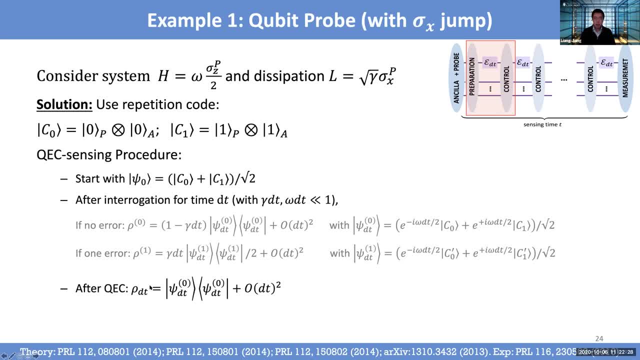 to the leading or to the linear order of dt. you basically have a unitary evolution within the logical space And the error associated with the bit flip and the other contributions is only contributing to the second order of dt. So basically, with this repetition code, 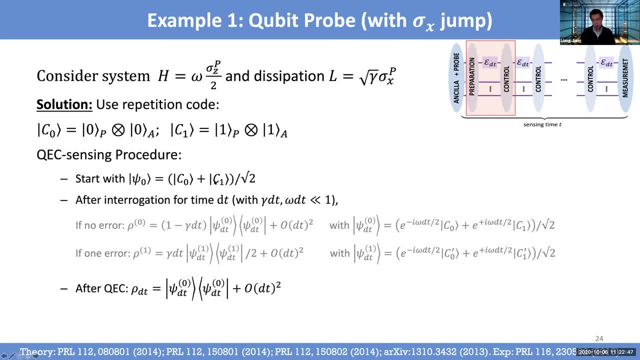 and this detection and correcting of the bit flip errors, we're able to restore coherent unitary evolution within the logical space and accumulating the phase signal we want and suppressing the error to the second order of dt And basically we effectively achieve a unitary evolution. 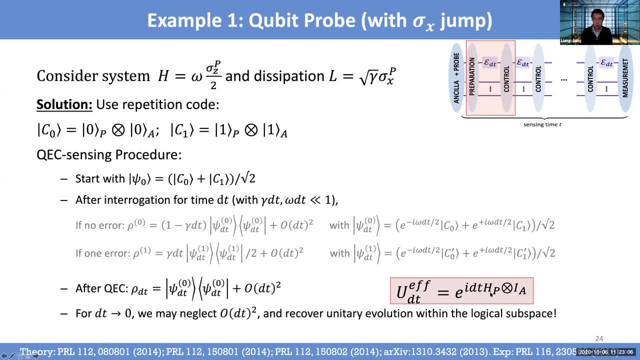 within the logical space that with the Hamiltonian kind of edge probe tends to identity of the answer. And if we take the limit that dt go to 0, then basically we can neglect there is any contribution from the dt square and we recover the effect of unitary evolution within the logical space. 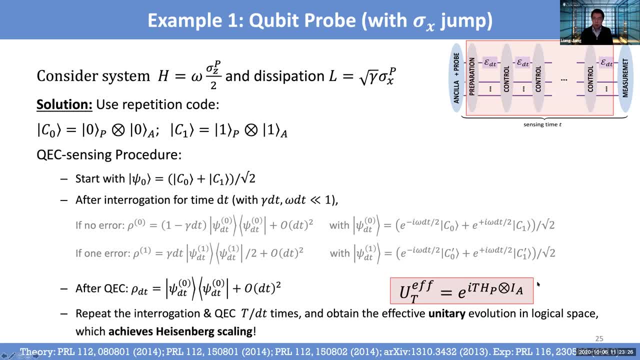 And if we repeat this procedure many times, then we will in fact actively obtain a unitary evolution within the logical space. And, as we mentioned earlier, essentially we're doing a Ramsey experiment in the logical space that will achieve the Heisenberg scaling. 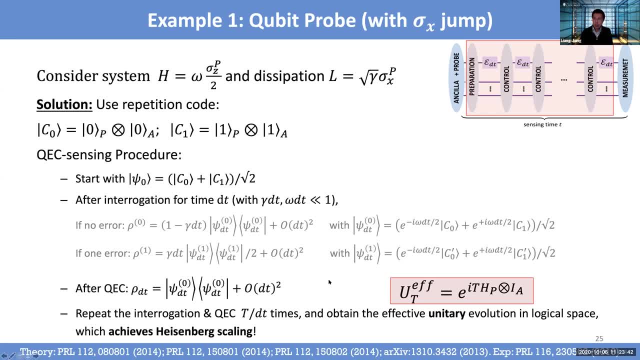 So that's kind of the key idea And I showed in this example that actually for this particular case, when we try to sense the energy sigma z signal in the presence of poly x noise, we can actually achieve Heisenberg scaling, assisted by quantum error correction, with this repetition code. 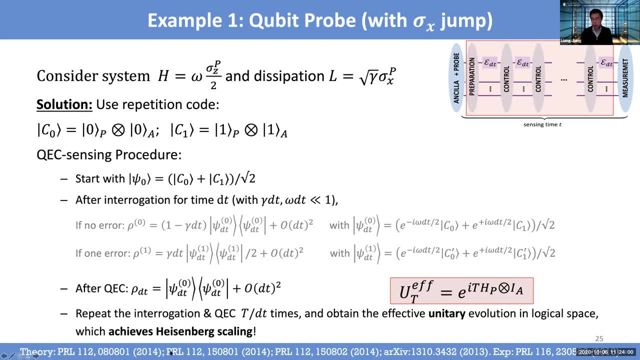 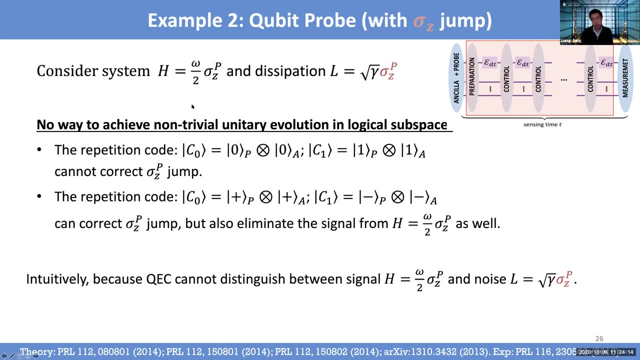 And this is actually proposed earlier around 2014.. And there's even an experiment using MV centers which tried to demonstrate that there is some potential improvement with such a repetition code encoding And, on the other hand, there are also other cases that it may not work. 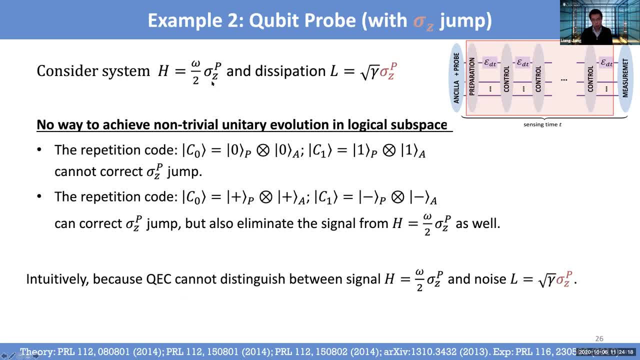 For example, if you want to sense the energy difference between the two levels in the presence of the phasing error, Then in this case actually there is no way to achieve this non-trivial unitary evolution in the logical space Because, for example, if we do the repetition code, 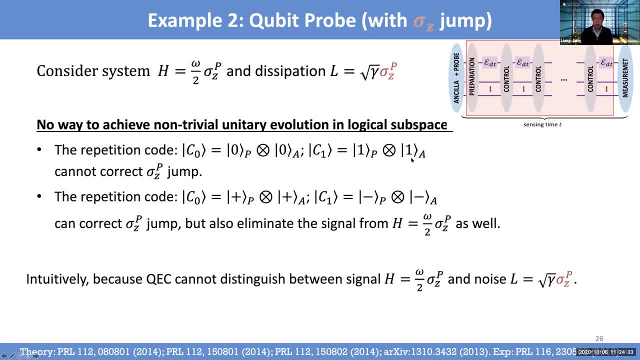 that we did earlier- 0, 0, or 1, 1,- then actually we cannot detect or even correct the phasing error, Because it cannot tell whether the phasing don't change this logical space. On the other hand, if we do the repetition code with a plus, 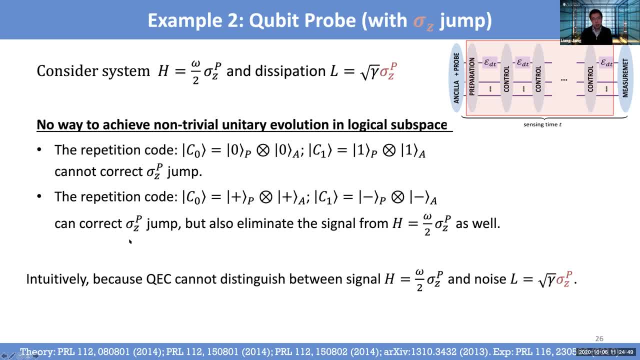 plus and minus minus, then basically it will correct this phasing error, But at the same time it also corrects the signal as well, Because the signal is treated as the phasing. So therefore there is no way that the quantum error 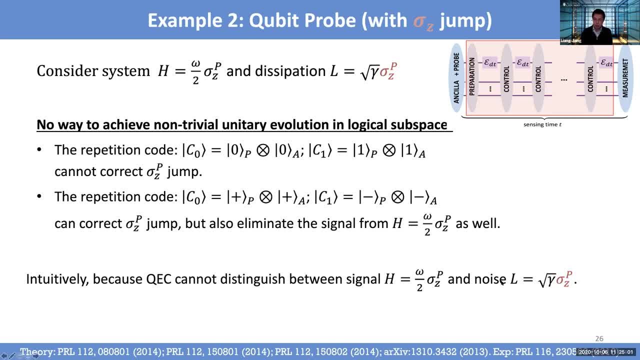 correction can distinguish whether the signal or whether it's a noise, Because essentially, it's the same policy operator applied to it. So then, the natural question is under what condition error correction can help us to restore Heisenberg scaling in the presence of decoherence? 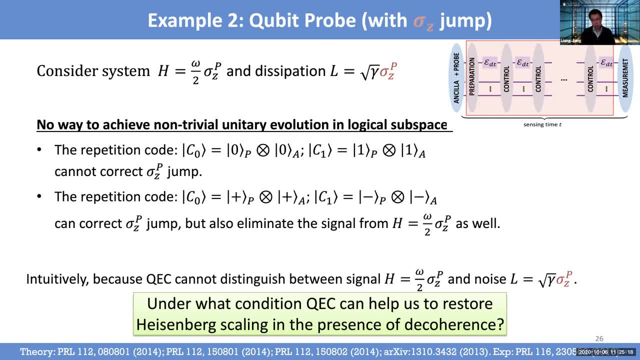 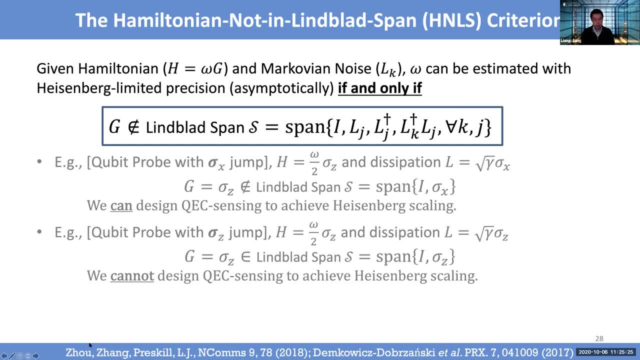 Because obviously, there are cases it may work And there are cases it may not work, And so here is actually the general criterion that's actually obtained by my students. This is around 2017.. And basically, here is a statement of the criterion. 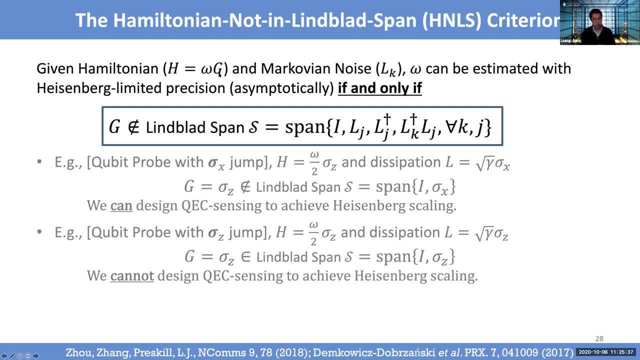 And basically your Hamiltonian will have a Hamiltonian operator And the Markovian noise will also have the jump operator, And we can actually use error correction to restore the Heisenberg scaling if, and only if, this Hamiltonian operator is not. 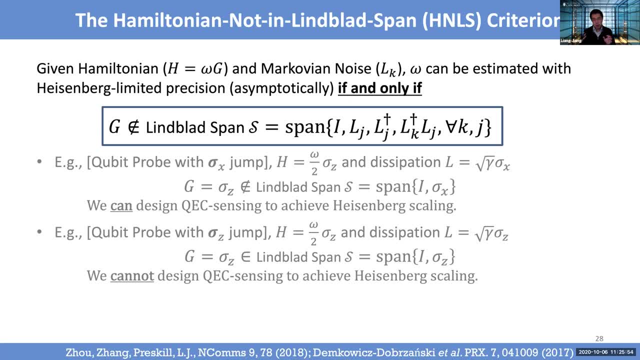 fully contaminated by this Markovian noise- And the way you can interpret the Hamiltonian- and not contaminated by the Markovian noise. there is a rigorous statement- is that the Markovian noise will span an operator space which is called the Lindblad span, which 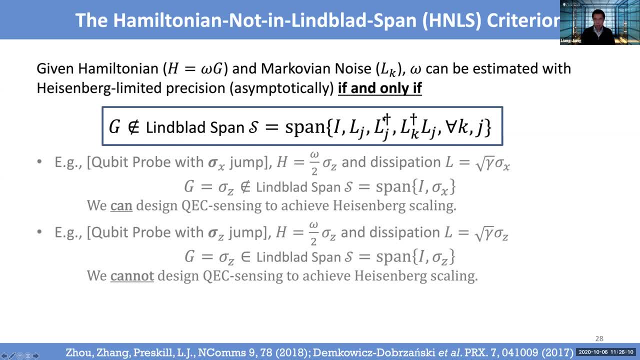 consists of identity linear or Hermitian conjugate of the Markovian noise and their quadratic combination, And those are, you can think, as operator space which are contaminated by the Markovian noise And if, by any chance, your Hamiltonian 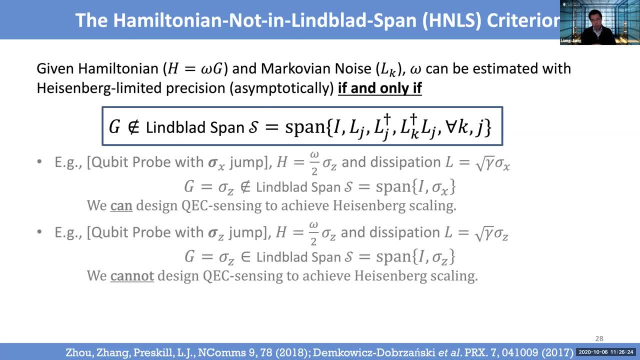 has some component which is not in that operator span, then you will have some And you will have a signal which can be distinguished from the noise. And even that's a tiny bit of a signal, you can still use that signal to sense and for sensing. 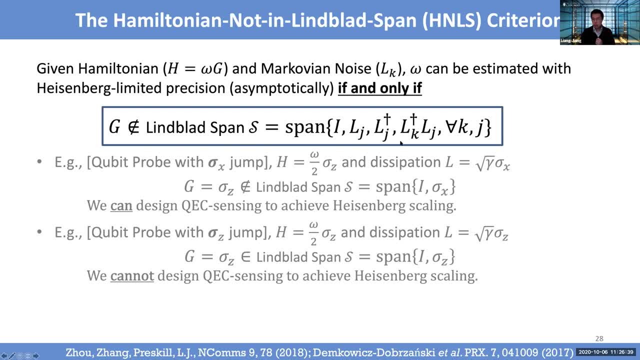 And because of that signal is sufficient, distinguished from the noise, then you can use active, you can use error correction to suppress all the noise and just keep that signal component and induce coherent, unitary evolution within your logical space to achieve Heisenberg scale. 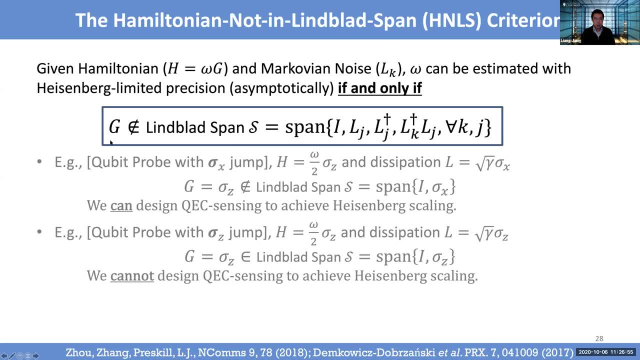 And so this is kind of like the underlying intuition of this Hamiltonian, of this G operator is not in the Lindblad span, which is a necessary and sufficient condition, allow us to achieve Heisenberg scaling with error correction. So now let's look at two examples we had earlier. 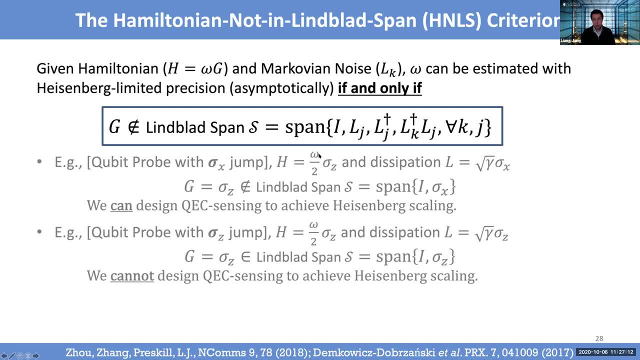 So we mentioned that we want to sense the energy difference of a two-level system. So the Hamiltonian operator is poly sigma z and the dissipation operator is poly x. So the Lindblad span for this case is identity poly x. 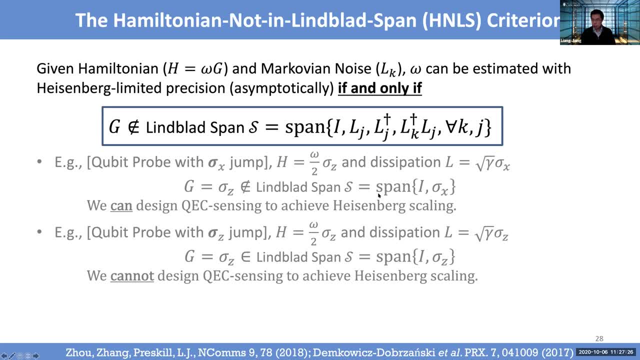 And you may have poly x squared, but poly squared is identity. So basically the Lindblad span is just identity on poly x And in this case actually our Hamiltonian operator, sigma z, is not in the Lindblad span. 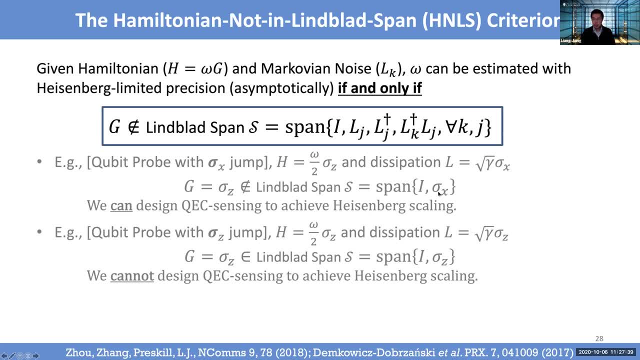 because poly z cannot be written as a linear combination of identity on x. So therefore we satisfy this condition. So there should be a Heisenberg limited version which indeed, as mentioned earlier, we can use repetition code to restore Heisenberg scaling. 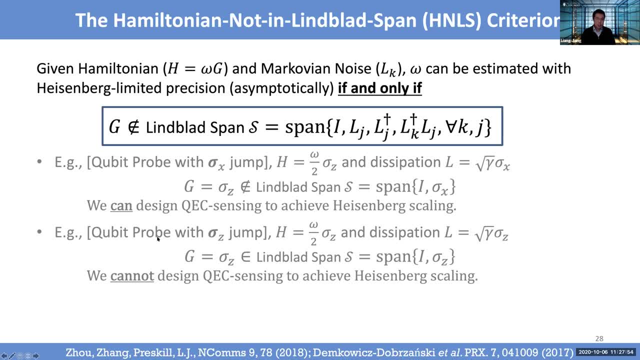 or quantum error corrected sensing. Now the other case, which if we have sigma z noise and we have sigma z Hamiltonian, then in this case, unfortunately, the Hamiltonian is within this Lindblad span because sigma z noise can cover our Hamiltonian. 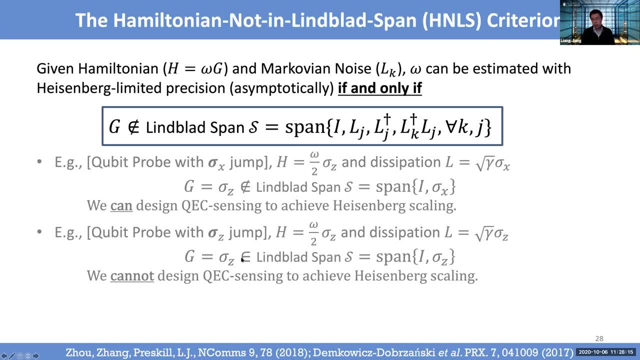 with a sigma z signal. So we cannot design error correction scheme to achieve Heisenberg scale. So maybe, I guess that's maybe for the time sake, in case people are interested, you're welcome to look into the paper, But here just to like a sketch. 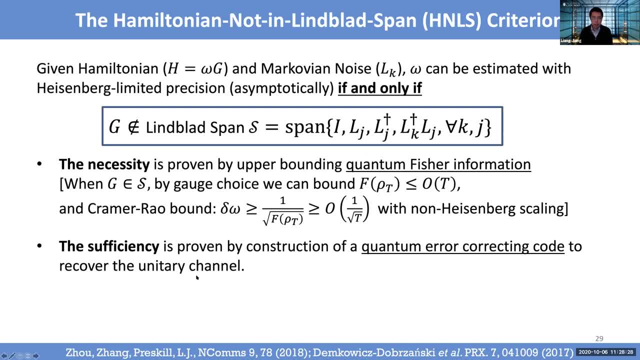 here how we prove this condition. the necessity is actually proven by computing the upper bound of quantum fissure information. So basically, if the Hamiltonian is in the Lindblad span, is in this contaminated subspace, then basically we can choose. 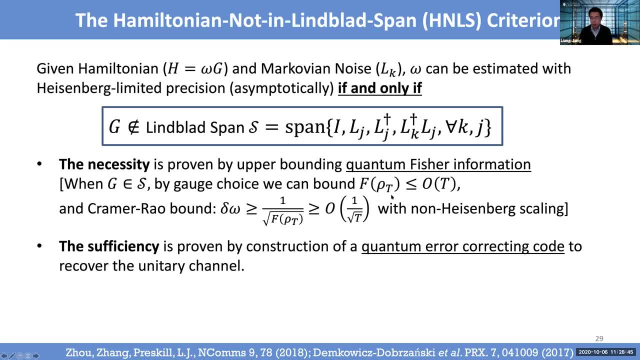 and compute the quantum fissure information which will be upper bounded by something linear with time t, And then we can use something called the Crammerer bound which says uncertainty of the quantity you try to sense will be limited by kind of the inverse. 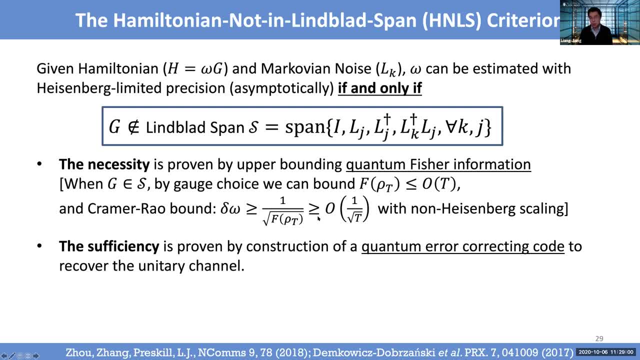 of the square root of the fissure information And that will give you a bound which says the uncertainty will be kind of like a lower bounded by one over square root of t, which is no Heisenberg scale And the sufficient condition is proven. 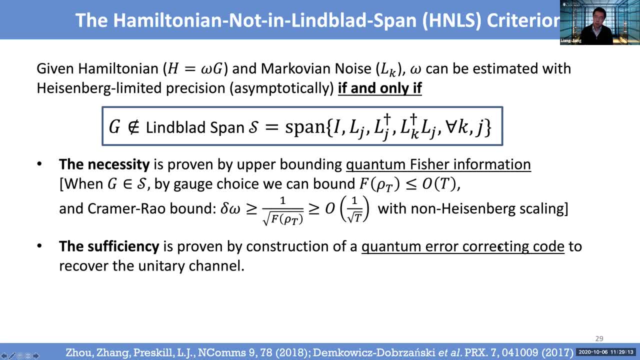 by the construction of quantum error correcting code that can recover this unitary channel. And actually it's explicit construction of the error correcting code that we actually prove the sufficient condition. So, and I guess that maybe let me just go through one slide. 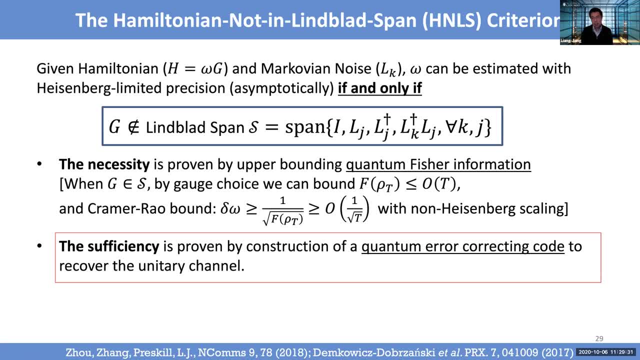 in case people are interested in this technical part, how we actually get the sufficient condition, And it's actually like a not that hard. So the key idea is the following: We want to take advantage of this orthogonal component, the component of the Hamiltonian. 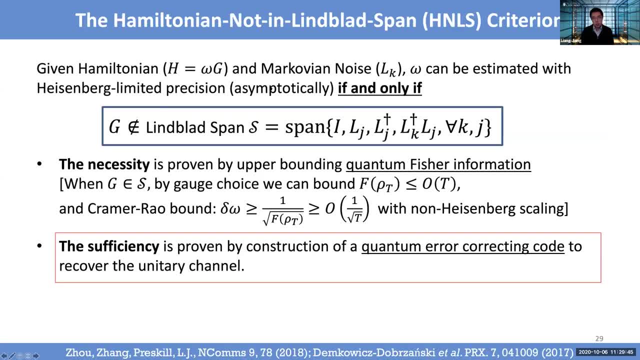 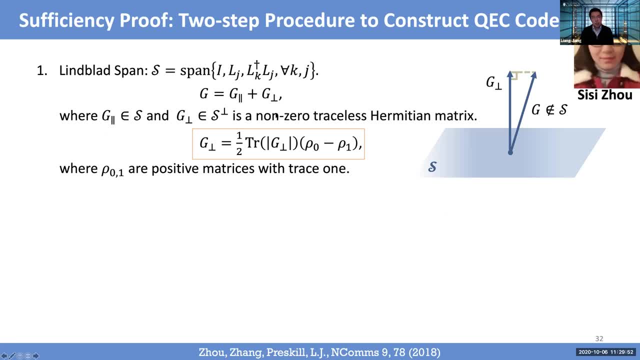 which is orthogonal to the Lindblad span, which we call this G perpendicular. okay, In this orthogonal component of this Lindblad span we can actually use that construct, the error correcting code. So first, the Hamiltonian can always be expanded. 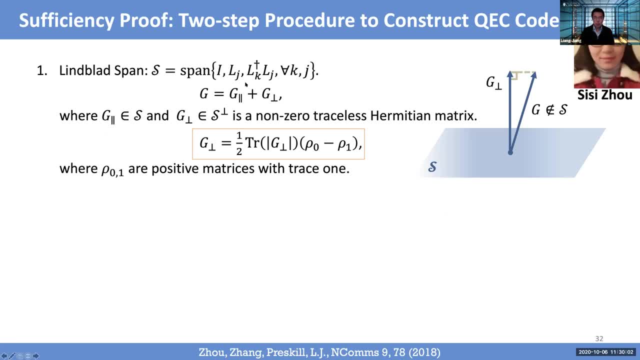 in a linear combination of a component which is contaminated by the Lindblad span and a component which is orthogonal. And because identity is in the Lindblad span, so the orthogonal component must be traced zero, which means that you can write some parts. 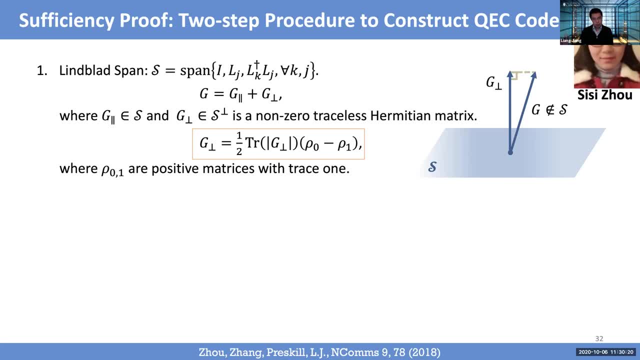 which has positive trace, some parts which has a negative trace, and you can combine those two things to give you this orthogonal component of the Hamiltonian And, if we can call the positive trace, could be called to be row zero with a normalized version. 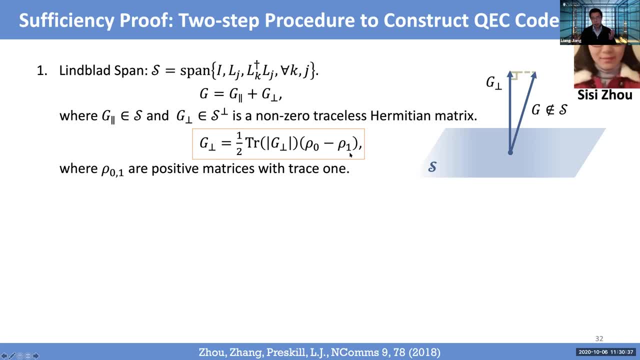 And the negative part of the trace is row one, which you can think. those are two kind of density matrices And those two density matrices actually need to have orthogonal support And they actually corresponds to like two different like states, which has no overlap. 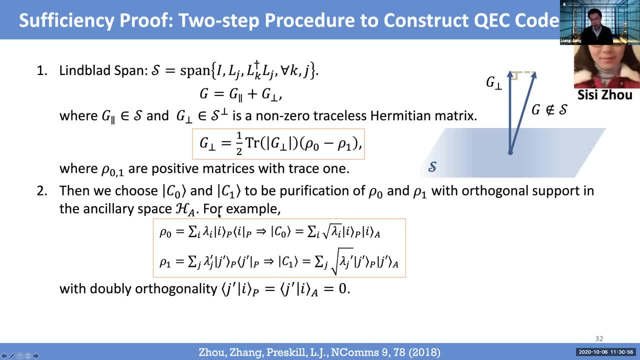 And you can construct or purify those density matrices with additional ancilla And that actually gives you the code word to the encoding information that can be used for error corrected sensing. So one example, as we discussed earlier, if G perpendicular is sigma Z, for noise sigma X. 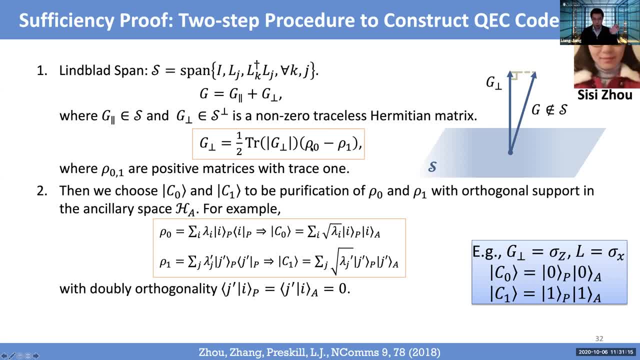 then sigma Z. you can write it as zero, zero, which is row zero, minus one, one, which is row one, And you can purify it with additional ancilla. So basically the code word will be zero, probe zero, ancilla. 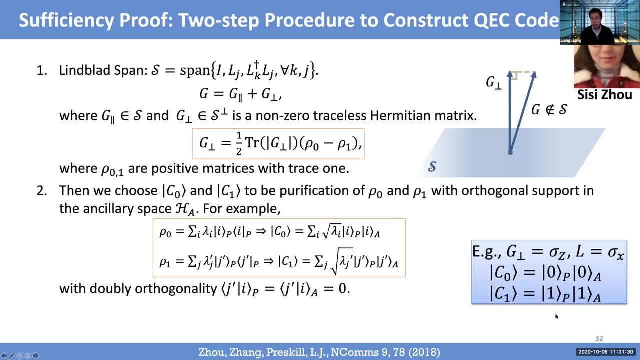 And the other code word will be one probe, one ancilla, And that's exactly the repetition code that we constructed and allow us to achieve Heisenberg scaling, as shown earlier. So, basically, this gives you a generalized recipe which actually invented by Sisu. 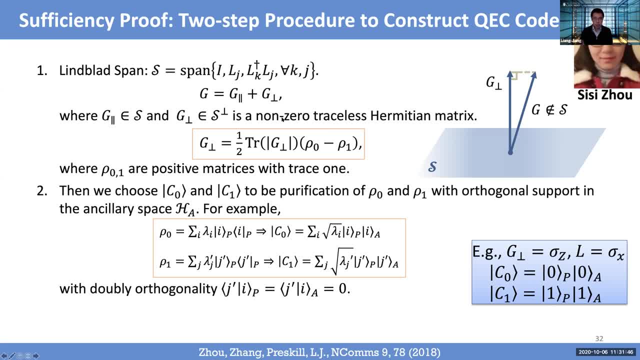 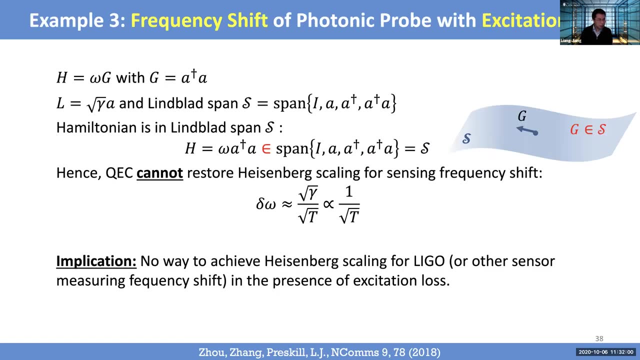 that one can actually achieve explicit constructed error correcting code that allow us to use quantum error correction to restore Heisenberg scaling If the Hamiltonian is not in the Lindblad span. So maybe, just it probably could be more like intuitive to see some more examples. 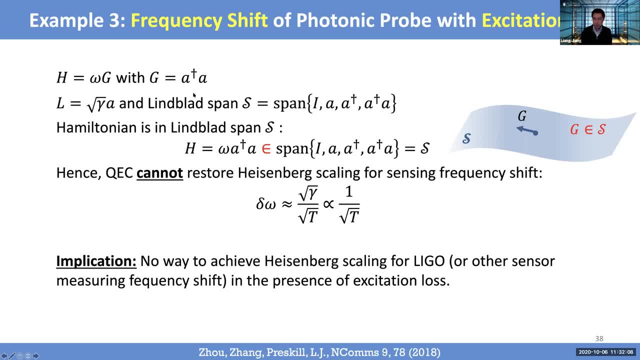 And here's the example which is kind of related to the earlier discussions of LIGO, That I'd say okay. well, we're asking the question like: can we use quantum error correction to help LIGO to restore Heisenberg scaling? 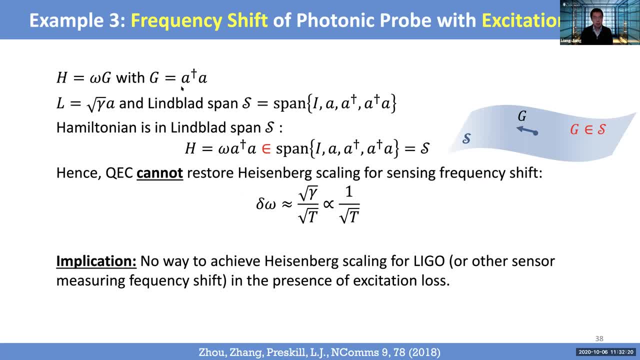 And so here we have the Hamiltonian, which is this: we want to sense the frequency shift of some resonator, Which could be induced by the gravitational wave signal that induce the lens change of the resonator and induce the frequency shift. At the same time the system may have photon loss. 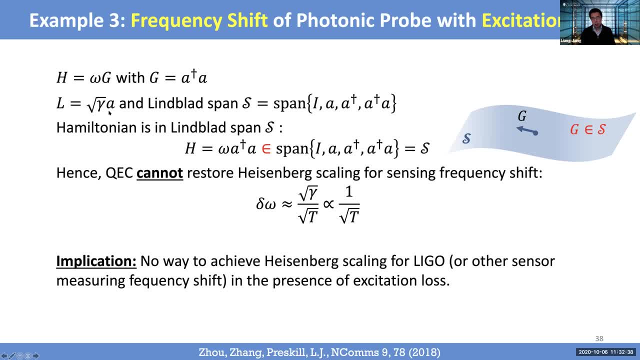 So in this case the loss is characterized by the annihilation operator A. So the Lindblad span, which consists of identity, these loss, linear of these jump operators and the quadratic of those jump operators, it span this operator space And notice that the quadratic part of the span, 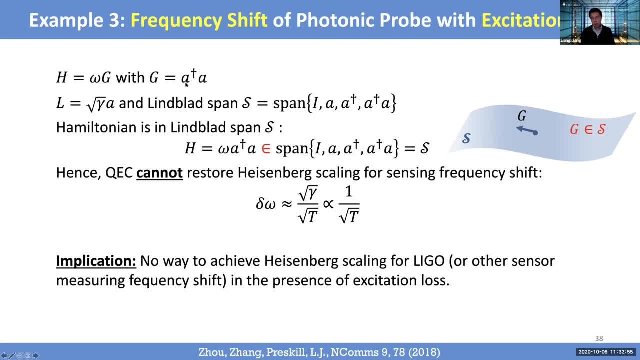 which is A dagger. A is exactly the same as our Hamiltonian. we want to sense. So in this case, unfortunately, the Hamiltonian falls within the Lindblad span, So basically, it's contaminated by the noise due to photon loss. 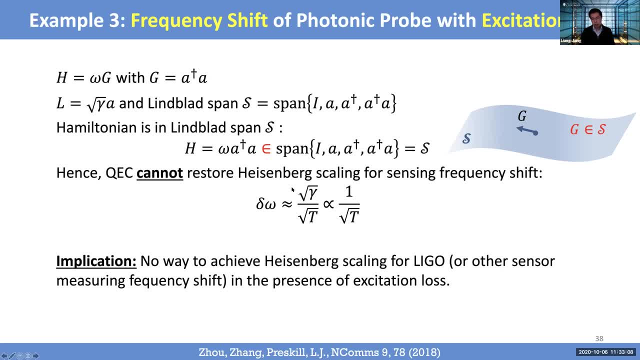 So therefore, quantum error correction cannot restore Heisenberg scaling if we want to sense the frequency shift of the cavity in the presence of photon loss- And this is kind of like implying that okay, there's no way to achieve Heisenberg scaling for LIGO. 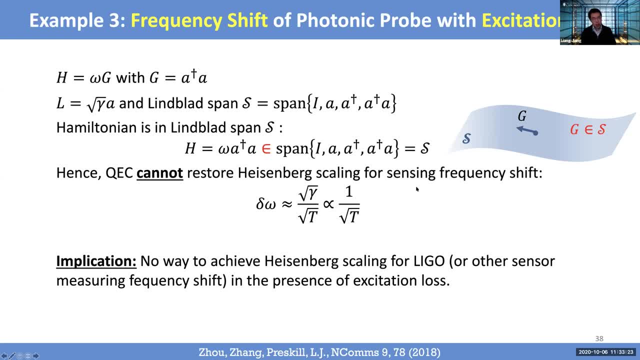 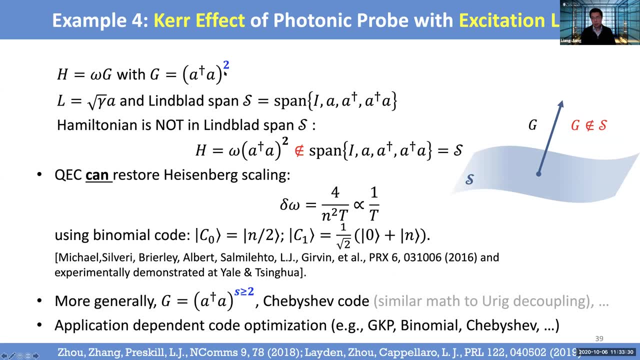 in the presence of excitation loss. If you have a signal which is not just a frequency shift, if it's a Kerr effect, A dagger, A square, then in this case still suppose you have photon loss. the Lindblad span is spanned by this linear. 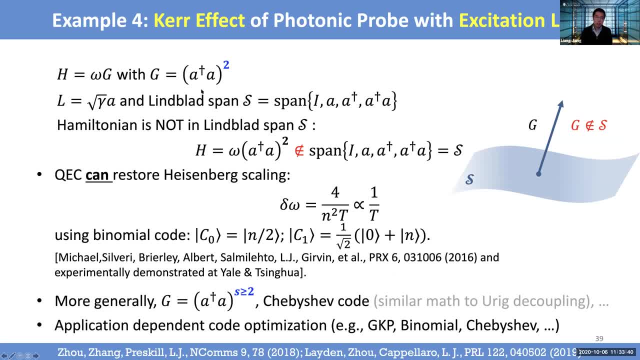 or quadratic combinations of A and A dagger, Then this Kerr effect is aquatic with A and A dagger. So it's not in this Lindblad span which indicates that there should exist a good error correcting code to suppress photon loss errors while achieve Heisenberg scaling for sensing. 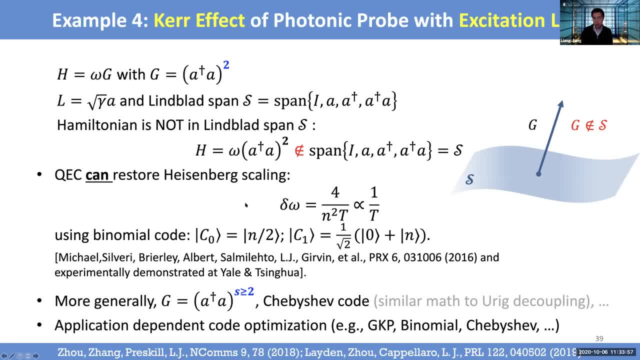 the Kerr effect And it turns out it's possible, And the one of the code to do it is something called the binomial code, which was invented, like by my colleague, Steve Gervin and a few others while we were trying to do error correction. 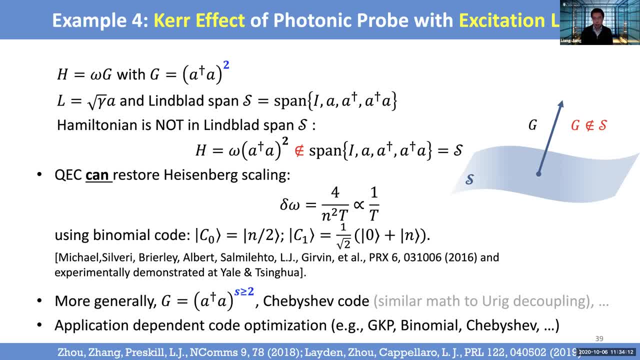 And it turns out that code is also useful to sensing Kerr effect and suppressing photon loss And intuitively you can see it as a code word. The C zero is just a fog state which has a photon number n over two. assume n to be an even number. 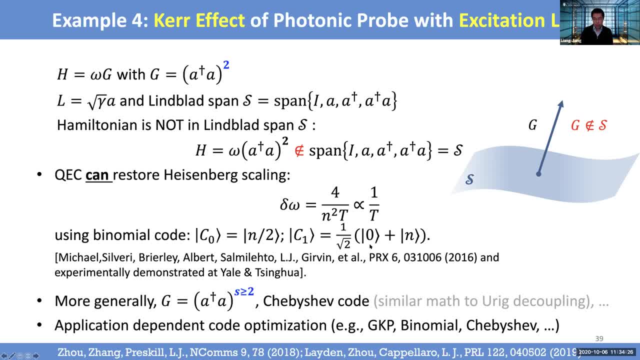 And the other thing that we can see, which is that you know other codeword is a symmetric superposition of a vacuum and the fob state N, And notice that these two codewords have equal average photon number, which enables it to actually like: have no back action from the photon loss. 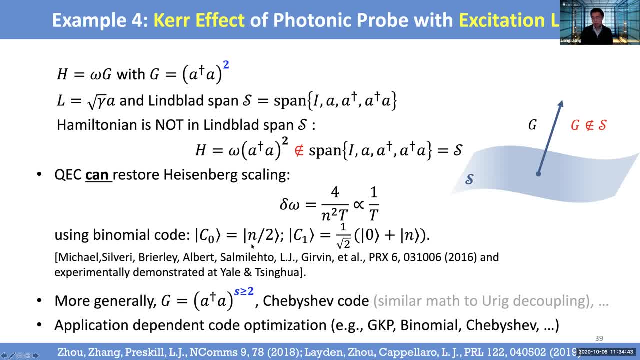 to the first order. In addition, these two codewords has a different variance of the photon numbers, because for C0 there's no variance, for C1 the variance is in the order N square and that enables us to be sensitive to the Kerr effect. So basically, this codeword, allow us to both simultaneously correcting. 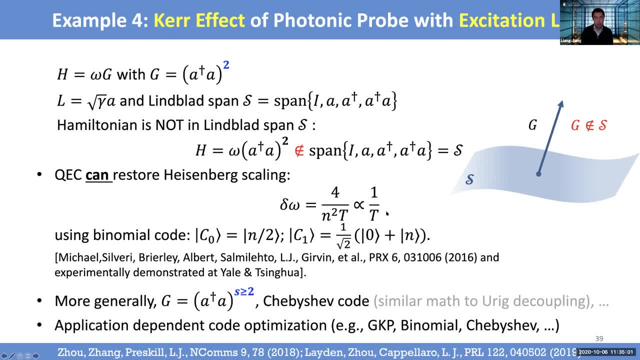 photon loss while be sensitive to Kerr effect. And that turns out that you can restore the Heisenberg scaling as calculated here, And actually there are more codewords that allow us to actually achieve, like the Heisenberg scaling for Kerr effect or higher order Kerr effect And, in case you're interested, you can. 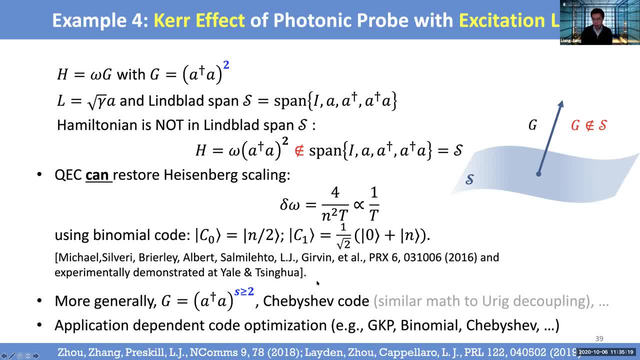 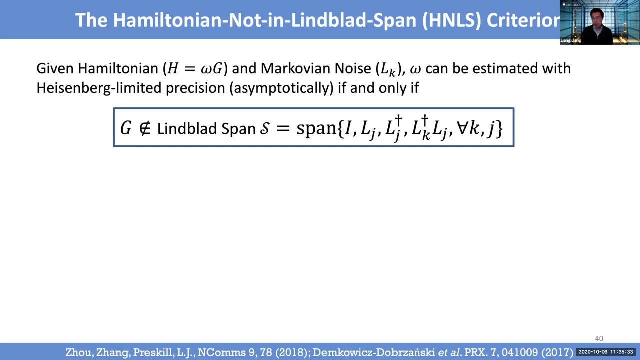 look into this PIL paper which gives you the answer to this question. It gives the Chebyshev code and that allow you to systematically approach the best sensing limit. So maybe, just as maybe, a summary on the perspective for this part which basically we can, the key condition, maybe a key take-home message. 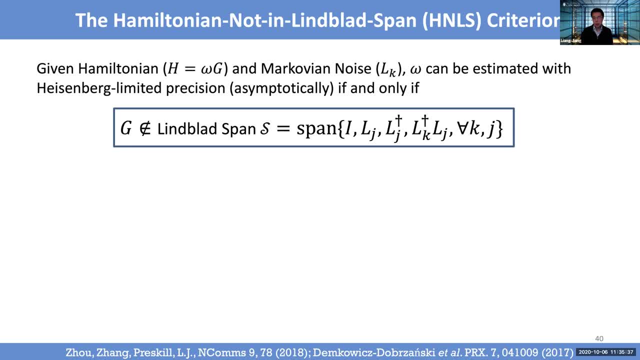 is, there's some operator space which contaminated by the noise, the Markovian noise, which is called the Lindblad span, And if your Hamiltonian is not in that Lindblad span, then you're lucky, you actually can do Heisenberg limited. 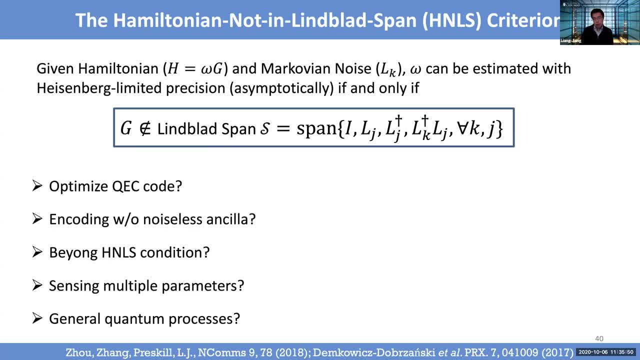 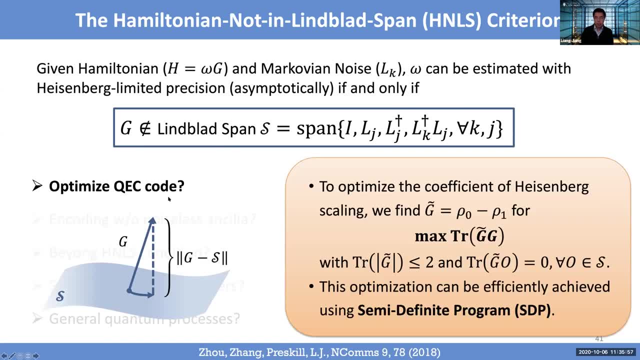 sensing with error correction And there may be a few related further generalization to this question. One question is: can we optimize the error correcting code so that we can maximize our coefficient associated with the Heisenberg scaling? And the answer is yes, And we can actually maximize the design of the error correcting code by performing efficient. 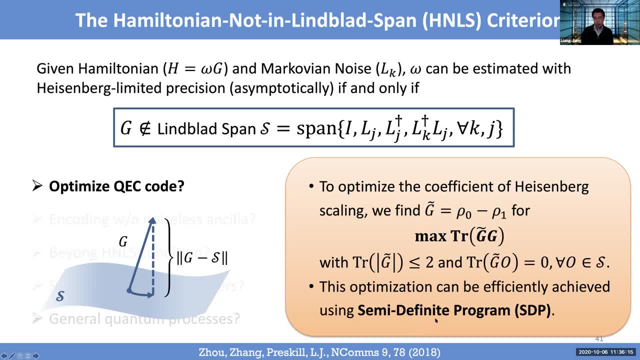 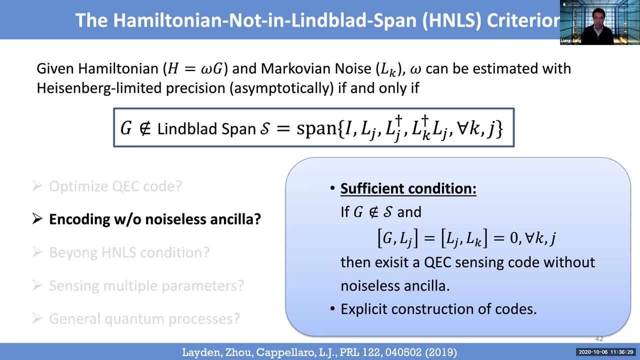 calculation using semi-definite programming And that allow us to come up with a good codeword that's optimized. The second question is: can we encode without additional noiseless ancilla? because that seems to be a very strong condition and turns out it's. 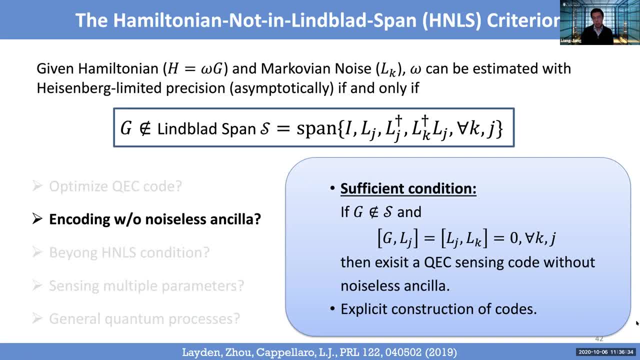 actually possible, at least we have a sufficient condition. if the generator of the Hamiltonian is not in the Lindblad span and also Hamiltonian commutes with the Lindblad span and the Lindblad spans commute with themselves, then there exists the quantum sensing code that do not need additional noiseless. 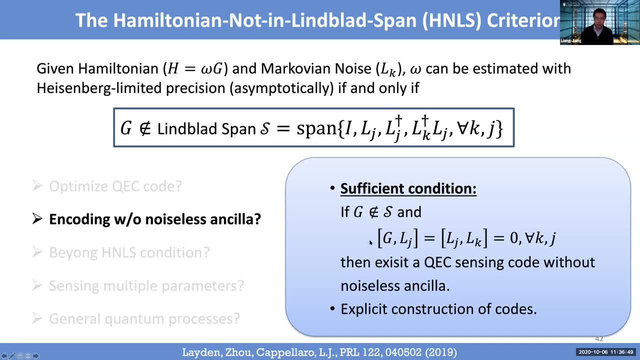 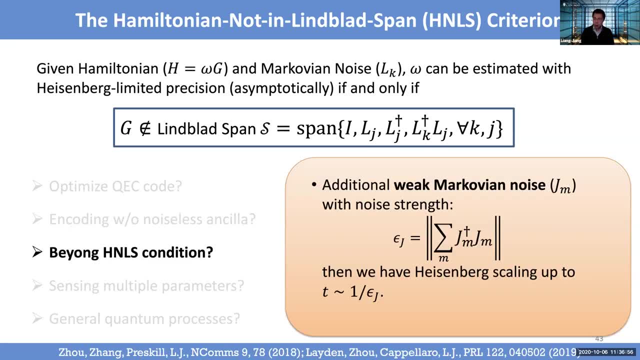 ancilla, But basically they are scratching and the code space can already like. just without additional ancilla we can already do coding. And the third condition is: in practice, however, this condition may not be perfectly satisfied. Maybe there is a small component of the jump operators that might cover or contaminate. 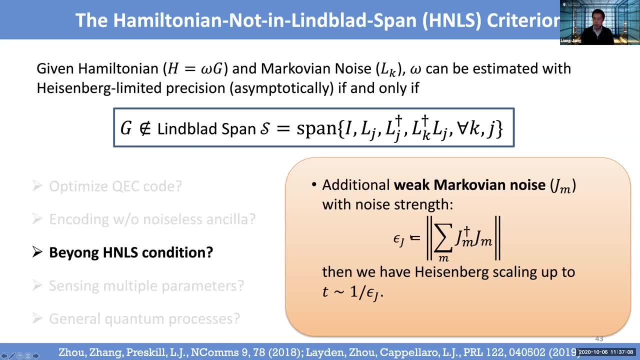 our Hamiltonian. But if that's really weak, then probably we can estimate the strength of those and kind of small noisy part which we might not be able to correct with our error correction. Then that gives us at least a boost And improve the range of Heisenberg, scaling up to a certain time scale which is 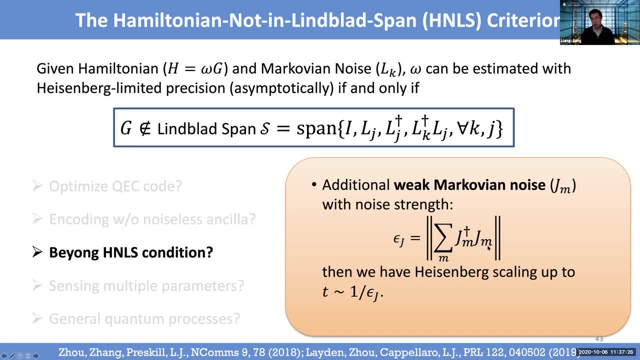 associated with the inverse of the strength of those jump operators. So we can kind of guide the design, that maybe one can design error correcting code to suppress the dominant part of the noise, And if there is a tiny bit apart which is just left behind, it's okay because at least 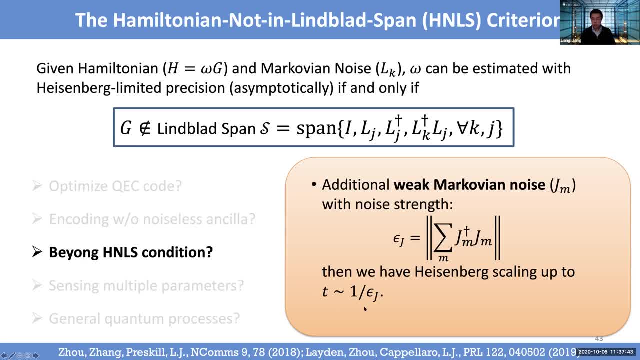 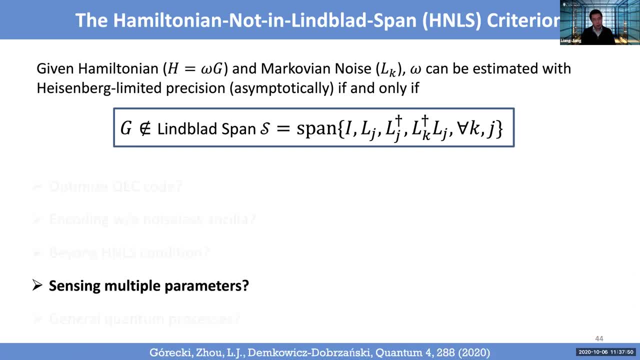 we can boost the performance up to the time scale, which is limited by the small part of the noise that we cannot correct with error correction And, if you want to sense, multiple parameters, which is also a relevant situation in practice, is actually we can further generalize this condition. 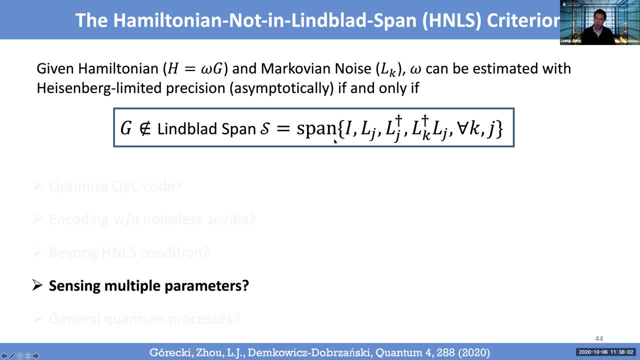 So if you look at this condition, we say Hamiltonian, not in Limbless band, which can be equivalently stated as the perpendicular part of the Hamiltonian with respect to the Limbless band is not zero. Or mathematically you can say another way, is saying that the perpendicular part of the 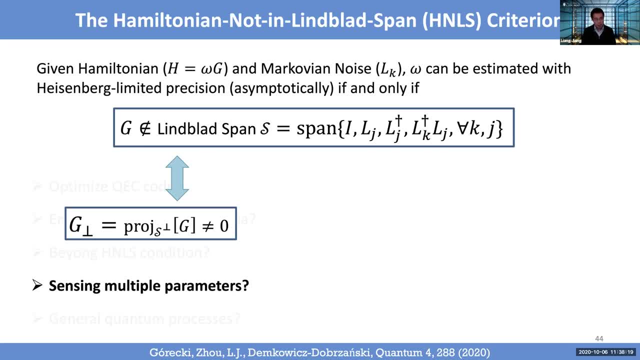 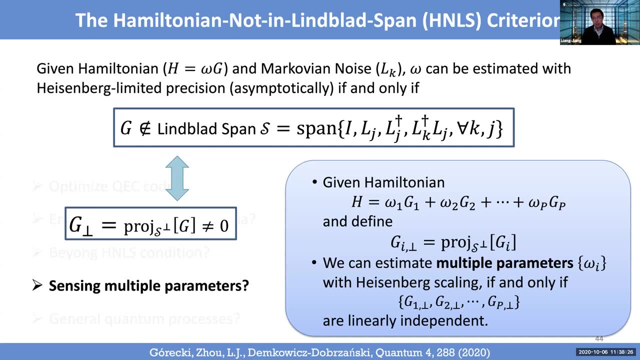 Hamiltonian is linearly dependent. Okay, Here I just have one term: If it's not zero, it's not linearly dependent. So then, if I have multiple Hamiltonians, multiple generators, I want to sense the coefficient associated with the generator of the Hamiltonian. then the generalized condition is that those 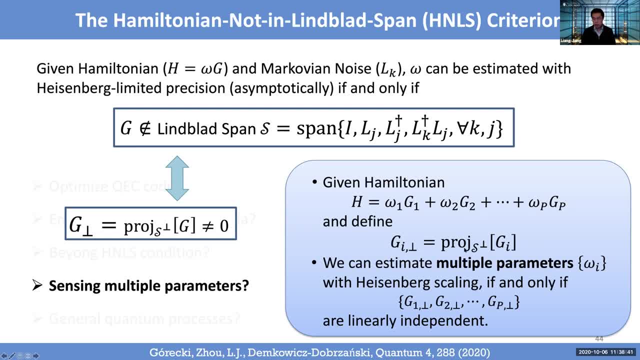 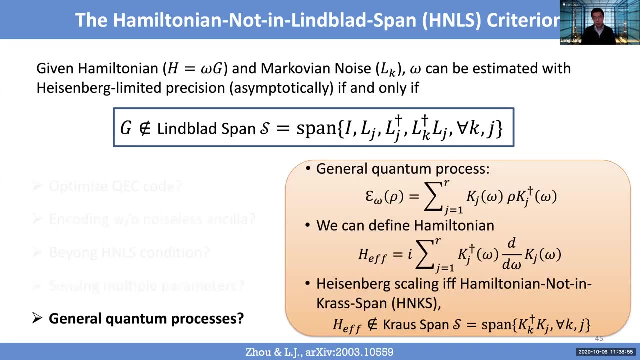 perpendicular part associated with the different generator of the Hamiltonian. they should be linearly independent, And it turns out that's a necessary and sufficient condition For multi-parameter sensing, with Heisenberg scaling assisted by error correction. And, moreover, we can further generalize this from the Markovian noise, which is this Limbless: 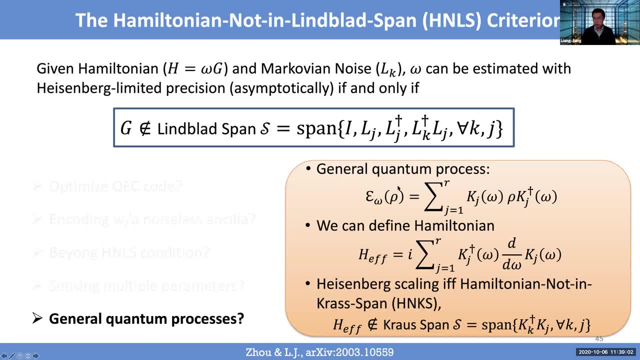 mass equation to the general quantum processes characterized by the CPTP map And in this case these cross operators are associated with the CPTP map. We can define effective Hamiltonian which is associated with the kind of the derivative of these cross operators. 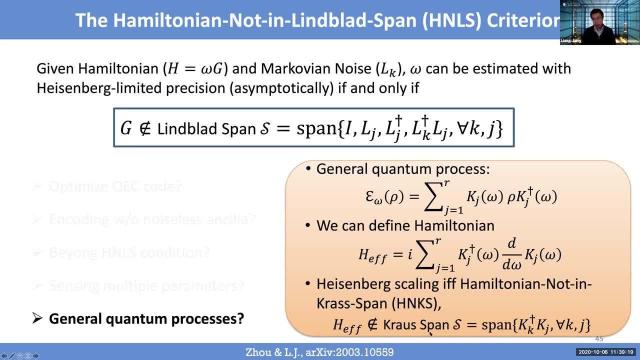 And if this effective Hamiltonian It's not in this cross span instead of the Limbless span, which is the span of the cross operators, then actually we can show that's a necessary, sufficient condition for our Heisenberg sensing, Heisenberg scaling sensing assisted by error correction. 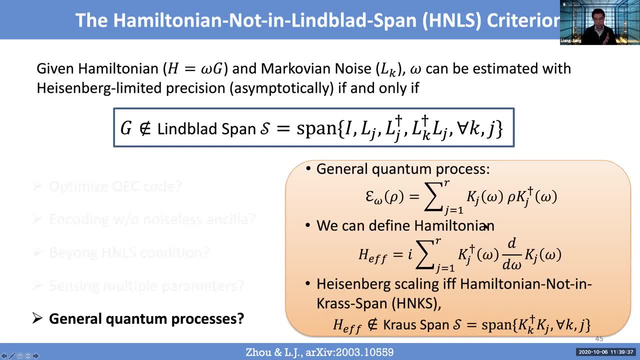 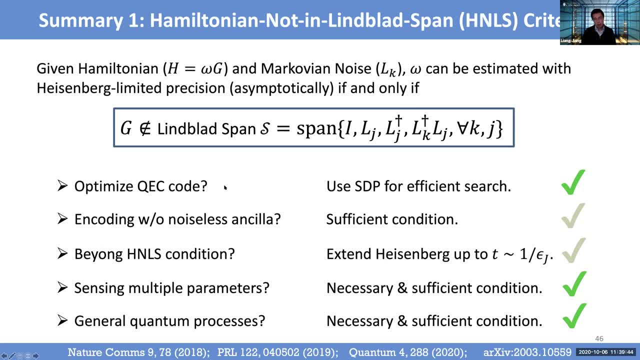 So this is kind of you can think of it as a generalization to a more general quantum processes. So maybe just as a summary for the first part is basically we developed like an optimized error correcting. Oh, we can, We can further extend the results of Hamiltonian Limbless span by consider optimized code code. 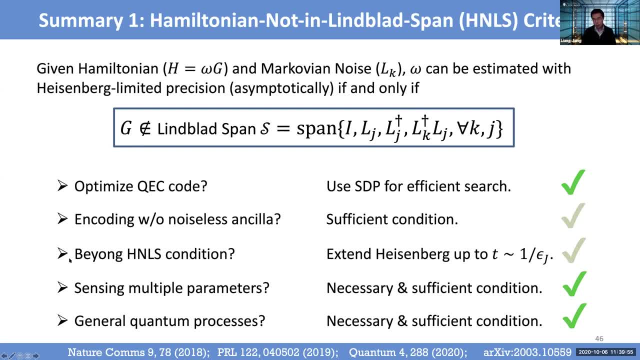 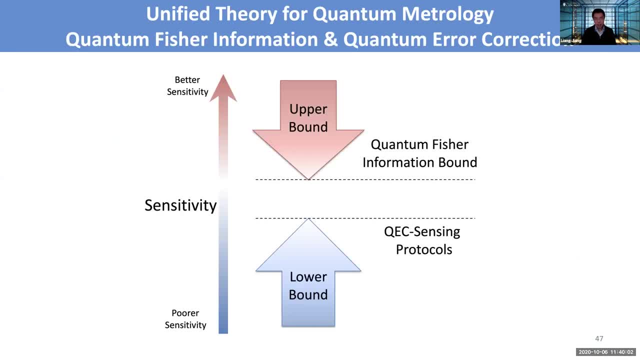 with noise. this answer that beyond the Hamiltonian, not the Limbless span or multiple parameter or general quantum processes. So maybe the the the bigger picture is basically you can think that you have upper bound from quantification information and you can also show some lower bound by explicitly constructing. 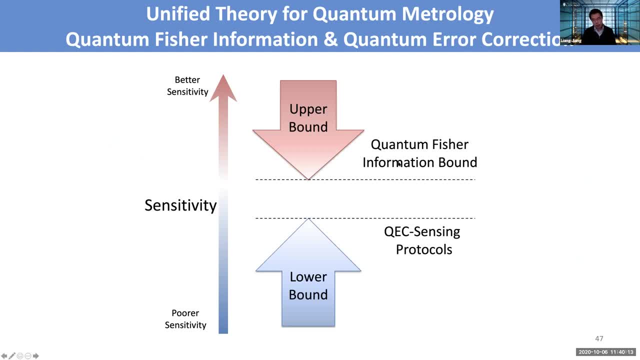 quantum error correction and by further computing better upper bounds or design better error correcting codes So you can get the two closer and get a tighter kind of a pro, probably like a designer code that saturate this upper bound. Yeah, Oh, yes, Marius, had a bunch of questions but you seemed like you were on a roll, but would now be. 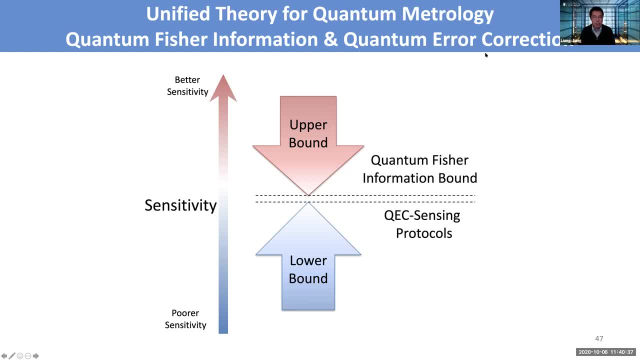 a good time. Yeah, Yeah, It's a. it's a good time, Yeah, Hey, Marius, do you just want to unmute because you have several questions? Yes, So I will just focus on the most important one. 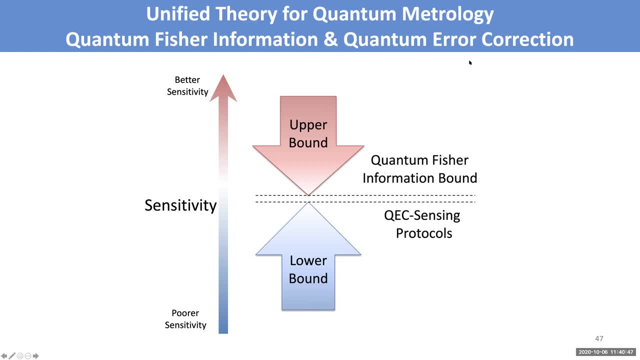 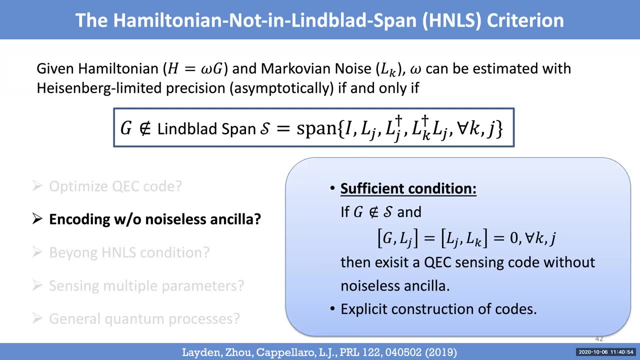 If you go back to page 42.. I guess 42 or 43, you had a sufficient condition for right. so so do you really think that the commutativity of the Lindbladians here is necessary? I have the feeling that should not be necessary. 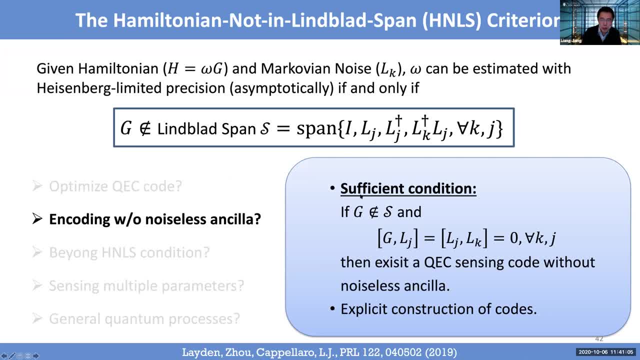 Yeah, it's probably not necessary, But here we can just only prove the sufficiency with this condition. And yeah, I think that. I mean, yeah, I have the feeling, if you know have no extra Hamiltonian part In your Markov, then it should be okay, then they should. you don't need the commutativity. 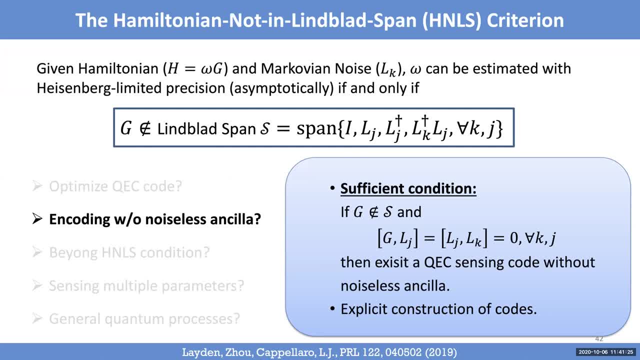 condition. That's what you know, my perspective would suggest, but that's just a guess, of course. And then I have one question. This is probably at the beginning, when you did this gamma t and dt, right? So yeah, so, so there is. you're losing this probability, gamma t- is that not an issue? 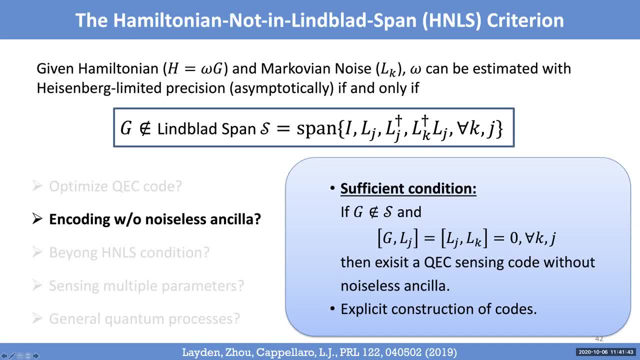 How can you renormalize this? I mean mathematically, I can just, you know, divide by Yes, By gamma t, and then then I'm fine. But can this be done physically? this is always a mystery to me how you can renormalize if 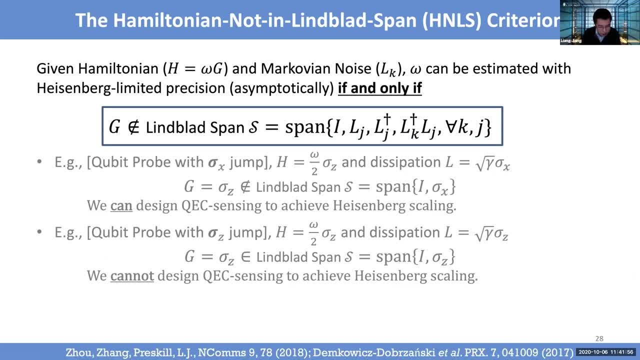 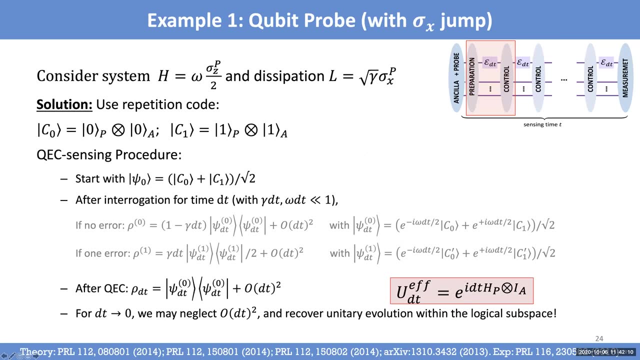 you have lost probability. So let me see, if you're like, if there's an example like so, I will refer to this slide. there is Right, exactly. So if you look at the gamma t there, right, this is small, it has to be small. 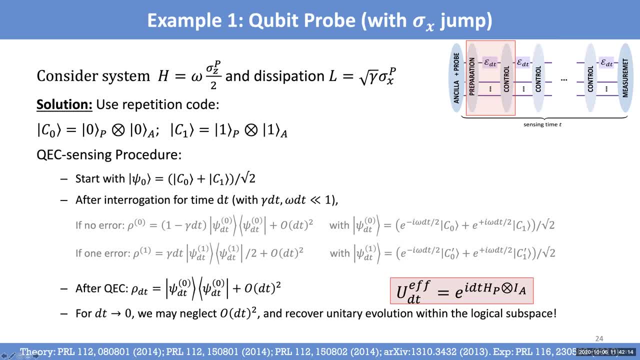 It has to be small. So you're somehow dividing by gamma t And then this square should disappear, if I'm not mistaken. but you know right, because you're dividing by order t. but you know physically, how can you? how can you somehow? 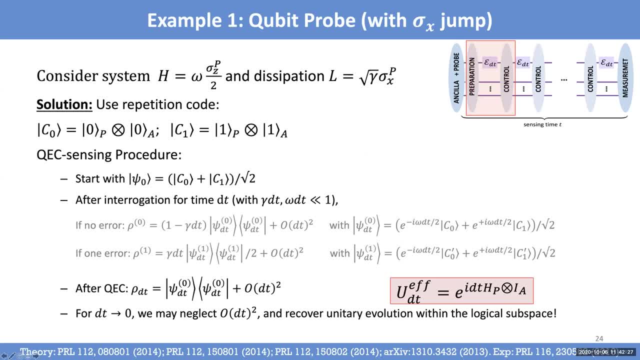 ignore this, this factor, because it's no longer a state, right? Yes, So one intuitive way of thinking. it is something kind of like a quantum Zeno effect, So if, but? here it's kind of like if you suppose, like if you're looking at a state. 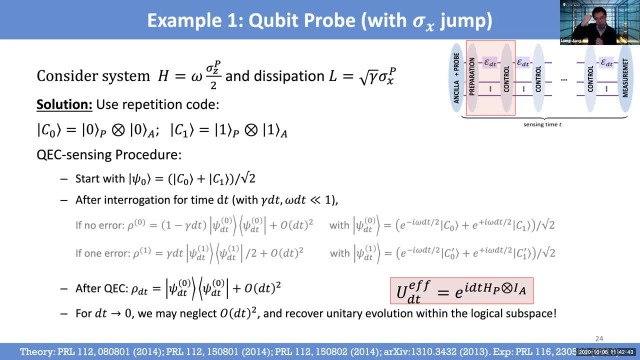 which you want to do, a rotation from once kind of from one state to the other, Right, And if you keep measuring it, then basically the probability that it flip will scales as a square of dt. And if you keep measuring it, basically if and set a limit, dt equals to zero, it actually 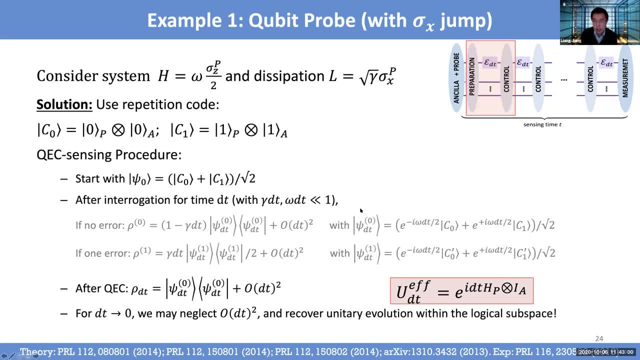 vanishes. Or here maybe I can think, say another way, is that suppose I cut this entire evolution by n n steps, okay, And the probability of this dt square will go as a one over n square. Oh, different scales, Yeah. 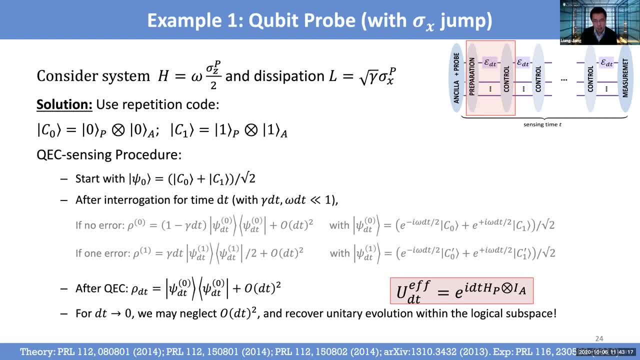 Different scaling behavior And that helps you. That's right. Yeah, Okay, good. And then just one extra comment. So you have this sequential model and the parallel model? Yes, But if you do the parallel model with the tensor product of the of the time evolution, 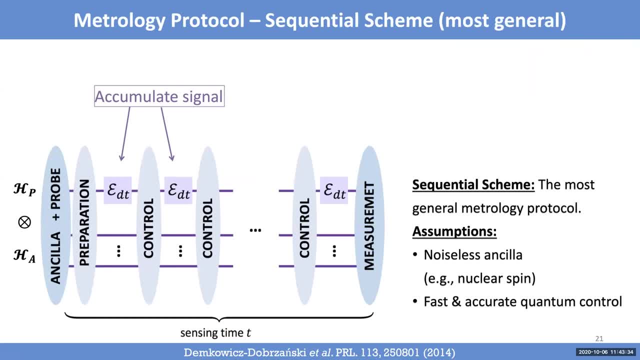 you have larger code spaces which leave, which are completely left, invariant, right, Because the tensor product always produces, and isn't that helpful, because there you could use that to send some some Hamiltonian, Yeah, Yeah, Yeah, Hamiltonian or something. 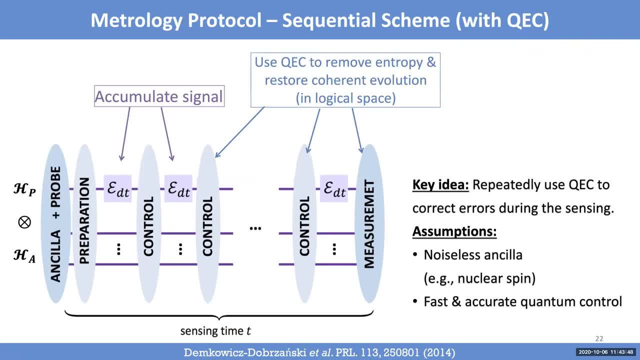 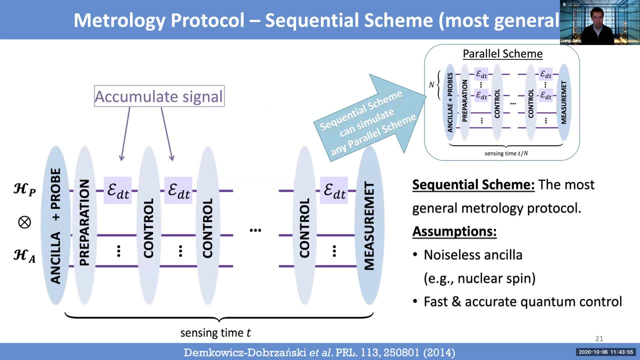 You know, if you use these error unaffected spaces, is that not useful for your analysis? I agree it might be useful, But that can also be simulated with our sequential scheme. So you can think that you have a single probe combined with n minus one ancilla, which those? 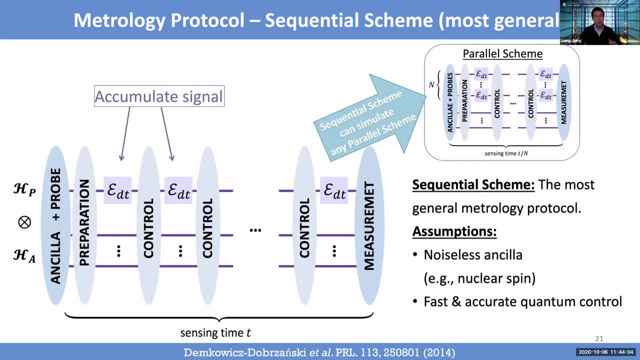 n minus one. ancilla actually stored this effective like n minus one probes And so, effectively, your single probe and n minus 1 probe will be prepared. be prepared in some like a permutation in space if we need that one. yeah, Okay, so it comes from the simulation. 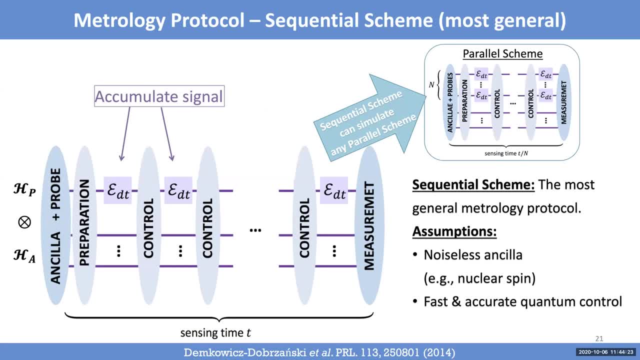 and you're losing the factor n, right? So exactly, yes, And which is shown here, Yeah, so here I have this sensing time t, and over there it's a sensing time like t over n, So the difference disappears in that analysis. 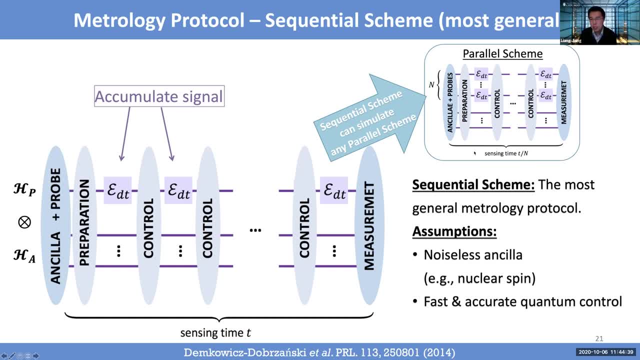 Okay, thank you, That's right. yeah, Thanks, Mariusz. Eric also had a question on the slide that you were sitting on at the end with the quantum Fisher information and the quantum error correction, Yes, And he was asking: how are you lowering the upper bound in that case? 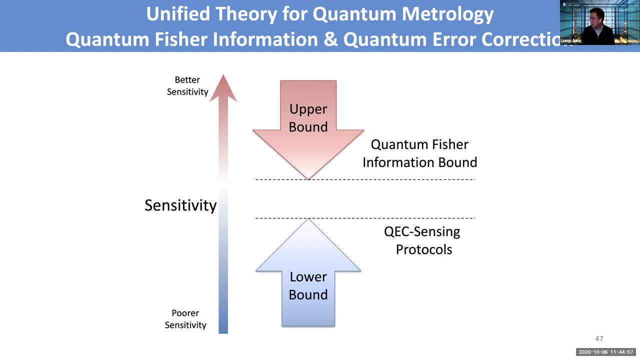 So, regarding the lowering upper bound, this is more kind of in the context of like a market parameter sensing, And if you have the parameters, the tricky thing is that you may have operators which may not commit with each other And for those sensing case, 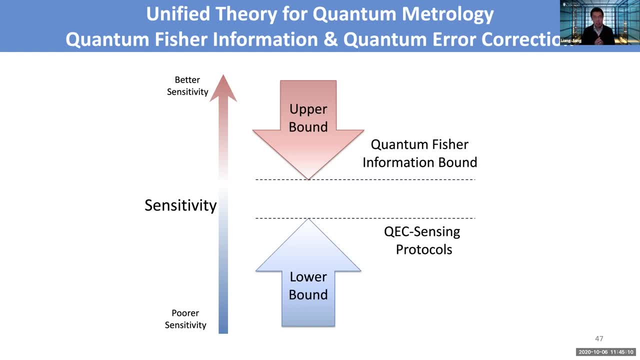 that actually quantum Fisher information bound is not tight and you need to use this like a high level, like a sharing information bound, So that will give you a tighter bound And they are like it's more involved in the calculation, but that actually can further improve. yeah, 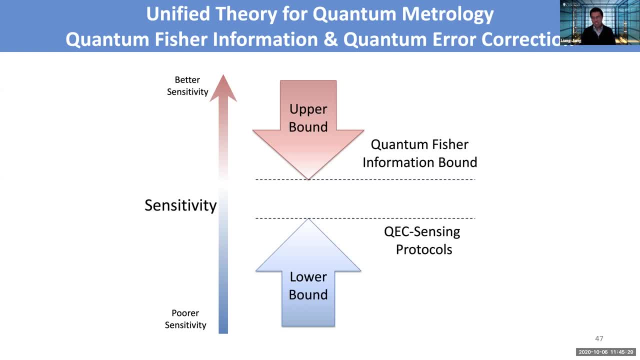 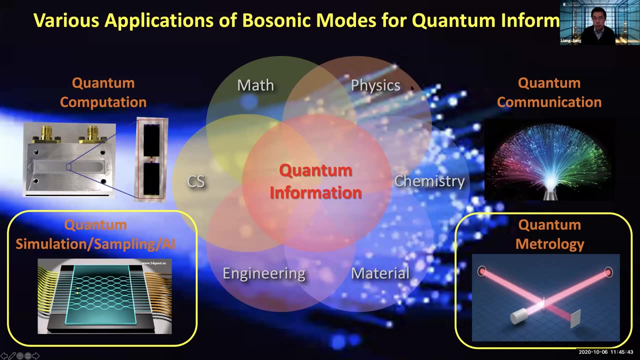 But I agree for single parameter, the quantum Fisher information bound is. it's there, yeah, Okay so, yeah, shall I move on to the next part? Yeah, so the next part is about this quantum. let me about, like a quantum simulation. 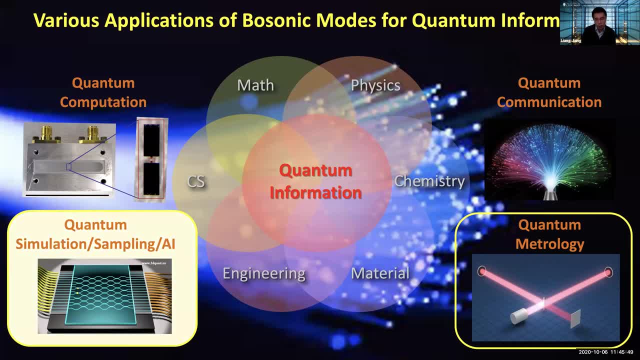 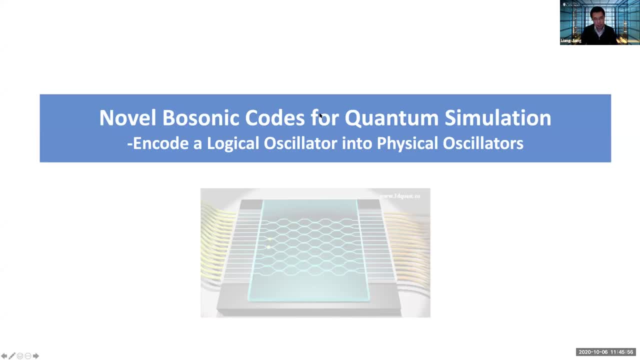 And so one question is actually like probably people might heard about, like we can use the both on system to do both on sampling, which is actually if ideally there is no loss, it might be very difficult to simulate and to get the statistics from classical computer. 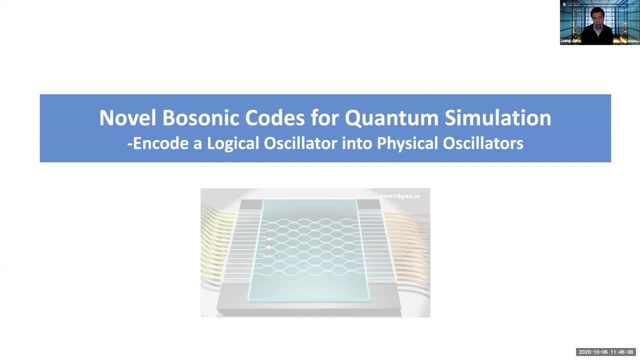 And so one question is that indeed the system has loss. And then can we actually overcome the loss while preserving the bosonic nature, so that we can do something like boson sampling or maybe simulating bosonic systems? And if you look at all the codings with the bosonic modes, 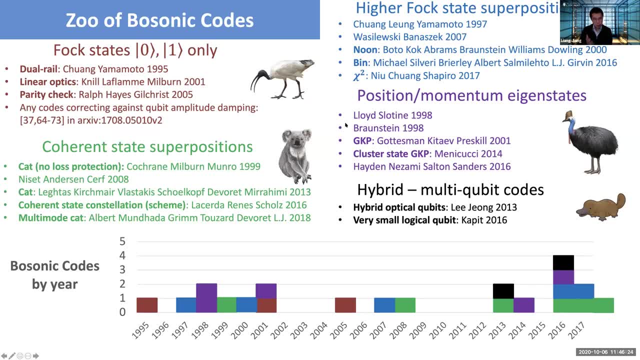 actually most of the coding is actually encoded d-level system or qubit, or d-level system using bosonic codes, And this is kind of like a summary of the progress up to maybe 2018, like prepared by my former student, Victor Albert, when he was having a trip to Australia giving 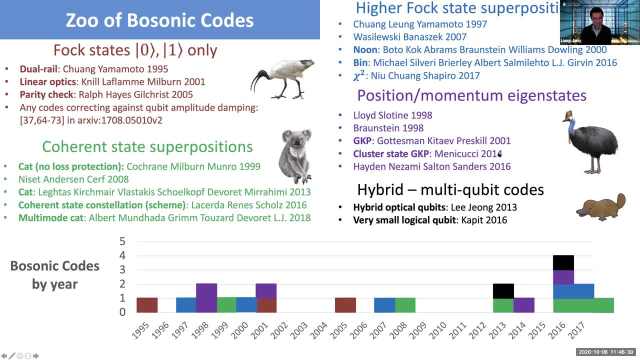 talks there. So you see lots of strange animals in Australia. But I guess the key idea here I want to show is that actually there is so far we do not have a code which can simultaneously correct loss errors while preserving the boson statistics. So the natural question is: can we encode a logical oscillator? 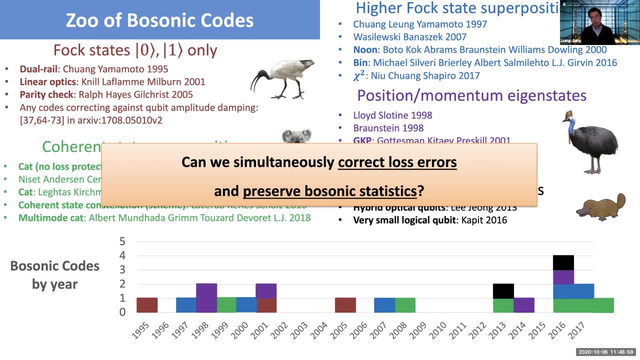 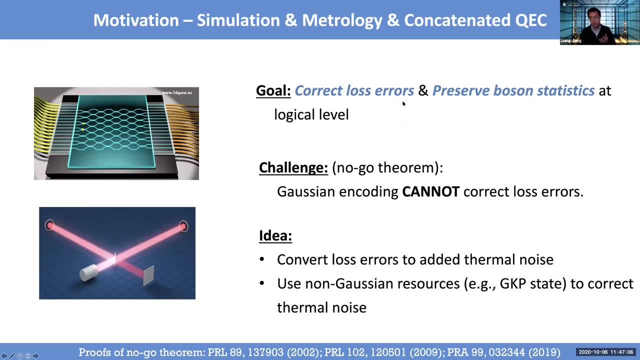 using multiple oscillators while correcting loss errors. Okay, so basically, the goal is to construct some like lossless and preserving the bosonic statistics at a logical level And the actually there's a no-go theorem. that, because this is the question, which it's actually very natural and people have thought about it early on. 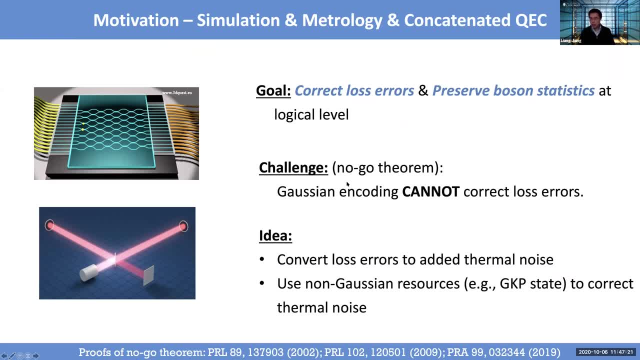 And actually like there is no-go theorem saying that if we just use beam splitters, squeezers, Hamilton detectors, you actually will not be able to achieve such a goal, because all those are Gaussian operations which effectively can be achieved by something like a quadratic Hamiltonian. 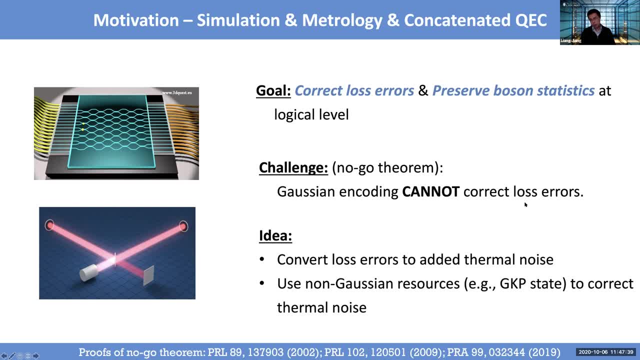 or those evolutions that cannot correct loss errors. Okay, Because the Gaussian operations kind of can and otherwise. you will be able to get kind of like improved, like entanglement distillation using just Gaussian operations, but it's actually not possible in this case. 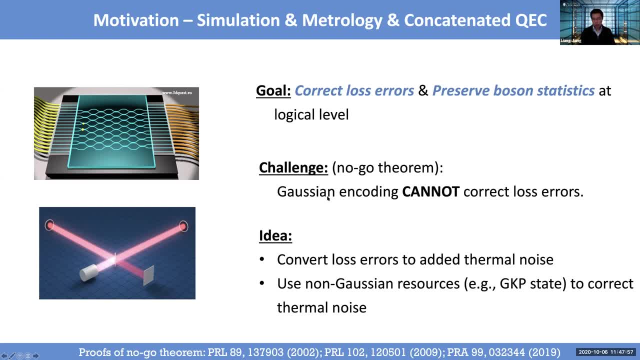 So now we actually want to overcome this challenge of no-go theorem, And the way to do it is to change the conditions of the statement of a theorem. The condition is a Gaussian encoding will not work And we try to do something which is non-Gaussian. 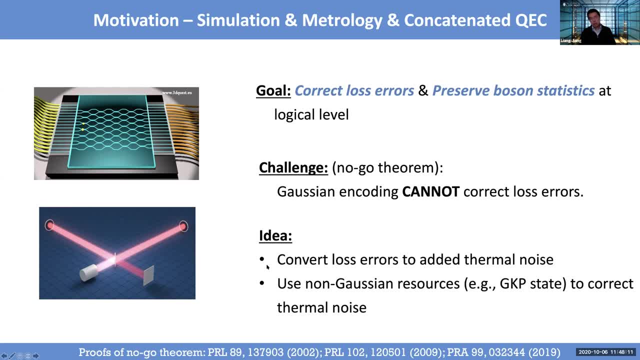 So basically, the idea consists of two steps. So first is that we want to convert the loss error into something called added thermal noise error, which is easier to handle. Secondly is that we want to introduce some non-Gaussian resource which is called the Gottesman-Kittayev-Preskill state. 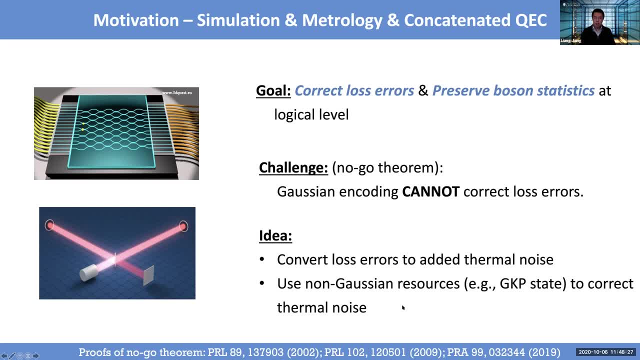 that can use to correct thermal noise error. Okay, So in the next two slides I will first explain how we convert loss to thermal noise. Second slide: I will define what the GKP state is. So first how we convert from a loss error to thermal noise. 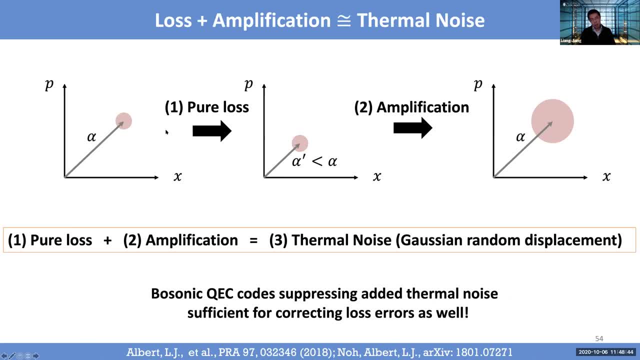 So suppose I have a pure coherent state, I have a loss. Basically it goes the attenuation, the amplitude of coherent state, But the amount of noise is still have this equal amount of uncertainty because the coherent state and the loss still goes to a coherent state with a reduced amplitude. 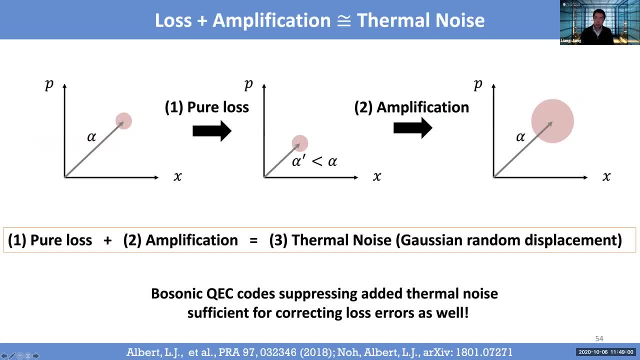 Now what I can do is I can apply a phase insensitive amplification Just to perform a two-mode, squeezing over this mode and an ancillary mode which start in the vacuum, And that allows me to do amplification. So with amplification you actually increase amplitude, but at the same time 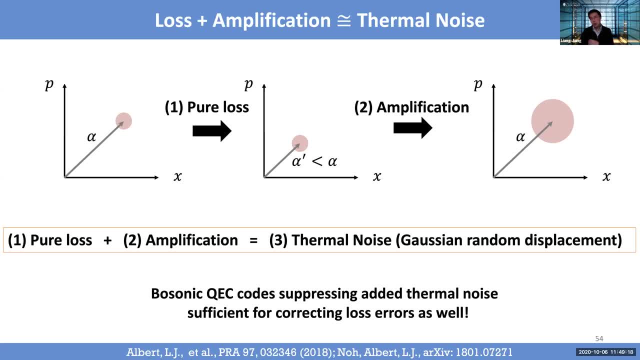 you introduce some additional entanglement with this additional ancillary mode which shows up here, as there is a bit more uncertainty associated with this particular state. So basically, the pure state, pure loss, combined with amplification, actually gives you something, effectively the same as the thermal noise added to the bosonic system. 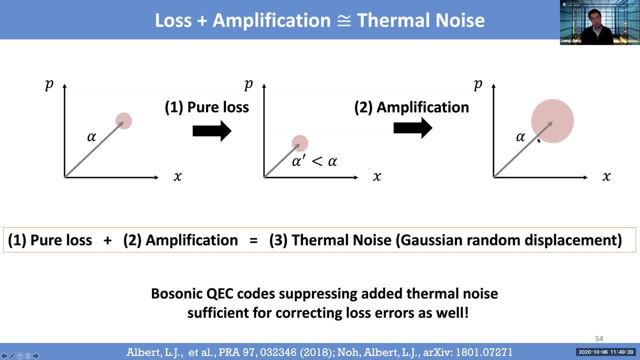 So now, if we could develop a bosonic code that can correct this added thermal noise, Then essentially we can actually correct the photon loss as well. Okay, so the logic is that if you have loss error, let's say I can amplify it, make it to thermal noise, and then I can use error correcting code to correct thermal noise. 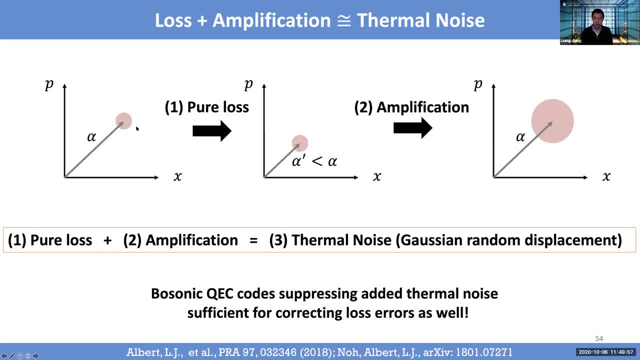 to correct loss error. Now, with that said so, basically from the rest of the discussion, I was just discussing how to suppress thermal noise. Okay, now, in order to suppress thermal noise, there is actually a very interesting code called the Gottesman-Kittayev-Preskill code. 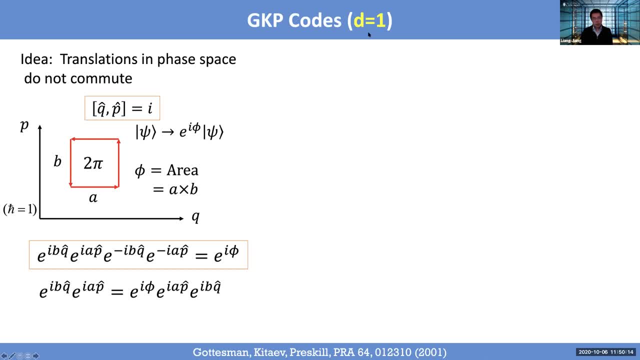 And it's basically considering a particular case where the code space has just one dimension, it's just a single particular code state that's actually defined as the eigenstate of a certain operator. So first we know that uncertainty principle says that the commutator come from the commutation between position. momentum is not equal to zero. 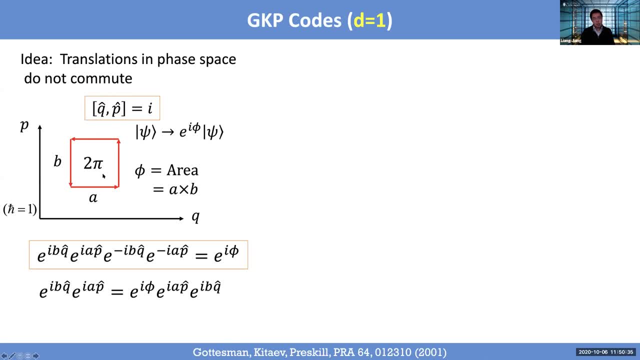 It's actually a constant i h bar, and that indicates that it cannot simultaneously measure position momentum to arbitrary position, However, and you can actually do something- evade this constraint. instead of measure position momentum, you can actually measure position momentum module or something that's actually possible. 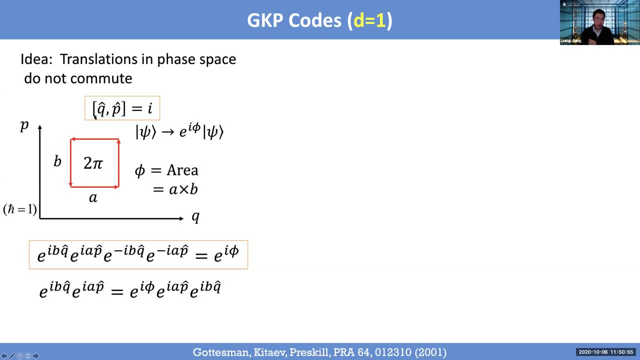 So, in order to show it here like one can first, from this commutation relation you know that if you make a closed loop in the phase space, you actually will accumulate a geometric phase which is proportional to the area in the phase space And that mathematically you can actually use the BCH formula to prove that the 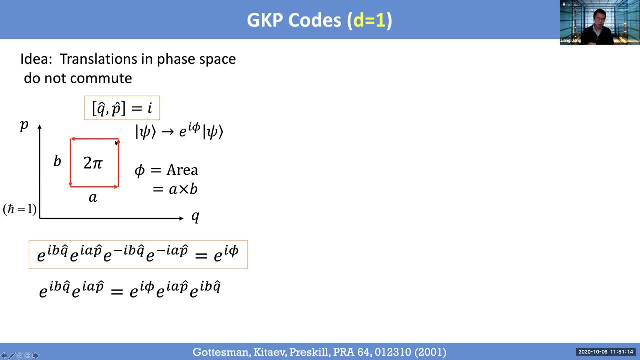 area in the phase space is equal to the area in the phase space. So if you first make a displacement along p, then displacement on q and then make a closed loop, this product of these operators is actually a constant which is proportional to the phase accumulation. and you can move some operators from one side to the other side. and if this 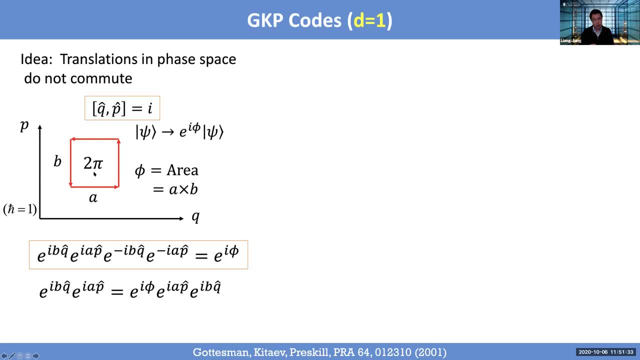 area happens to be integer multiple of two pi- and here I say the area is equal to two pi- then basically it indicates that these two operators will commute with each other. So if you make a displacement along the p or q quadrature, both by like a square root of two pi. 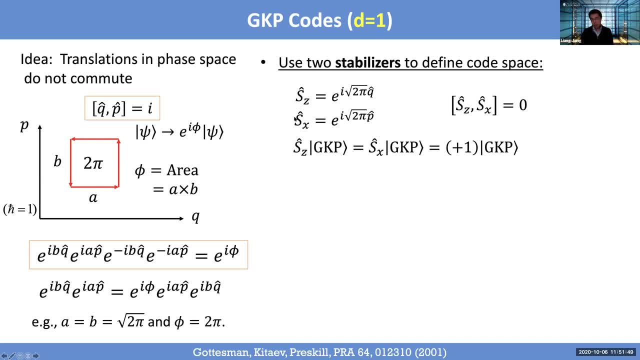 then those two displacement operators. they commute with each other. So if they commute with each other it indicates it's possible to find the co-eigent state of these two operators with eigenvalue, say, plus one, and turns out there is a one eigenstate which has eigenvalue plus one for both of these operators, which here we call the GKP. 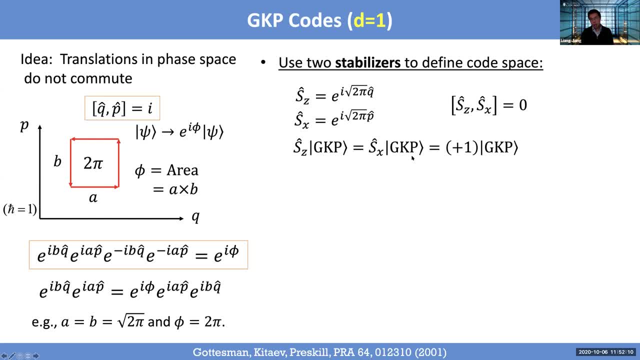 state and there is no information encoded here, because it's just a particular state defined by the co-eigent state of these two operators. and if you let it encode the larger areas, say 4 pi or 8 pi, then you can encode multiple qubits using the GKP state GKP code. but here we 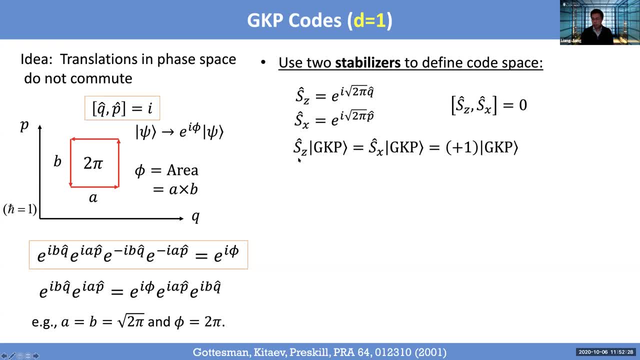 just need a particular state, which is the co-eigent state of these two operators. Why I need that? Because, first, it indicates that I can use this state to simultaneously measure sx and sz, which allow us actually to simultaneously measure modulo Q, Q, modulo root pi- root 2 pi, or position modulo, or momentum modulo- root 2 pi. 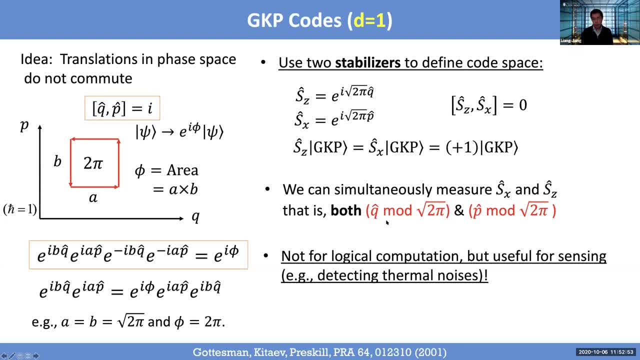 And this is actually allowed by quantum mechanics. If I remove the modulo square root 2 pi, then it's not allowed because I cannot simultaneously measure those. But if I put in this modulo square root 2 pi, actually these operators, they actually can be simultaneously. 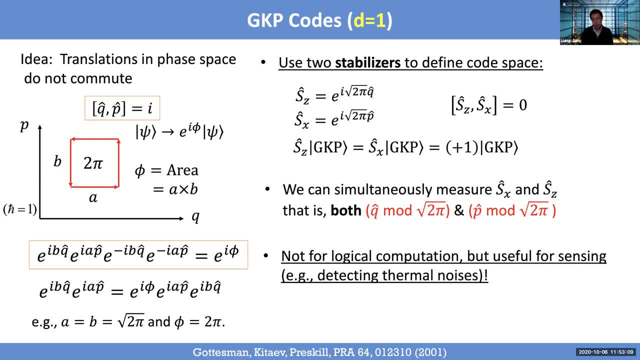 measured And that's actually useful because, if you imagine you have some states like the GKP states in here, if there's some additional thermal noise being added, you can actually measure these quantities and know how much the thermal noise is added to the system. 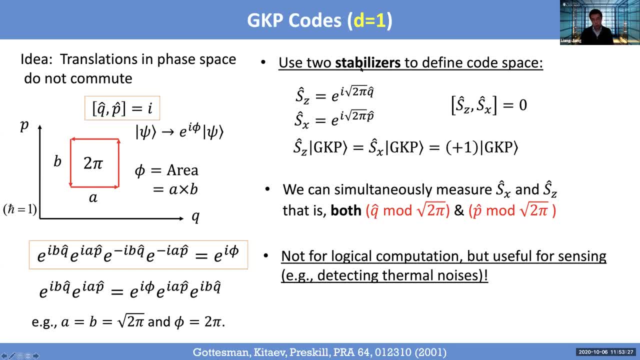 Okay, and here I introduce a particular, just as the trivial GKP states, because I'm not trying to do any logical computing. I just want to use it for sensing, To detect the thermal noise which later on we'll help us to detect or suppress the photon loss errors in order to restore a bosonic mode. 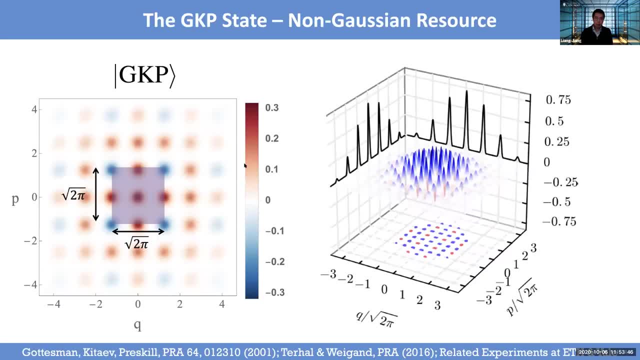 at the logical level. But just to give you some intuition about what GKP states look like, here is a Wigner function of a GKP state, with horizontal axis being positioned, vertical axis being momentum, And you see a periodic structure of a square root of 2 pi. 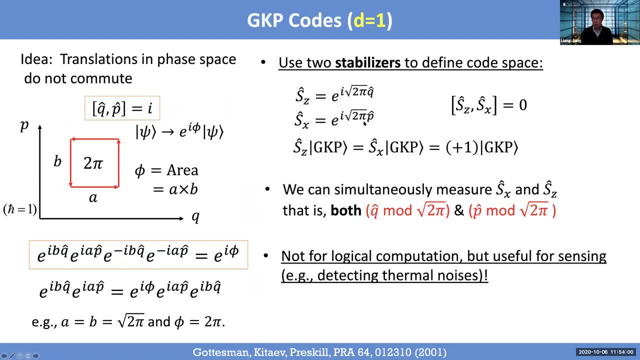 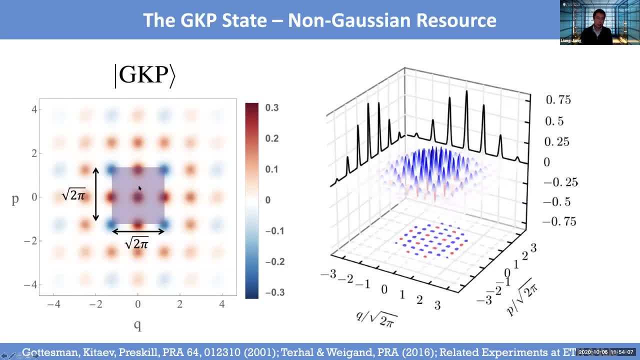 which is kind of consistent with this definition of a stabilizer, which is the translation It's indicating. the states should be translation invariant in position and the momentum by square root of 2 pi. And this is this lattice structure And I've kind of put a gaussian. 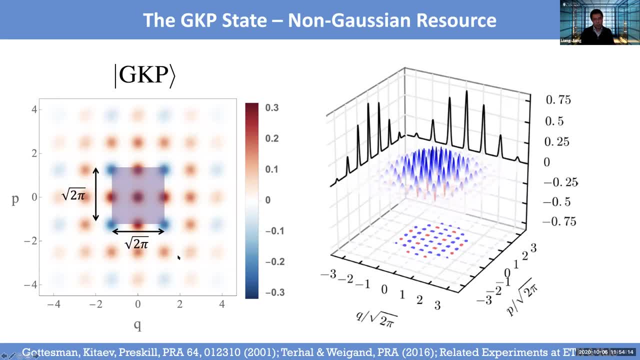 envelope on it so that at least I will not get the divergence in this expression. So, and here you can also, this is like a 3D plot of the GKP state with the Wigner functions. You see the positive, negative pattern And on the side you get the marginal probability distributions. 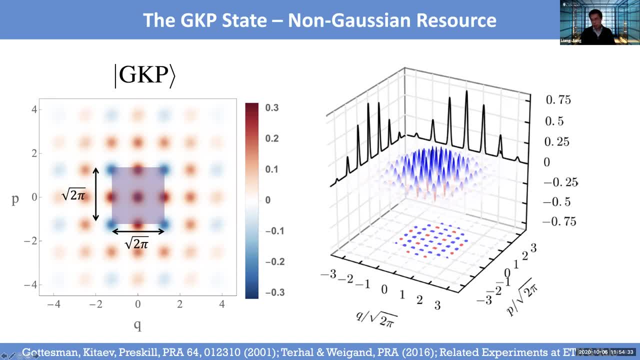 You see there's a kind of like spikes periodically spaced, That the periodicity is kind of exactly as the square root of 2 pi. So because of these spikes are kind of like very narrow and periodically spaced, it indicates if there's small displacement you will see the offsets. 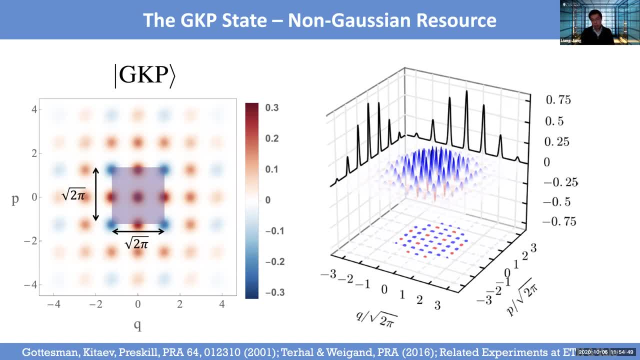 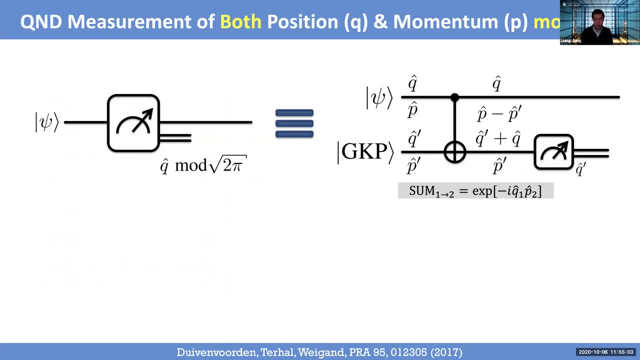 in these spikes And you can actually measure those quantities without destroying the whole state. So just to give you some idea like: so basically you can use this GKP state to measure the position modulo root 2 pi. So here is the example. Suppose I have a state. 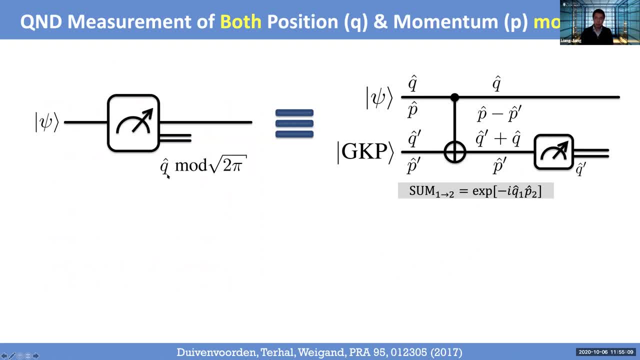 I want to measure position modulo square root of 2 pi. One way to do it is that I let this arbitrary bosonic states come in. Let's do a control sum gate between the bosonic state and the GKP state. So control sum is achieved by this unitary which is exponential of a position of the first mode. 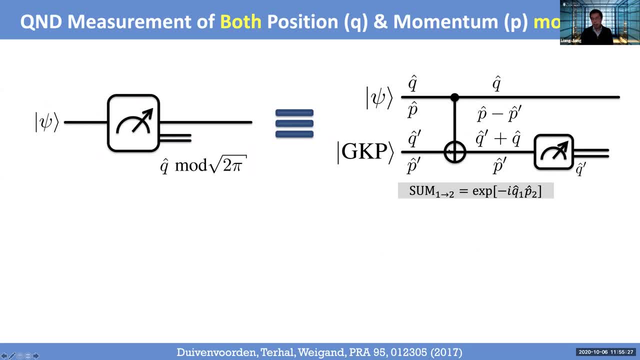 times the momentum of the second mode, And after this operation, you can think it as the position of the second mode being displaced by amount which is equal to the position of the second mode. Okay, While there's a back action, the momentum of the first mode being also shifted by something. 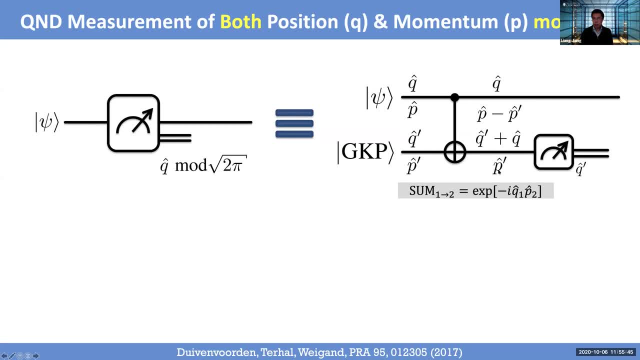 proportional to the momentum of the second mode, And that's allowed by unitary transformation. And then what you do is measure the position of the second mode, Because the position of the second mode is actually prepared in a GKP state. it has this periodic structure of modulo root 2 pi. So 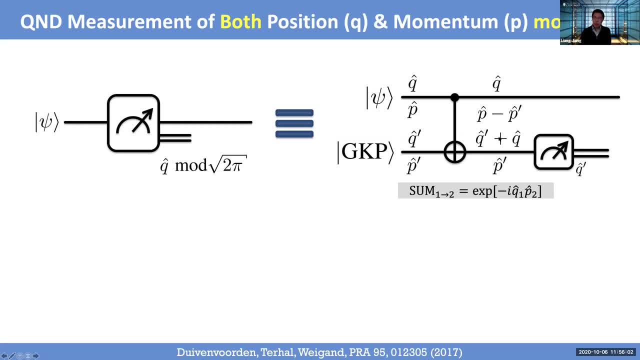 when I measure the position after this sum, I get the position of the first mode, which is modulo square root of 2 pi. Okay, So this is kind of a circuit to measure the position of modulo square root of 2 pi. Similarly, you can use a circuit to measure the momentum of modulo root 2 pi by using the same 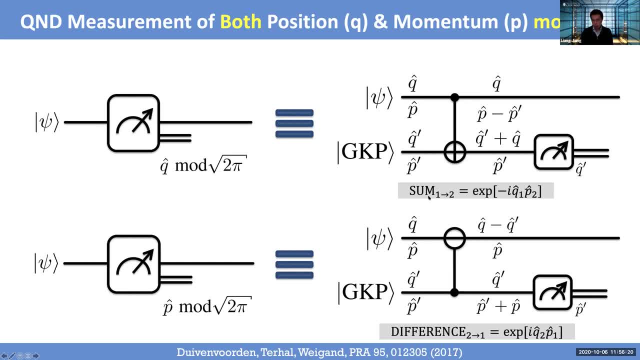 GKP state And by performing a control sum gate you actually perform something like a difference gate And following the similar mathematics you can derive like you actually can measure momentum modulo root 2 pi. So this is kind of explicitly showing you can perform sort of like. 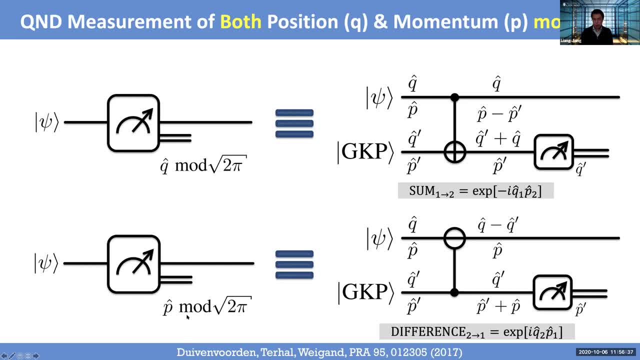 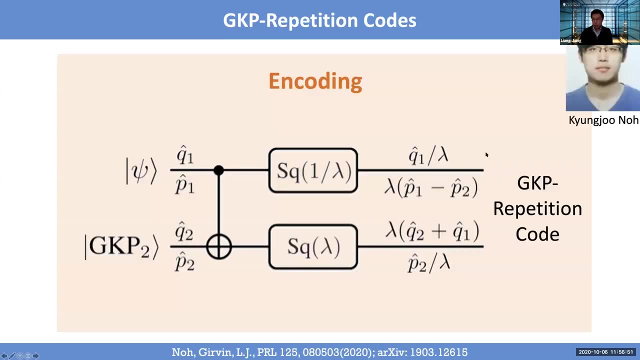 a non-demolition measurement Opposition modulo root 2 pi and the momentum modulo root 2 pi, using this additional non-Gaussian resource of a GKP state. Okay, So, with this preparation, actually I can show the coding of this GKP repetition code, And this is actually invented by, like, Ken Juno. 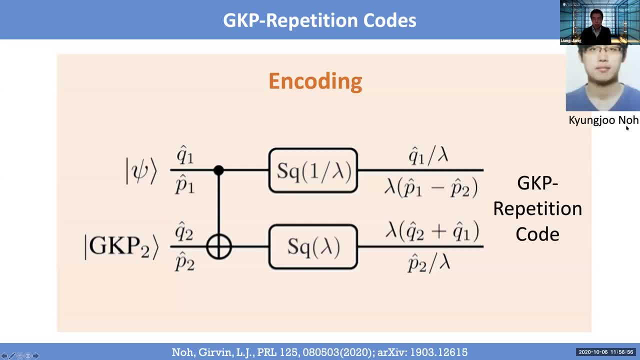 who is also a former student in the group and recently joined Amazon AWS. So here the idea is basically: you have an unknown state you want to protect You. let it couple and be entangled with GKP resource, non-Gaussian resource. Okay Now, after this operation of control, sum gate. 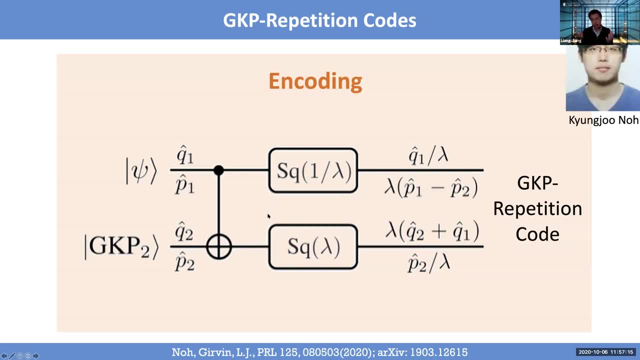 you get the entangled state between the mode that you want to protect and the GKP ancilla, And then you perform some squeezing operations to massage the state so it looks better, And after that you actually prepare the GKP repetition code. And now here I'm just going. 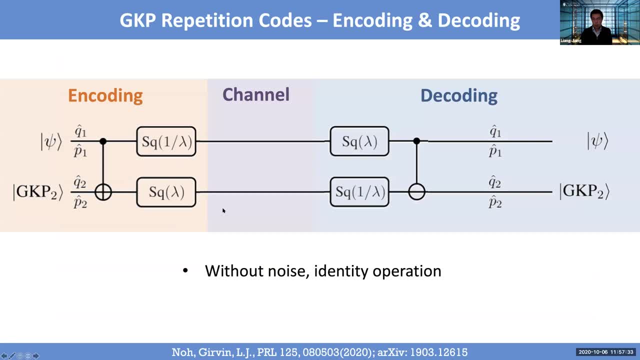 to illustrate how we actually use the GKP repetition code to correct errors. So the decoding procedure is the inverse of the decoding. Basically, if you squeeze along one quadrature, then you need to unsqueeze along that quadrature when you do decoding And the control sum will. 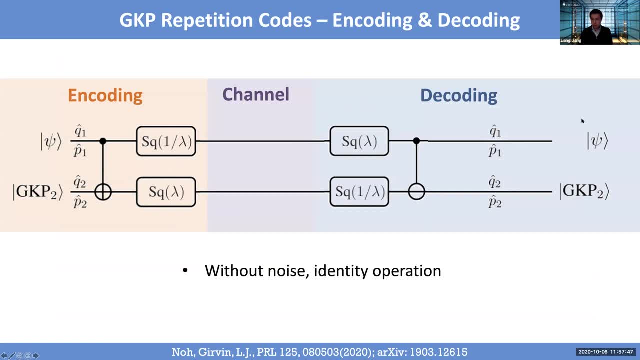 be the control difference And after that you restore the state as it should be. So this is ideally. you just do the decoding like this And in practice there will be noise. So if there's noise here, I assume the noise model which you have uncorrelated noise acting. 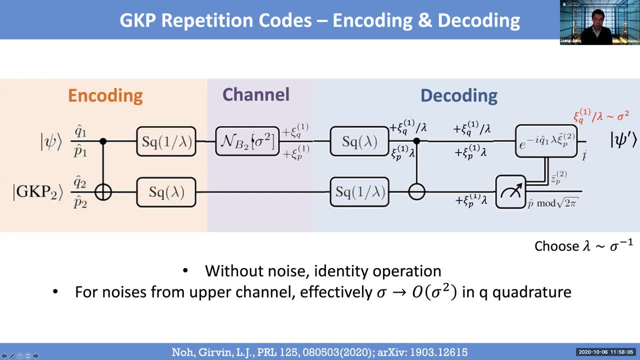 between this first mode and the second mode. So if you have noise at the first mode, then what will happen is that those noise- one component- will be passed on to the second mode. But it's okay because you actually measure this component, one component. 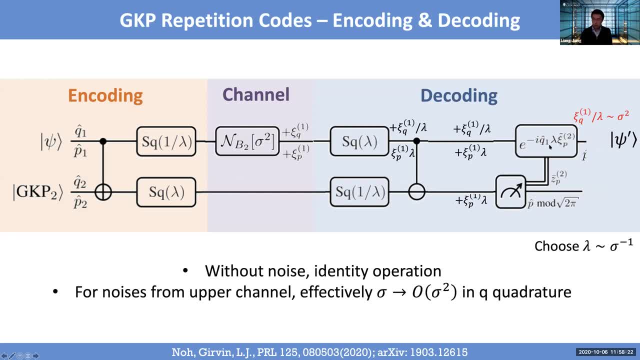 of noise in the P quadrature and you can suppress that quadrature of the noise. On the other hand, the noise on the other component will actually be squeezed and suppressed by effect of lambda. So after this procedure you'll find that both position and the momentum 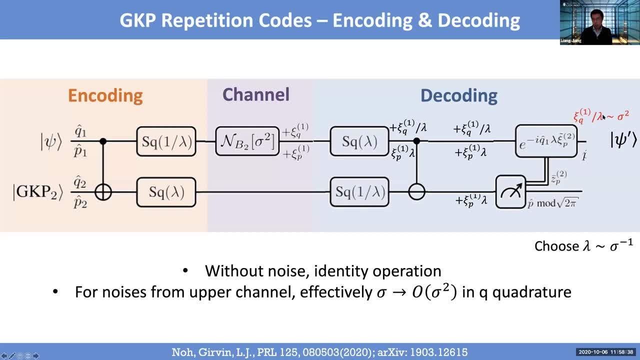 quadrature noise will be suppressed by effect of lambda, Because one quadrature noise gets suppressed by squeezing, the other quadrature noise actually gets amplified by squeezing, but with the GKP-ancilla you can measure and suppress that quadrature noise. So basically, 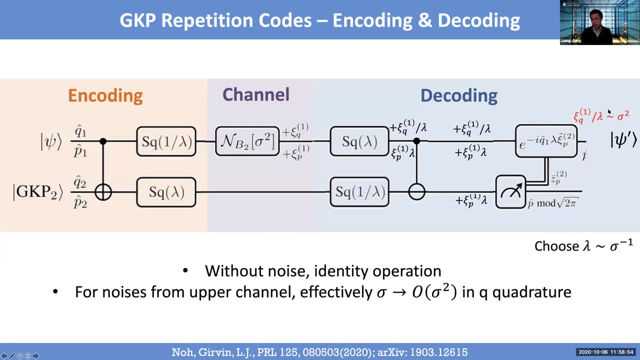 at the end you get both: quadrature noise get suppressed by effect of lambda And the lambda is chosen to be effectively limited by the finite squeezing of the initial noise. So you get the magnitude of the noise that you added to the system. So you just go noise. 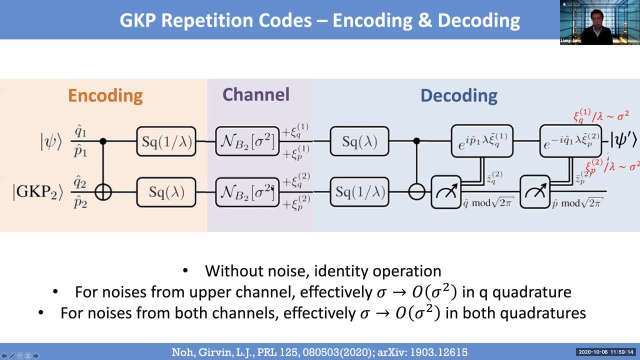 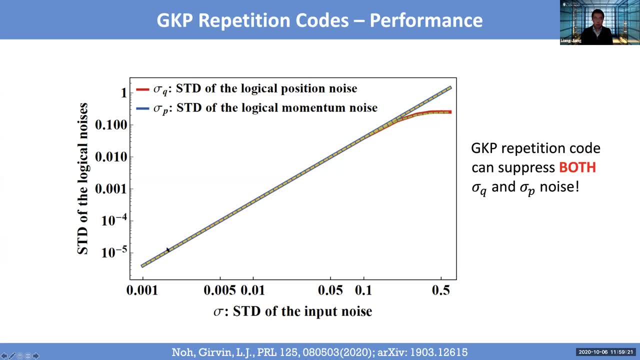 from sigma to sigma squared, And if you have noise added to this second mode, a similar procedure can also be performed to suppress both quadrature noise. So here is kind of like numerically you can verify that here- the noise that's the input noise and this is the noise after suppression. 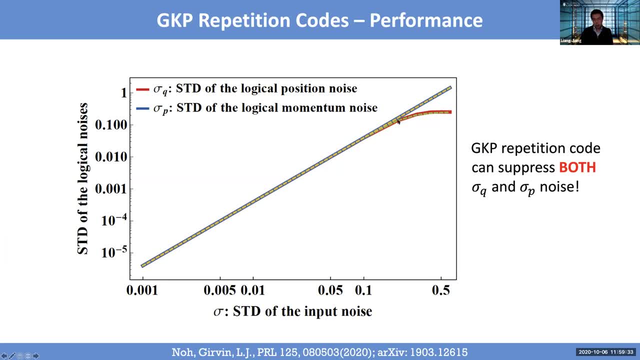 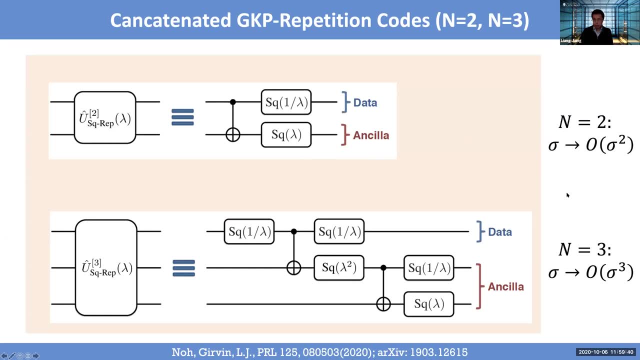 it has this quadratic scaling. when you perform this GKP-stabilized code- And this is kind of like a summary of like- you can have one ancillary mode, you can suppress noise to its second order If you have two additional. if you have two ancillary modes, you can suppress noise to 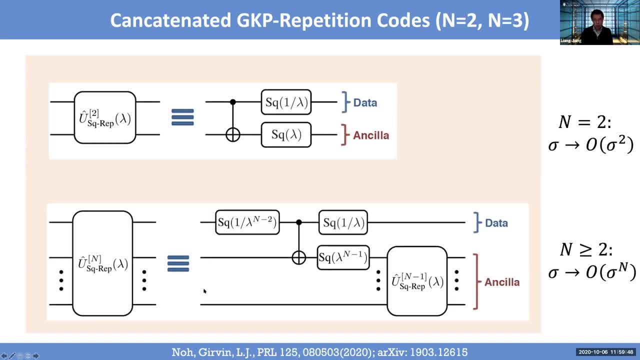 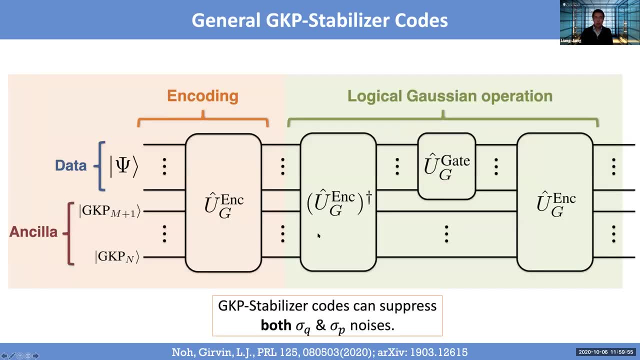 its cubic order And if you have n minus one ancillary mode, you can suppress noise to the nth order. So basically there is a systematic way of designing the codes which we call kind of the GKP stabilizer codes, because there is sort of a one-to-one mapping between the current 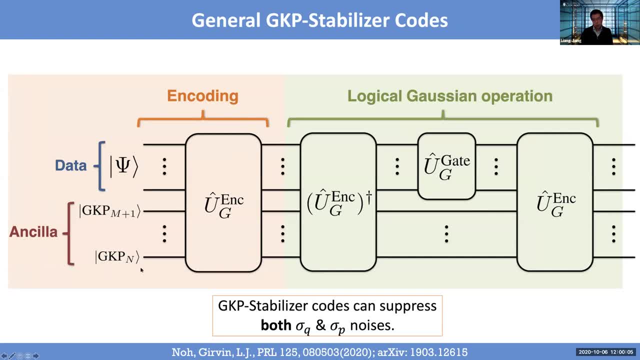 coding using kind of a non-Gaussian resource of GKP state and the Gaussian unitaries of being splitter and squeezing, And that allows us to achieve the bosonic code that can suppress both position and momentum, quadrature, noise And what's more important is actually in the logical space we actually still preserve. 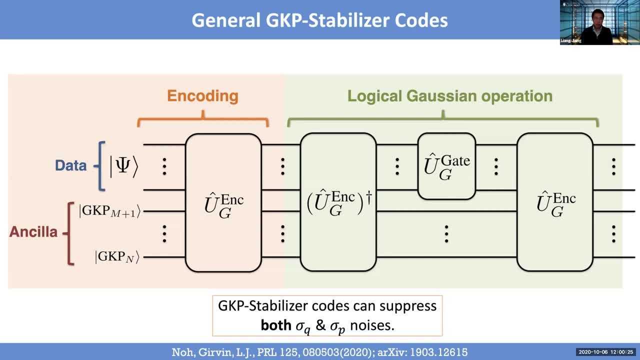 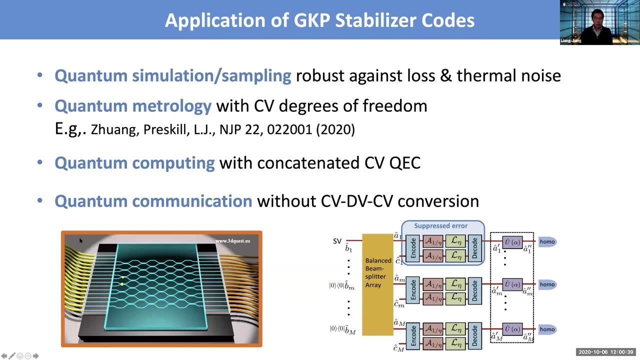 the bosonic nature of the system. So it is indeed a bosonic code for logical bosonic modes, while correcting photon loss error. So you can imagine that maybe these codes could be useful for like the boson sampling at the logical level, or maybe you can use it if you want to simulate the botanic systems. 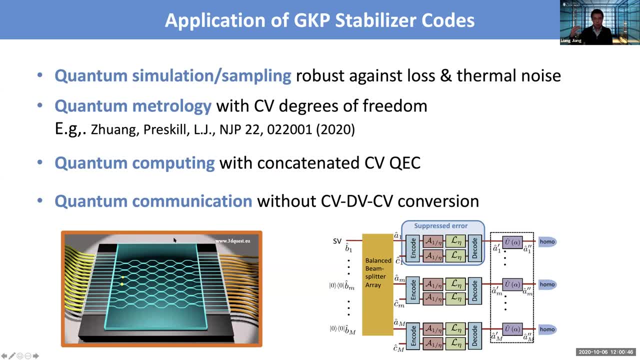 And then these codes could give you a logical level of bosonic encoding while correcting photon loss error, And it can also be used for distributed sensing if you want to preserve some of the bosonic nature before you're performing the sensing tasks. So I think that these are kind of like different applications one might consider. 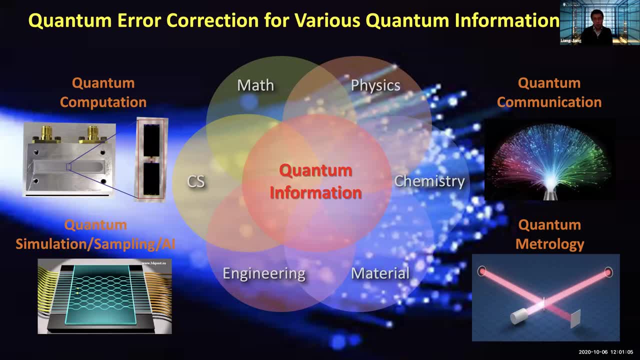 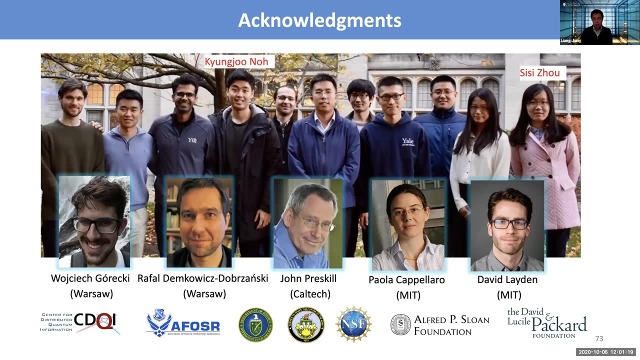 And just maybe as a summary, that basically, like the key message on the conveyor, is that the quantum error question could be useful for various applications Besides computing communication. it could also be useful for metrology, as well as quantum simulations, if needed. And finally, I would like to thank the people who actually work on these tasks besides collaborators. 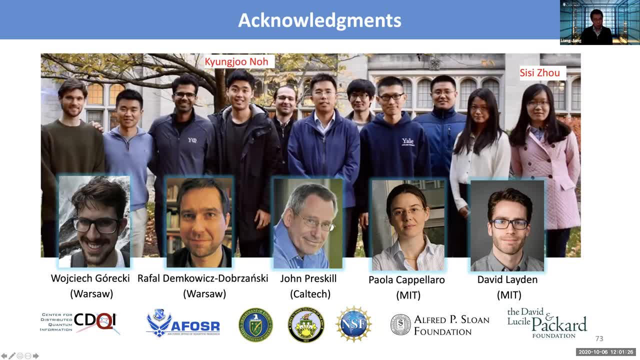 And I would like to highlight the two students like Sisu Zhou, who did a lot of work on this bosonic well, the error question with sensing For sensing, And Kendri Ngo, who also did this bosonic quantum error question while preserving bosonic. 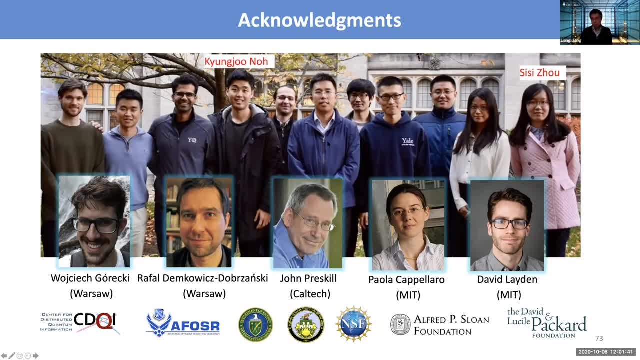 nature And, yeah, thank you for your time. Thanks a lot, Liang, for an excellent talk. That was great. So do we have any more questions from people in addition to the ones that we had? So I guess I have a. 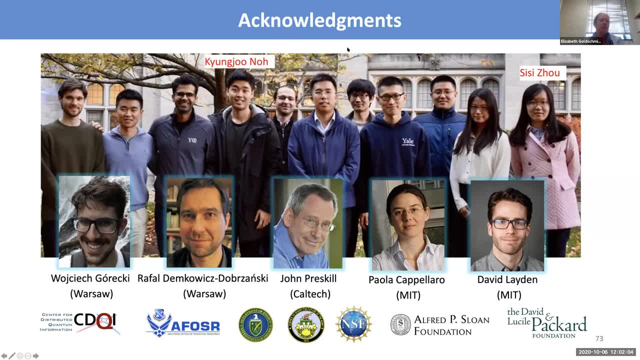 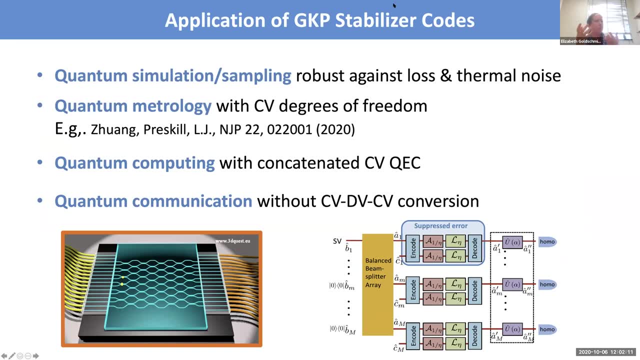 Maybe a very general question. The result that you had- that you couldn't do quantum error correction if the noise was within the Or if the sensing Hamiltonian was within the subspace of the noise. that feels like a kind of a basic statement of sensing is about sensing your environment. 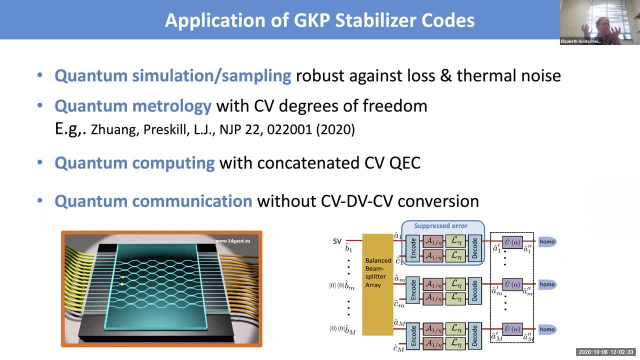 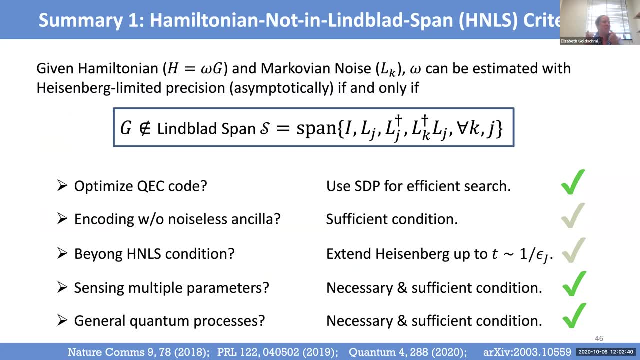 And if the noise is in the same environment, quantum error correction is for being insensitive to your environment And so you kind of maybe obviously can't quantum error correct the same thing that you can sense. Is that a reasonable interpretation of that result? Yes, 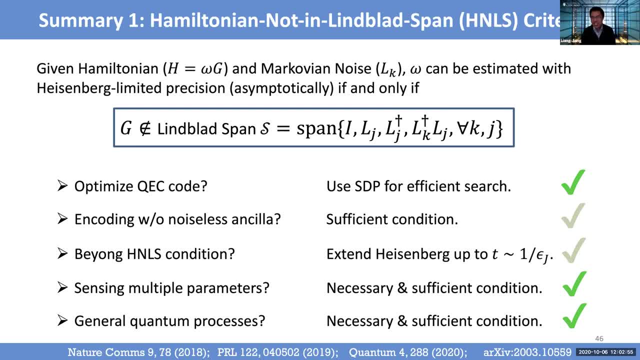 Yes, In some sense, like once you understand the theorem, it's obvious, right? It's like you cannot distinguish a Hamiltonian from your noise. Yeah, Especially if the Hamiltonian isif it's a noise, If it's the same as the Markovian noise operator, like a sigma z, sigma z, then basically there. 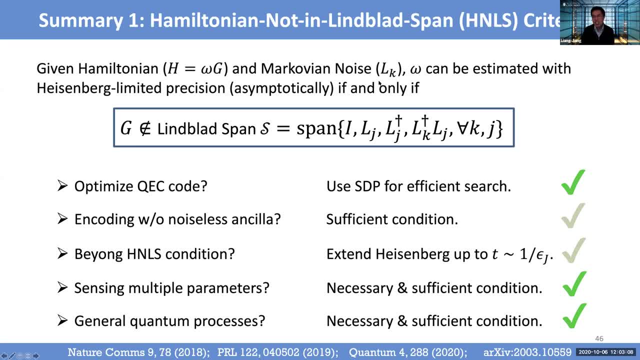 is no way you can differentiate whether it's signal or noise. Yeah, And that could be a little bit non-trivial. if you have photon loss and then you have a frequency shift, then actually the quadratic part of this Limbladian could also be contaminated. 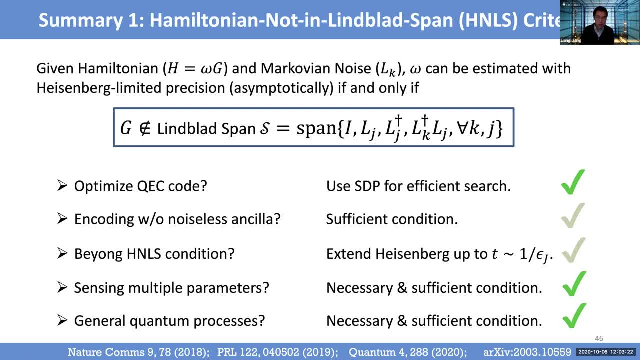 And that's the part which is a little bit less obvious. But on the other hand you can think that if you consider the back action from the Limbladian noise, There is a term in your Hamiltonian which looks like a kind of the k dagger, k right. 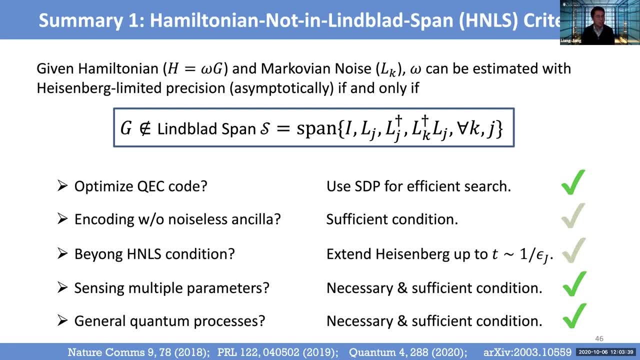 And those actually will cause a decrease. It's a non-Hermitian evolution, due to those parts which you cannot distinguish, whether it's a Hamiltonian evolution or whether it's a decoherence due to the Limbladian noise. Yeah, Okay. 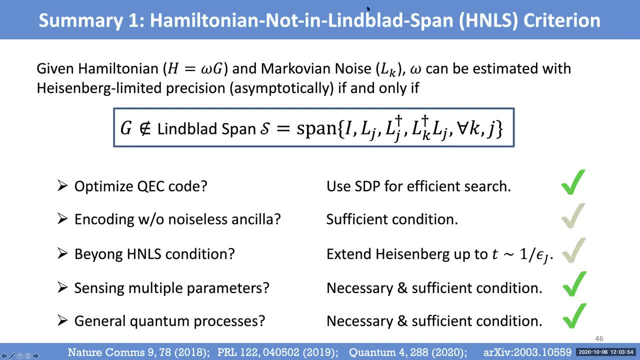 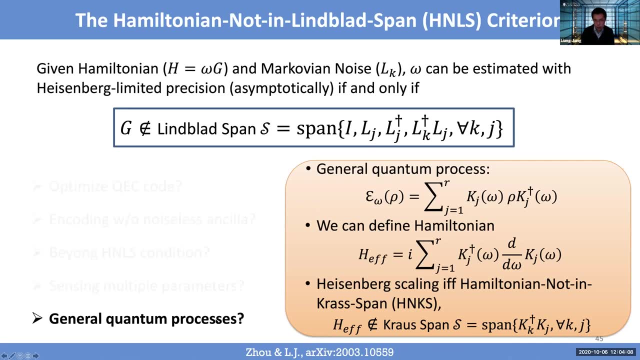 Thanks. Can I ask a question just following that one? So is there a similar theorem where you would replace the Limbladian by Fixed the Krauss operators? Yes, yes, And I think that's probably related to this statement. that's actually recently actually. 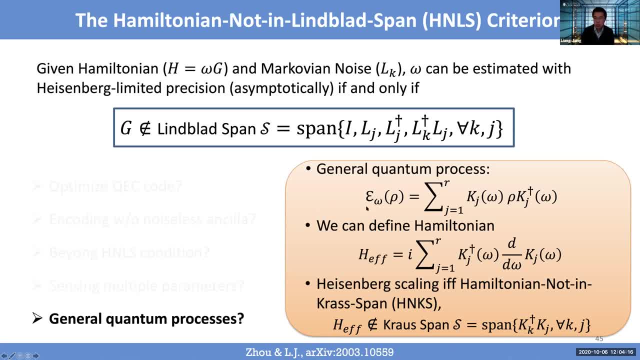 also worked out this general processes which you can consider. instead of Limblad mass equation evolution, we can consider general CPTP map which is characterized by these Krauss operators which depend on the parameter you want to sense And in this case, 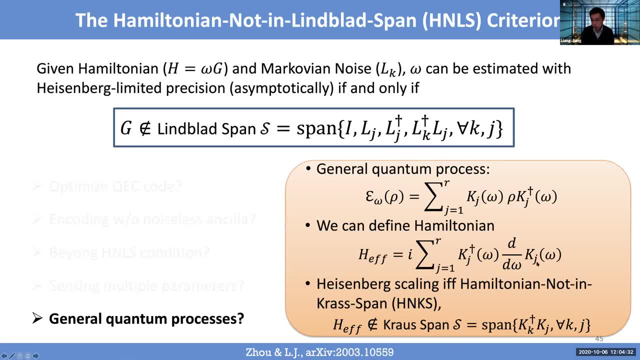 In this case, you can actually define an effective Hamiltonian which is associated with the derivative of Limblad and multiply its conjugate. Then you can show this is a Hermitian operator And for this operator, if you want to sense, 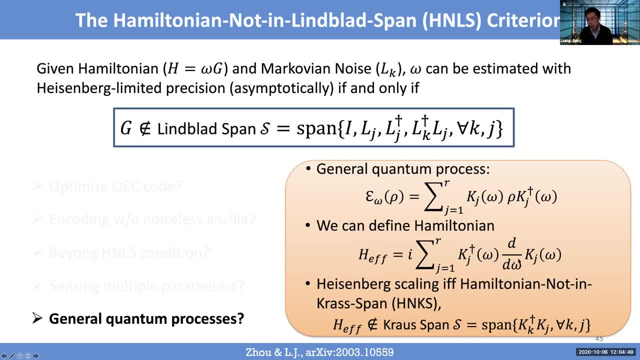 So if this operator, which is kind of you can think of it as in the- It's an effective Hamiltonian associated with the omega, Okay, If that operator is in the Krauss span, then you would. Okay, If that operator is in the Krauss span, then you will not be able to restore Heisenberg. 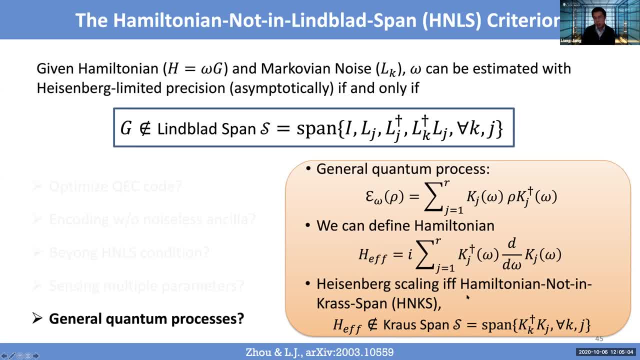 scaling. but if it's not, then you will be able to design a code to restore Heisenberg scaling. Yeah, Okay, I mean, of course, if there's no derivation in omega, then this might have to be tweaked a little bit. 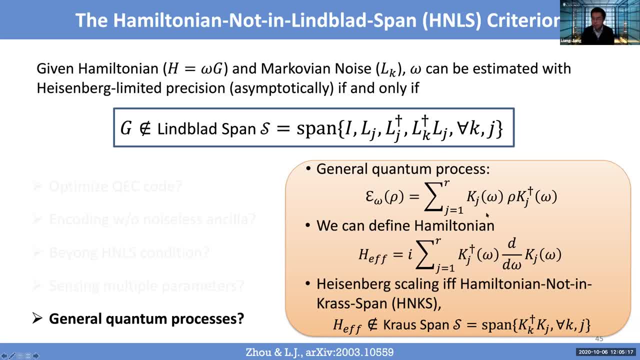 Right, Yeah, Yes, If everything is right, then you have to maybe change that a little bit, And yes, And then that actually comes to my second question. So so all this analysis is essentially for a sufficiently small time. Yeah, 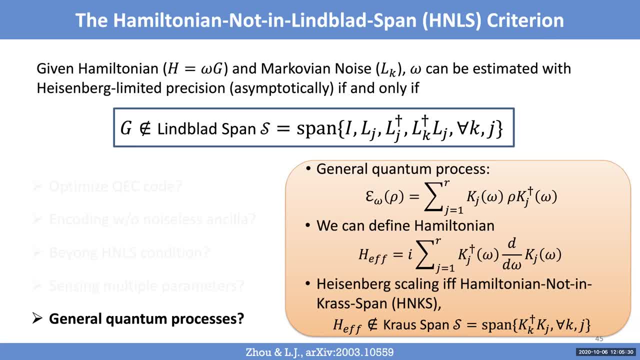 Yeah, That's the key, right. Well, actually, for this general quantum process, it can be a finite evolution, It should work as well. But usually what happened is that if you have Linn-Bladian dynamics, if you let it evolve, 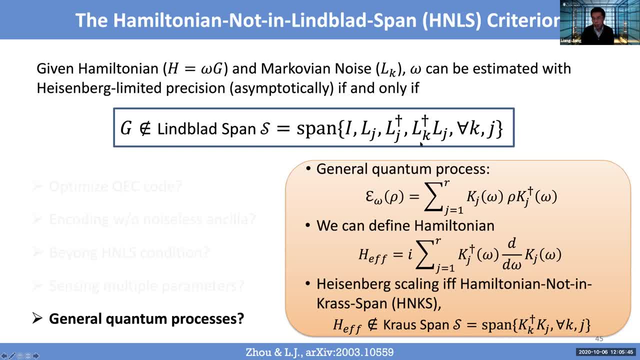 for finite time. actually, the Krauss operators would have higher orders of the Linn-Bladians. Well, that, And that's part of the reason why, if we start with the Linn-Blad master equation, we might need a dt to be infinite tesmos form. 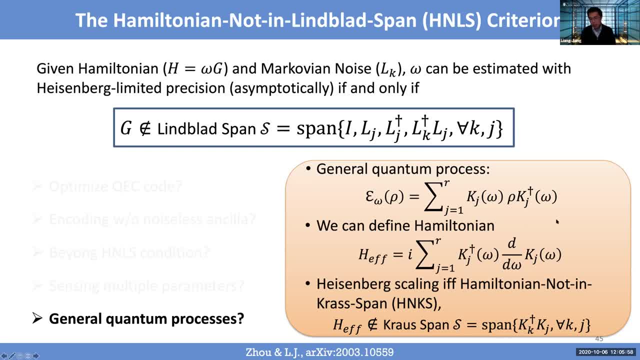 Okay, Yeah, if there's a general quantum process, somebody give you a black box, say this is a process characterized by these cross operators, then then you might be able to, then you can just use this criteria. yeah, yeah, very interesting. thanks, i think paul has a question. yeah, i do. 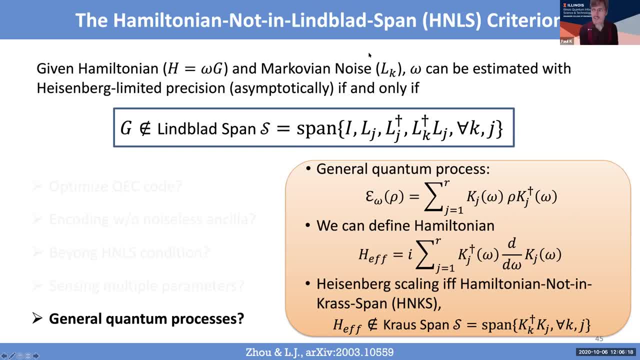 hi lan. so your notion of, uh, modular measurements, you know, yeah, this inspector 2 pi just reminds me a little bit. yakira harnoff always used to talk about modular momentum as a somehow a way of resolving lots of paradoxes or causing them. i don't know he was in his mind. those are kind of. 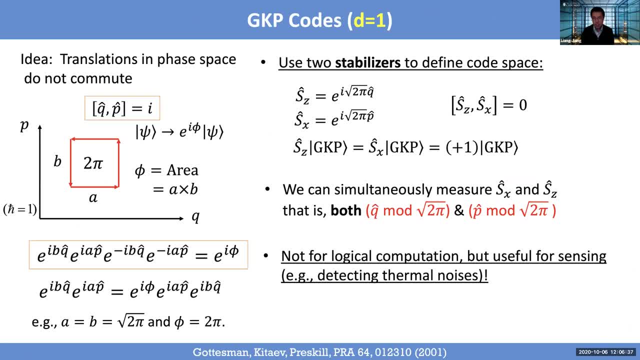 the same, the same thing, i guess i'm just wondering is this: is this the same concept that he's that he was talking about? again, i haven't looked at that his stuff in in many years at this stage, but yeah, yes, i think it's, it's related and uh, uh, so so i think that, uh, here i just listed one reference by: 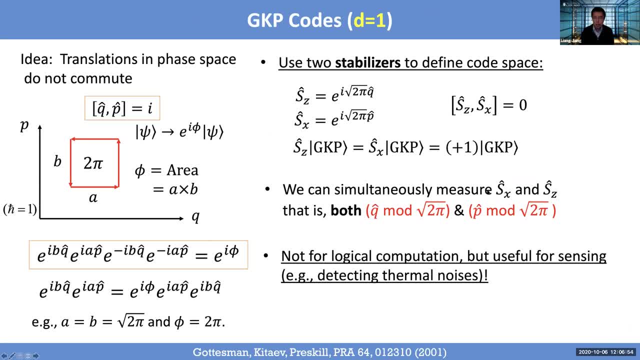 gkp, which is the original paper that proposed the gkp code, and there are also, like more recent papers by barbara tahar and others, which actually like a show that we can develop a scheme to measure these quantities, and also recent experiments by michelle de vera's group. they're actually using a transma to kind of like. 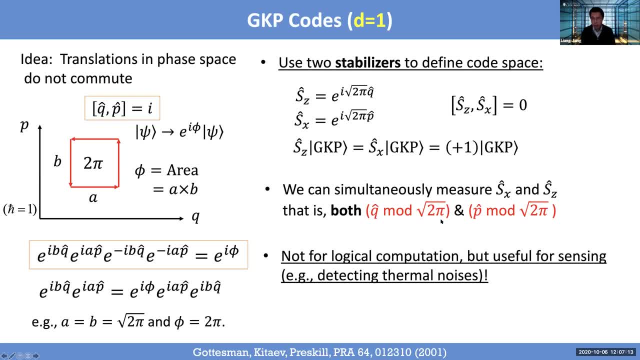 to perform a weak measurement of these positional momentum module, root 2 pi or root 4 pi, and you can actually, by just projecting those things, a weekly measurement and adjust it following that so you can actually stabilize the system to a gkp logical space, so that actually prepare a logical state by 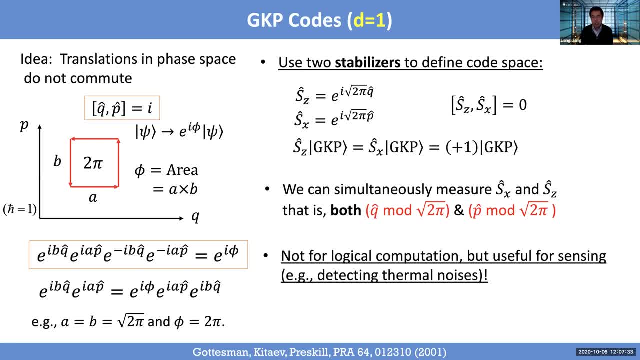 this measurement and the feedback interesting so. so it's actually a pretty powerful way of kind of prepared state. but you just keep measuring stable like this and then you actually prepare the state. yeah, cool, thank you. yeah, you're welcome, right, well, thanks a lot, liang um, for an excellent talk again. 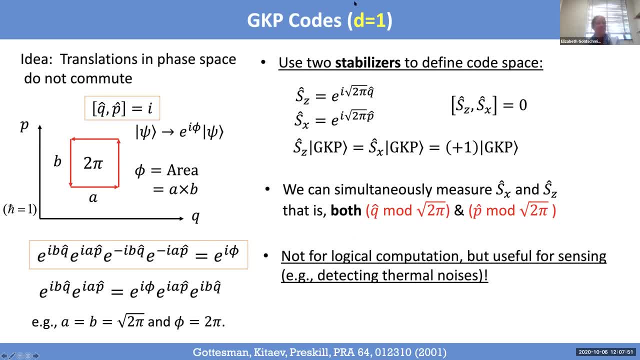 um, and it seems like i think we're done with questions. so, um, thank you, and yeah, you've got some media.